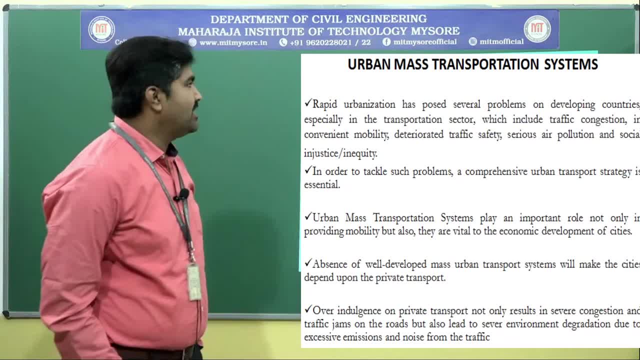 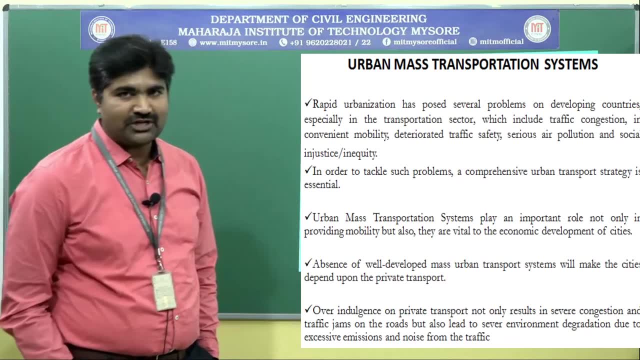 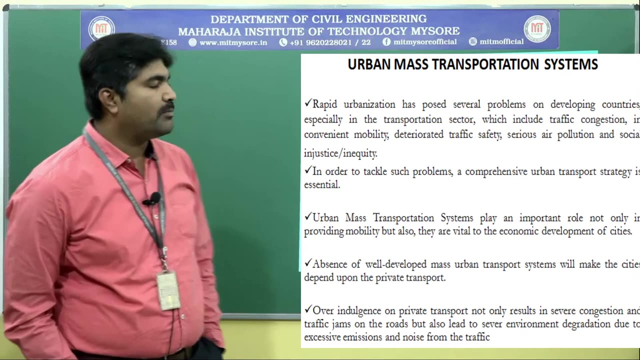 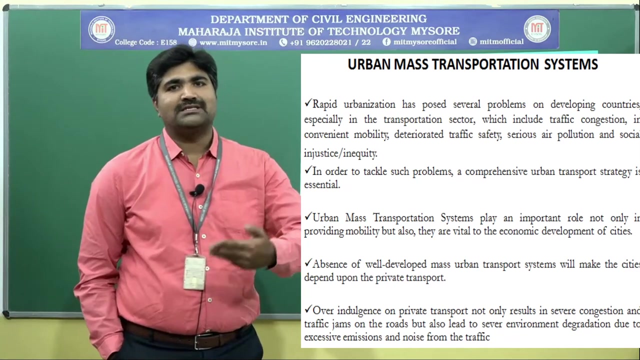 Especially in the transportation sector. The problems are the traffic congestion, inconvenient mobility, deteriorated traffic safety, serious air pollution and social injustice or inequity. In order to tackle such problems, a comprehensive urban strategy is essential. Today, as we know, due to rapid urbanization, we are facing with several problems. 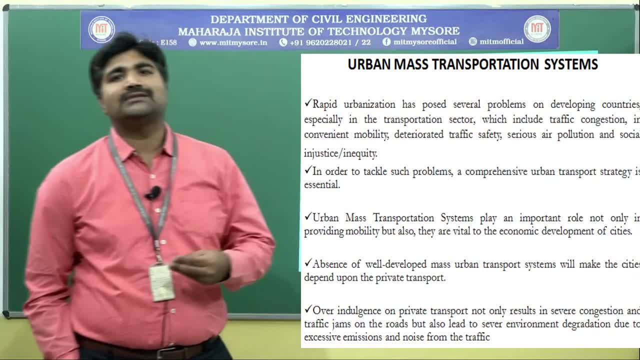 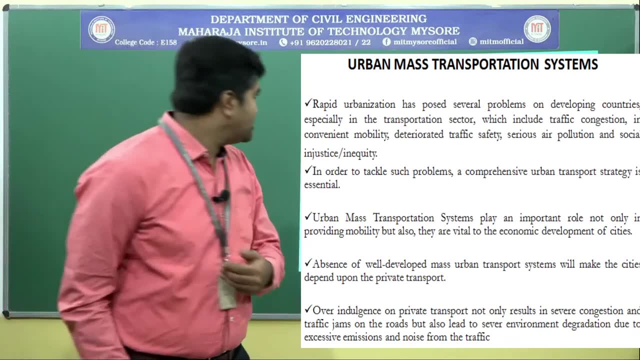 See the several problems. are the traffic congestion due to increasing population? Okay, This results in the increase of vehicle, private vehicle. This causes the congestion And also there is inconvenient to mobility Means, there is inconvenient for the movement, Okay. 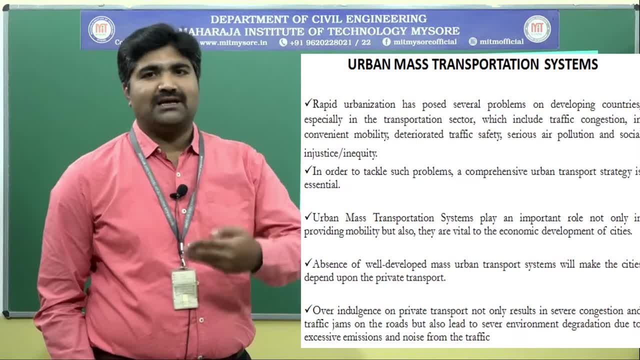 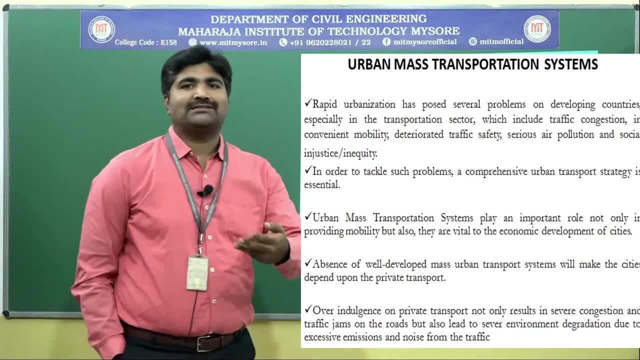 There is difficulty for the movement- Okay. Level of service is sorry. level of service is decreasing day by day. Deteriorated traffic safety due to more number of vehicles, There are more number of accidents. The peoples are feeling less safety on streets. 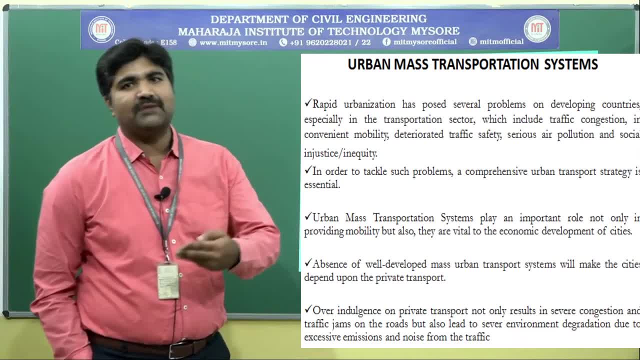 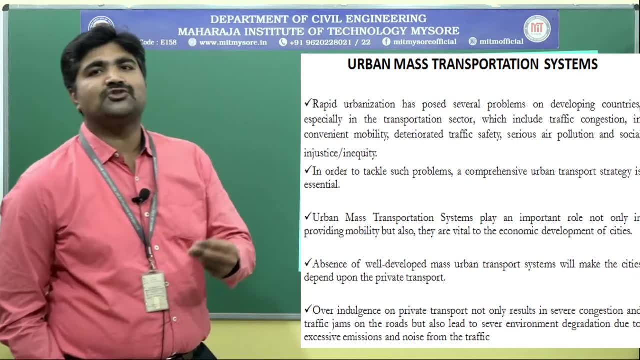 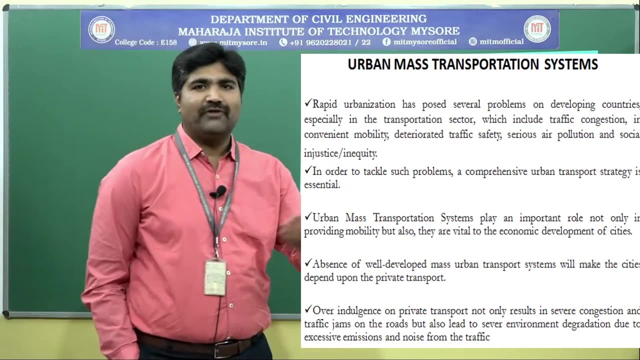 And serious air pollution. Okay, Due to more number of vehicles, The emission is increasing day by day. Okay, This is leading to pollution And also social injustice or inequity. Today we are facing social injustice. See the person who are having Porsche car and Porsche bikes, high-end bikes. okay, this SUV, these vehicles which are fast, okay, they are not leaving space to slow moving vehicles. 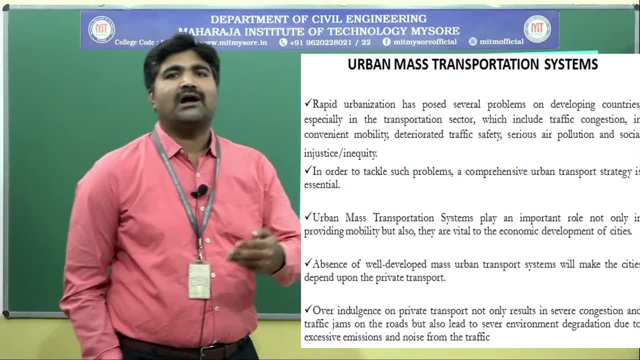 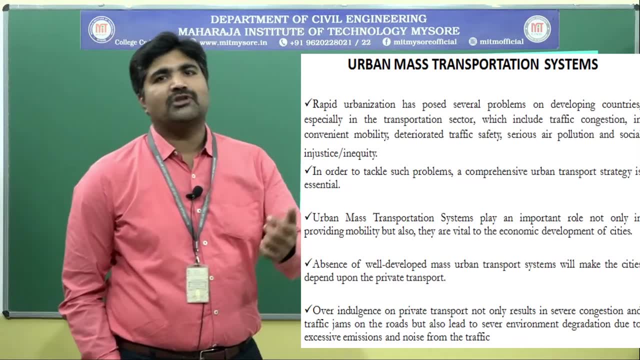 That may be cycle or pedestrians- okay, They are not leaving space to travel for slow moving vehicles. The slow moving vehicles may be bullock carts or cycle vehicles. Okay, The slow moving vehicles may be bullock carts or cycle vehicles. Next, to tackle such problems, we need a comprehensive urban strategy. 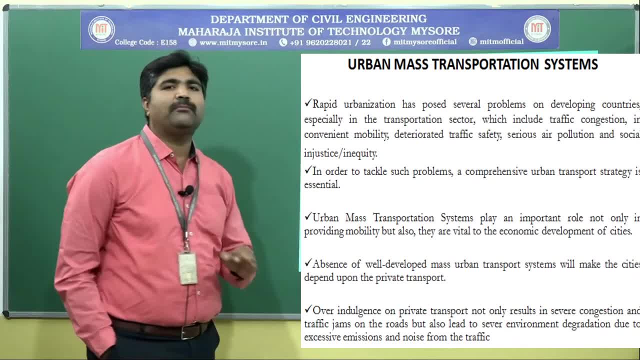 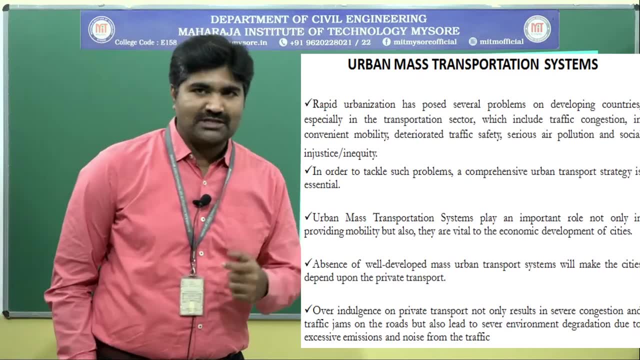 That is essential. Okay, See, urban transportation play a very important role, not only in providing mobility, Also, that is very important for the economic development in the cities and towns. They are very important for the economic development for any region. Okay. 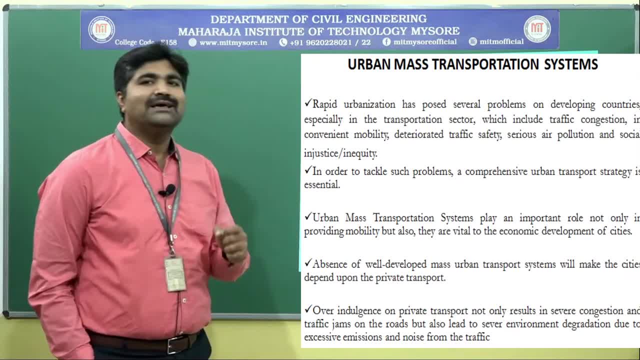 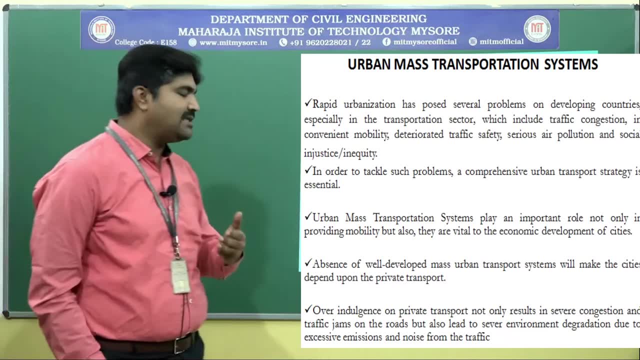 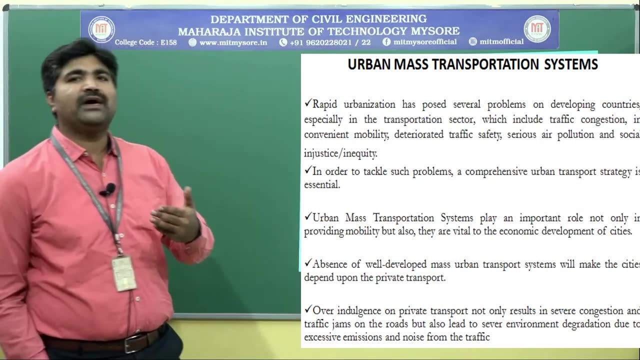 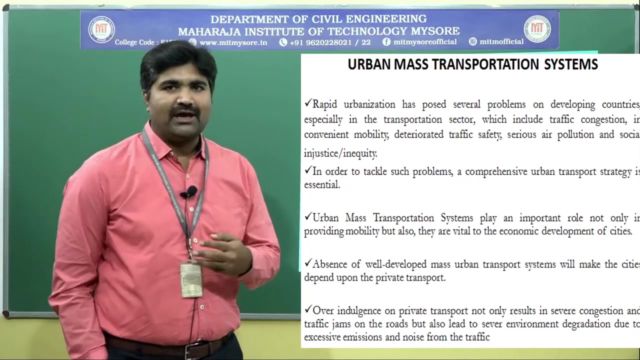 See absence of well-developed mass transportation will make the cities to depend upon the private vehicles. means private transport. See the war. Indulgence means the war. dependence on the private transport not only results in the severe congestion and jams- okay- on the roads, but also lead to severe environment degradation. okay, due to excessive emission and noise generated from the traffic. okay. 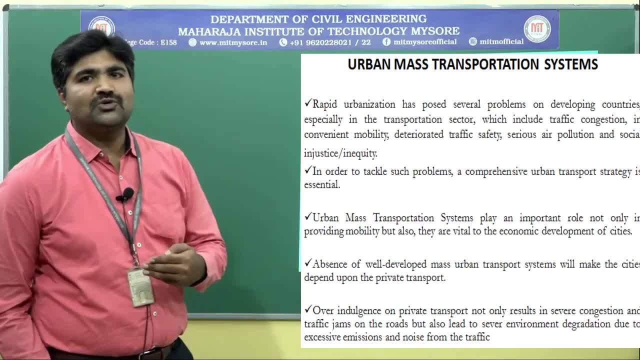 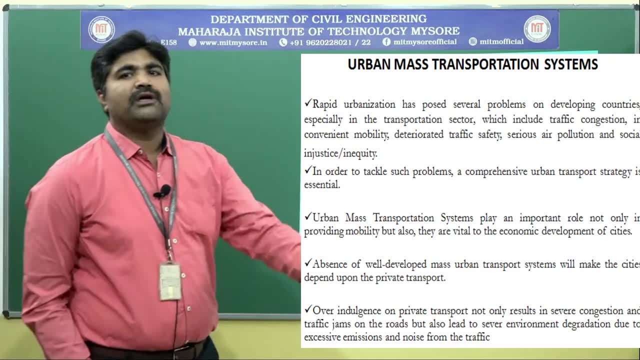 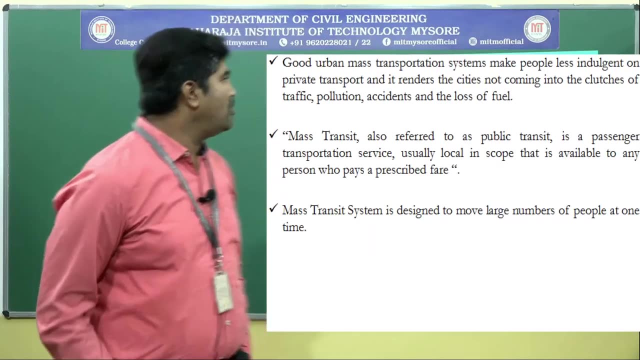 Overindulgence, war, dependence on the private vehicle leads to congestion and jams and also leads to emission. results in the severe pollution. okay, due to emission and also noise will be generated which cause the noise. See the good urban mass transportation system. make people less indulgent means less depend on the private vehicles. 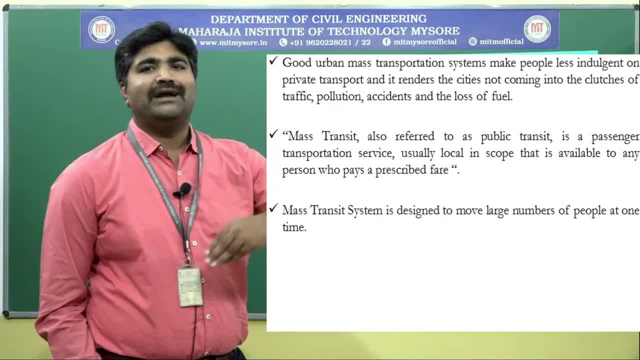 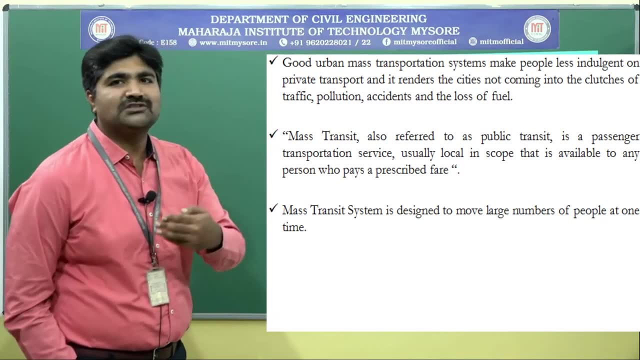 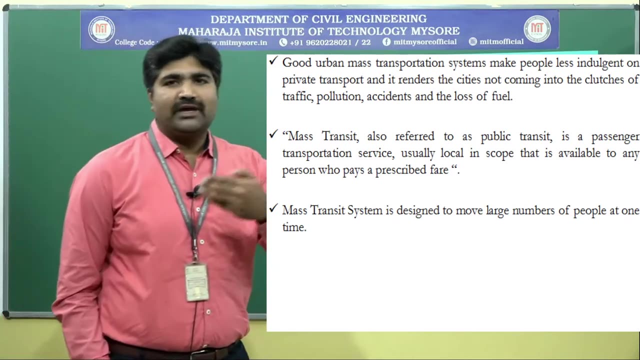 As we provide good, efficient mass transportation. we can indulge means we can reduce the dependency on the private transport. okay, It renders the cities not coming into clutches of traffic and pollution, accidents and loss of fuel. okay, We can avoid the. we can decrease the pollution okay. 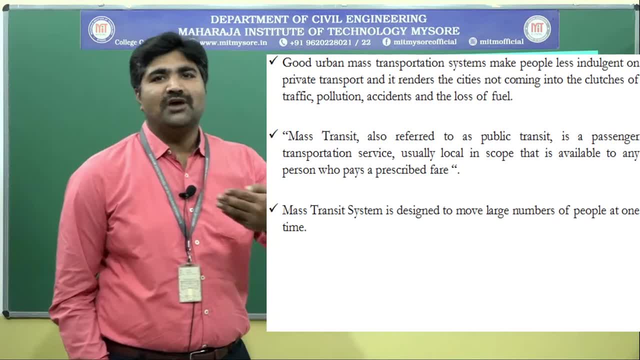 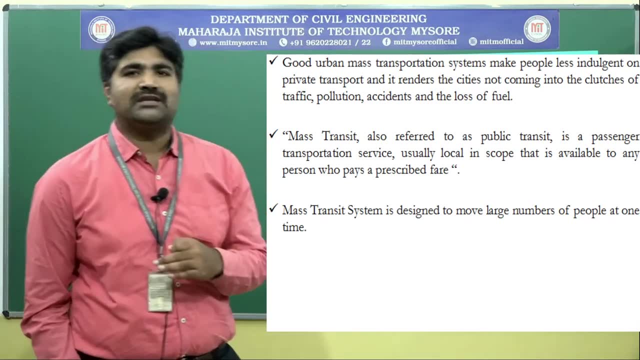 And we can reduce the pollution. And we can reduce the pollution And we can reduce the accidents, We can decrease the usage of the fuel. okay, These are the some of the advantages by providing the mass transportation. okay, What do you mean by mass transportation? 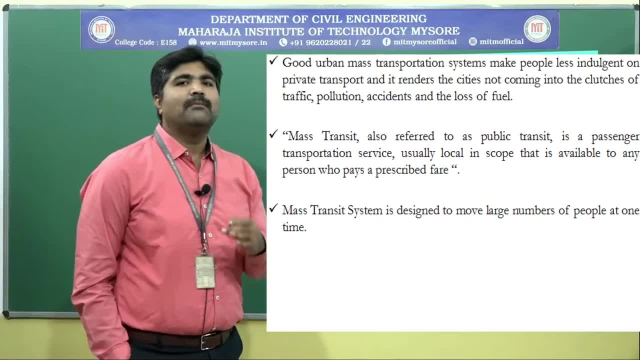 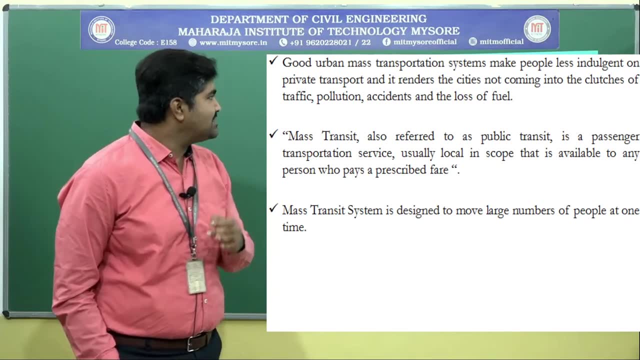 Mass transit. okay, Mass transit also refers to as public transit. Public transit means public transportation which carries a passenger. okay, It's a passenger transportation service, usually in local in scope. okay, It will be, it will have scope in the local. 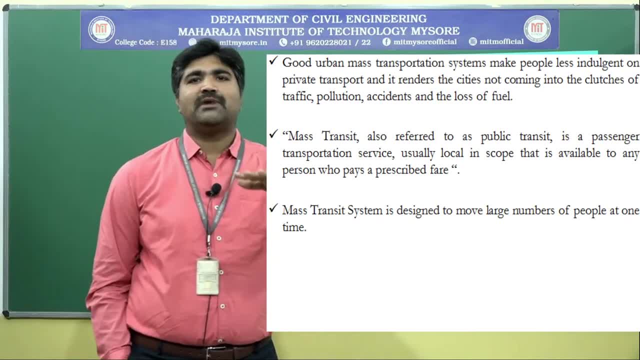 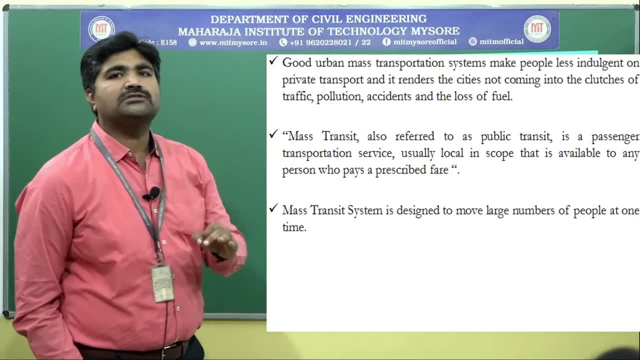 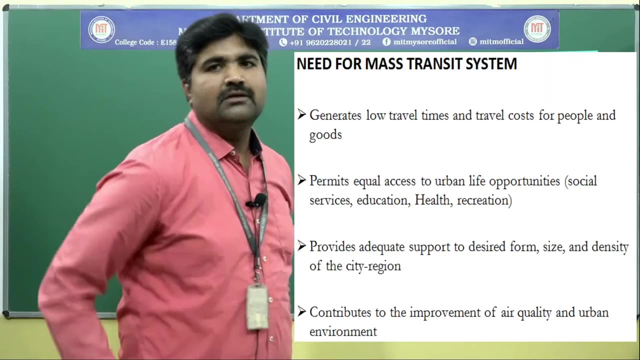 If you take Mysore or Bangalore, we have a Metro, BMTC, Mysore city buses. okay, Locally they have a scope. okay, This mass transit system is designed to move large number of people, large number of passengers at a time. okay, okay. 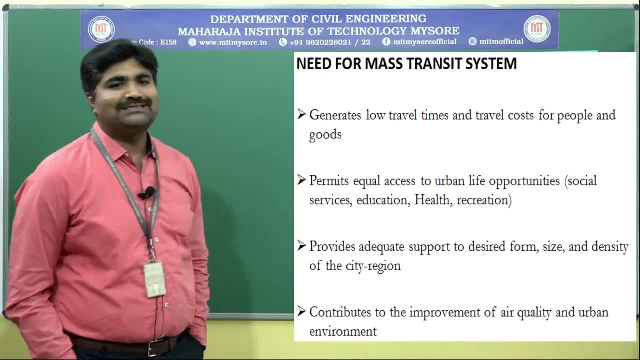 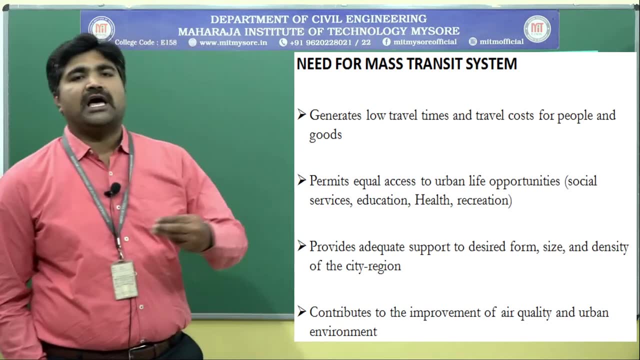 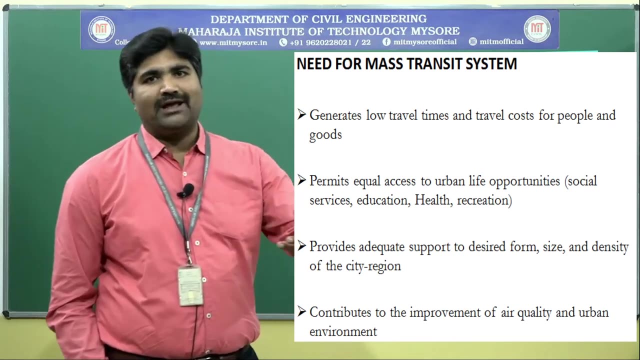 Why we need this mass transportation. Why we need mass transit system: okay, This generates low travel time and travel cost for people and goods. okay, As we know, as we travel in metro or monorail, it takes less time. Okay, in Bangalore, if you take, if you travel with your own vehicle or travel by bus- to travel a 5-kilometer distance, it takes more time. 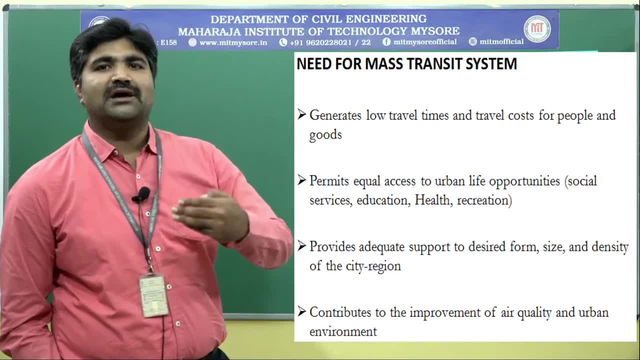 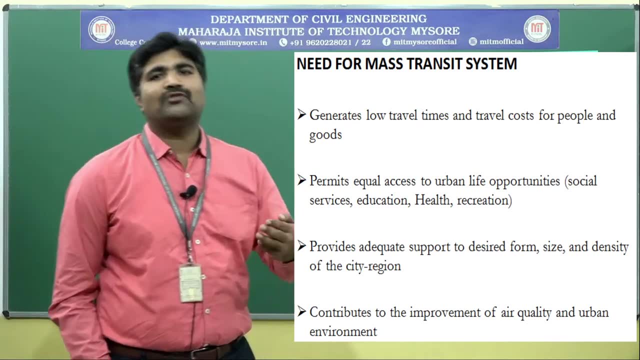 If we prepare the mass transportation, mass transit, that is, metro or monorail or suburban rail, it takes less time and also the cost will be less. okay, both for the people and the goods. okay. Next is permits, the equal access to urban life. 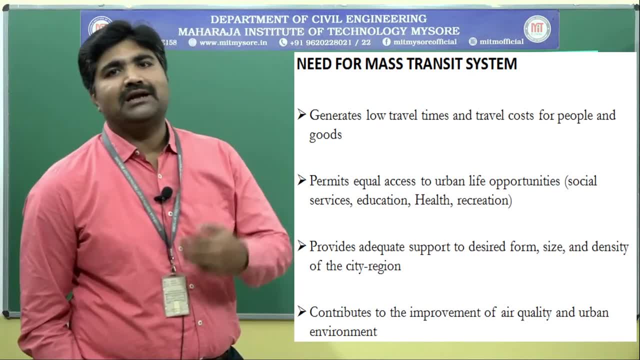 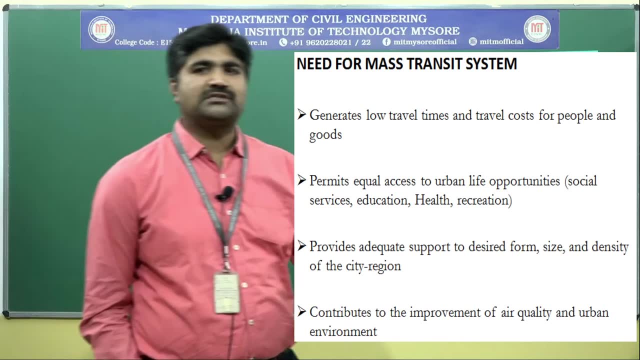 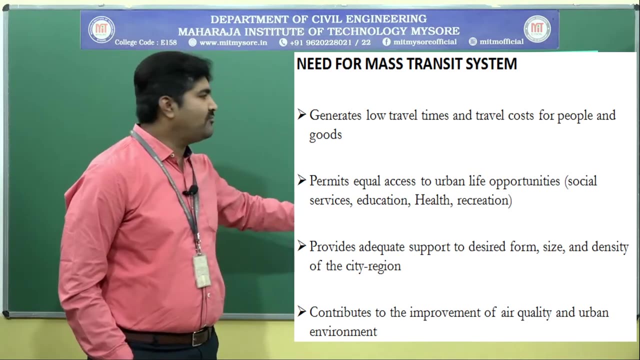 It permits equal access to hall in urban, That trips may be for social service, It may be for services or for hospitalization, or for education purpose trips, or for working purpose trips or for recreation purpose trips, Okay. and also it provides adequate support to desired form, size and density of the city or region. 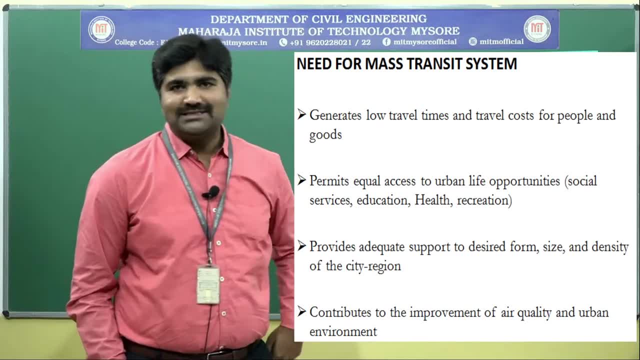 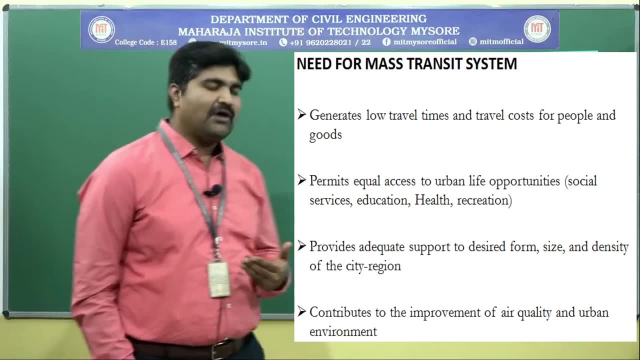 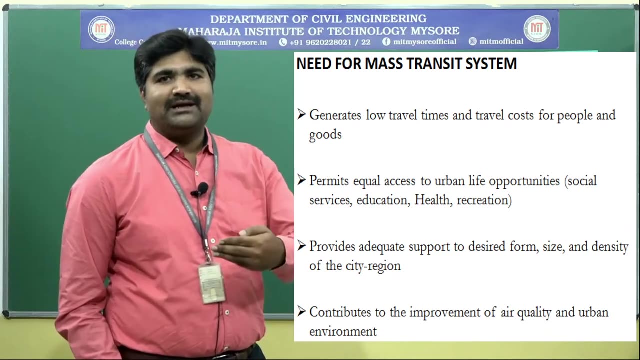 Whatever the density of the city, it gives adequate support to the city or region. okay. And next, it contributes to the improvement of air quality and urban environment. okay, As we provide efficient mass transportation. Okay, We can relieve the congestion which is automatically decreases the usage of personalized vehicle, okay. 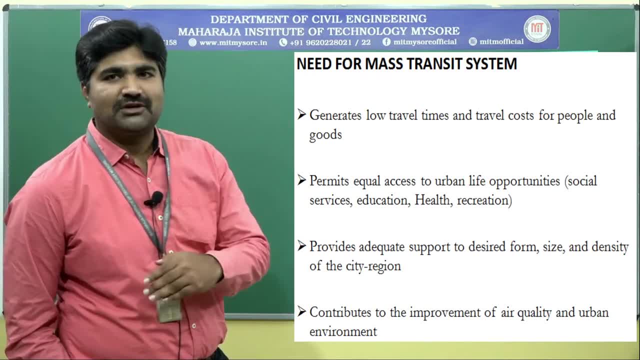 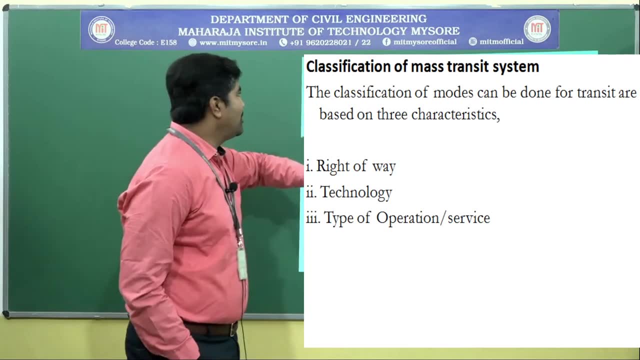 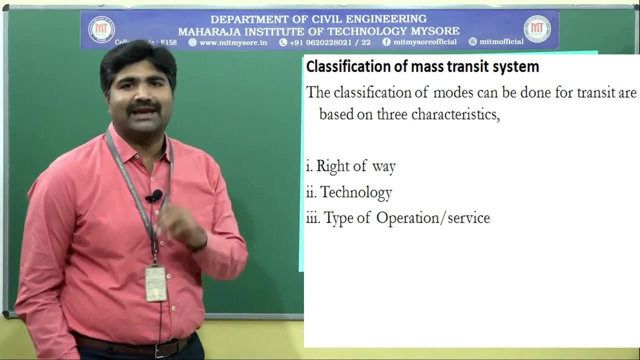 This in turn reduces the emission, which saves the pollution. okay. Next, classification of mass transit system: okay, The classification of modes can be done for transit or based on the three characteristics: okay, Based on three characteristics. they are right-of-way technology, type of operation or type of transportation. 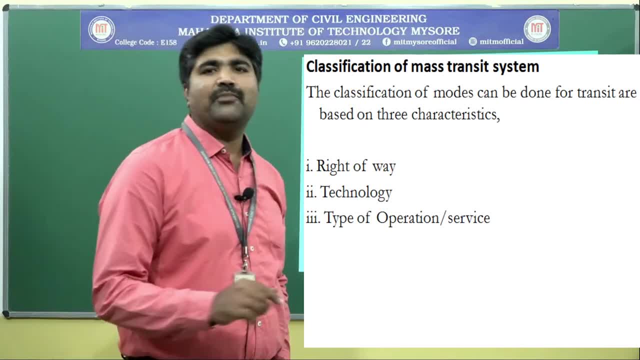 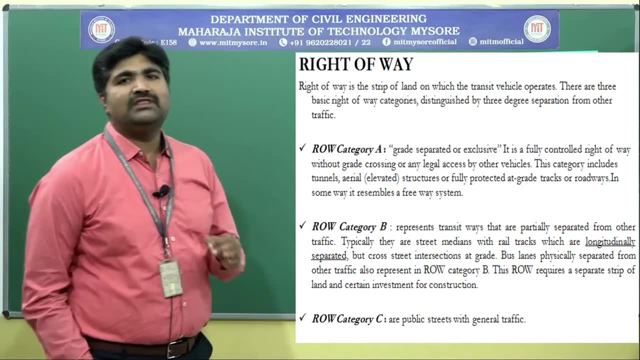 Okay. Type of service: okay. First, based on the type of right-of-way: okay, Right-of-way, what do you mean by right-of-way? See, right-of-way is the strip of land within which all the transportation facilities will be provided. 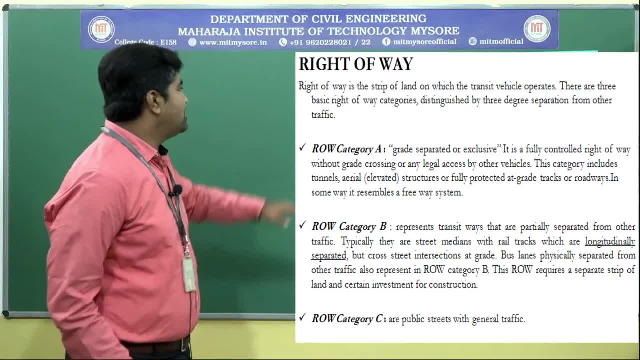 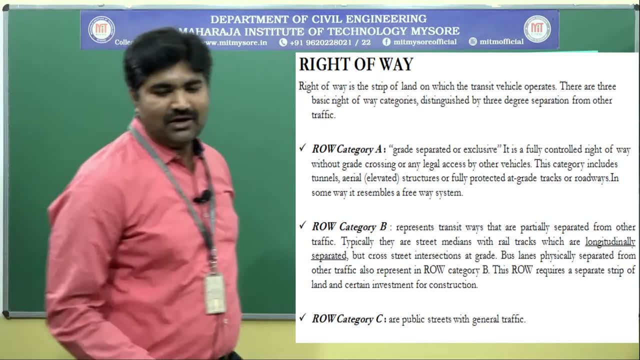 Where within which the vehicle will be operated. okay, See, there are three categories in the right-of-way: Right-of-way category A, Right-of-way category B And right-of-way category C. okay, See, in the figure you can observe. okay. 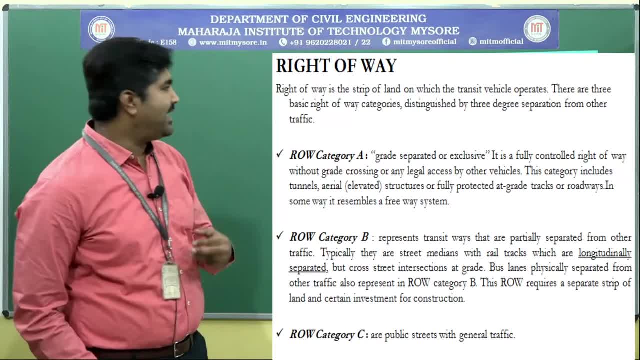 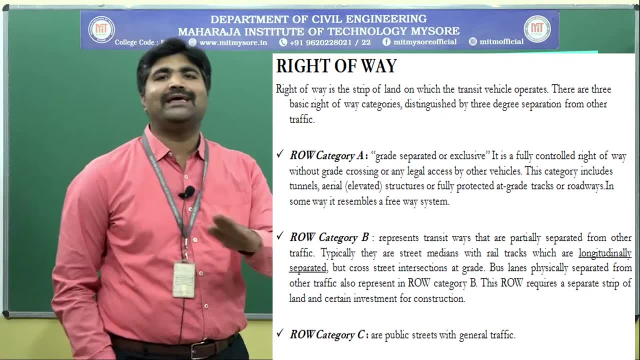 Right-of-way category A. In this category it is a grade separator or exclusive way. See. it is a fully controlled right of way. There is no access for any other vehicles. There is no any legal access for any persons or vehicles. 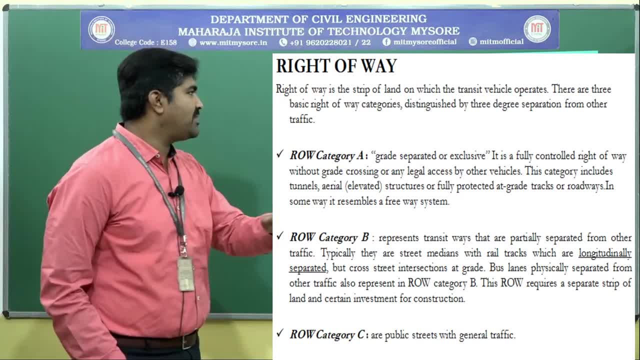 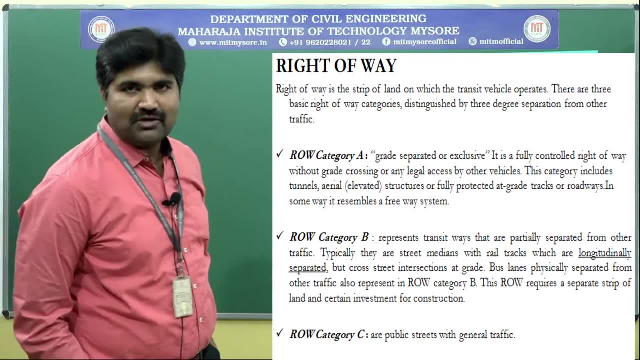 So there will be faster movement. So there will be no stoppages of the vehicles. It is a freeway system So there will be faster movement of the vehicles Separate way. there will be no access for any persons or any vehicle. 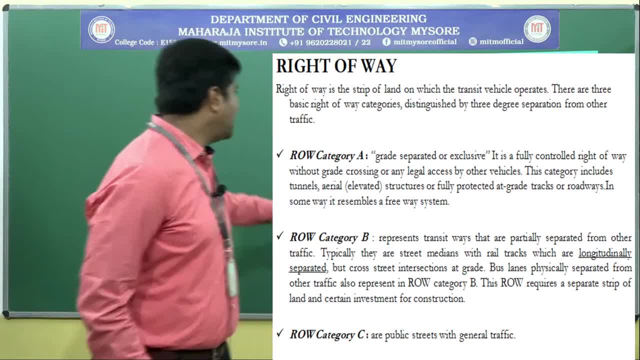 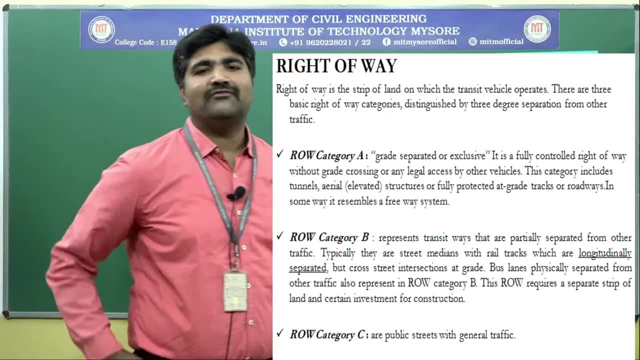 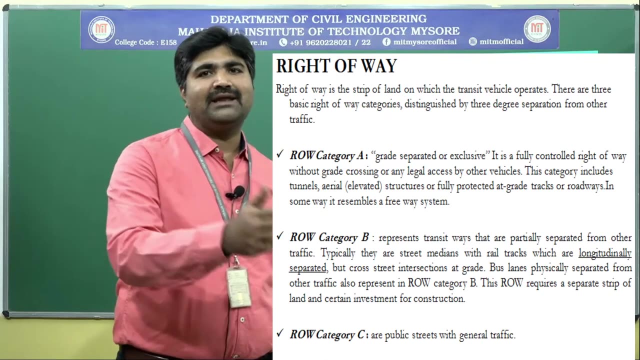 There is no legal access for any other vehicles. Next, right of way: category B: In this category the tracks are separated longitudinally From the general traffic. this mass transit will be separated. They are separated either by providing the curbs or barriers, or medians or grade separation. 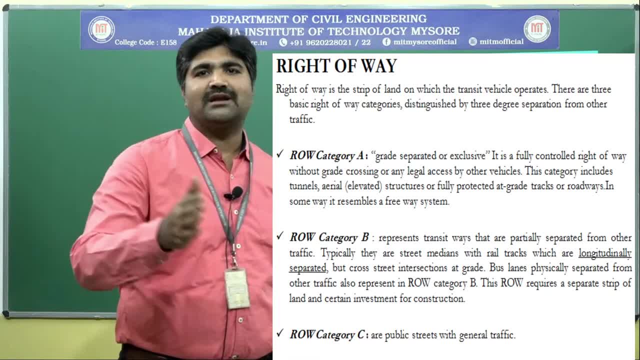 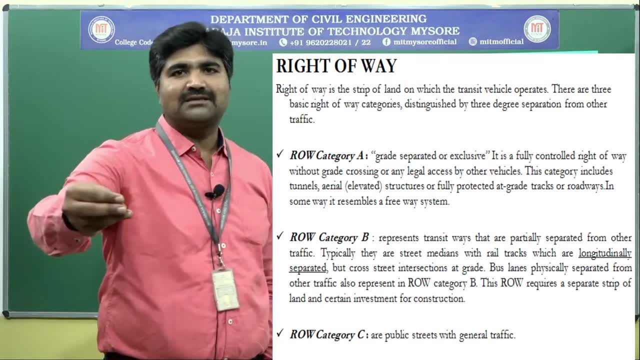 This mass transit will be separated from the general traffic. General traffic means mixed traffic. We know that. all the vehicles are there: Slow moving vehicles, from bullock cart to cycle car, bus Tracks, everything will be there. From this, the mass transit will be separated. 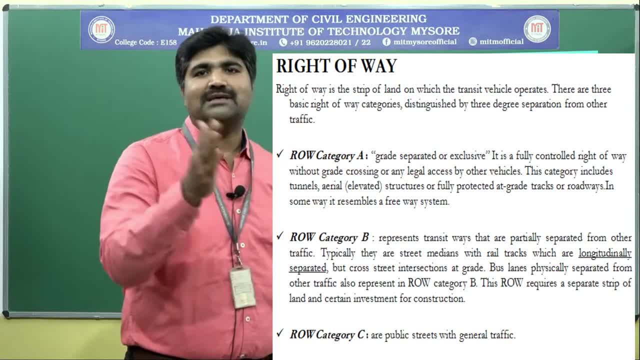 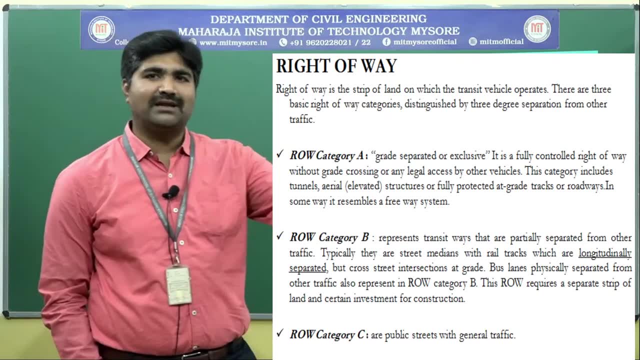 Mass transit means that may be tram, satwa buses. Separate tracks will be provided for the movement of the buses. Separate bus track will be provided. This has been provided recently in our Karnataka also, That is, in Ublidharwada. 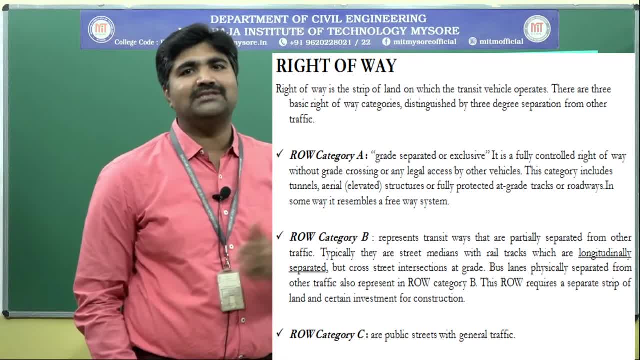 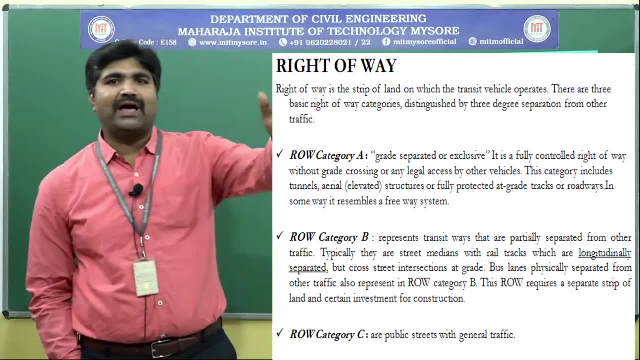 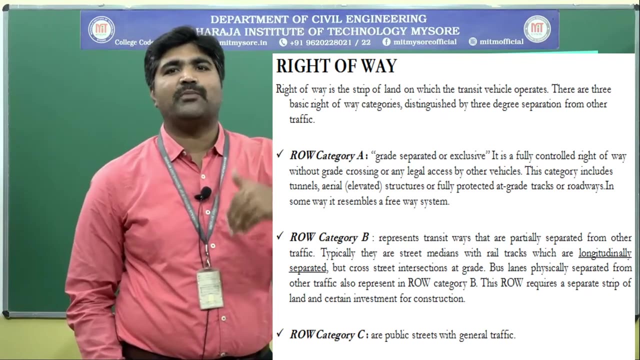 Separate BRTS bus rapid transit system lane is provided. In that way only the bus movement will be provided In Mysore also, you can see near palace For shorter stretch, near city bus stand for shorter stretch, only for city bus. they have provided separate way. 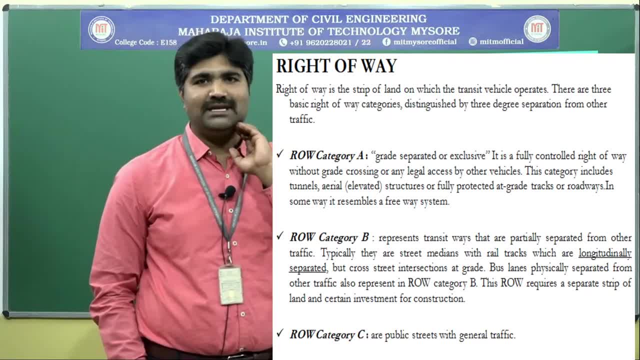 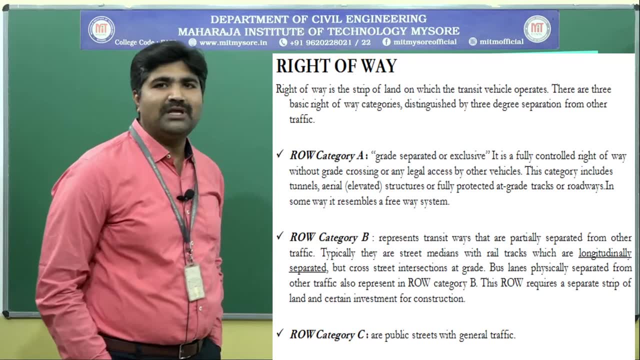 That may be for 0.5 kilometer. You can observe when you go into city. In Mysore city also it has been provided. Next, RW means right of way. category C, That are the public streets with general traffic. 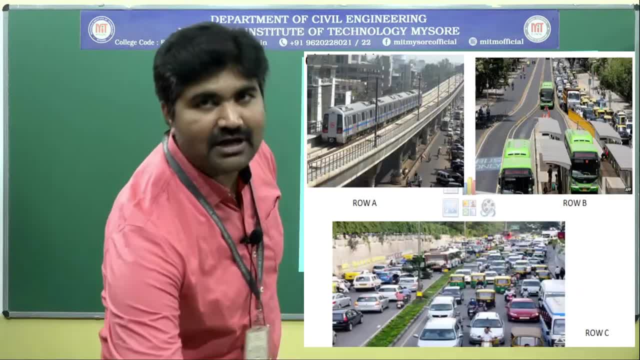 General traffic means that is the mixed traffic. See here in figure. you can observe here: Right of way category A. Right of way category A. In this there is a Right of way category A. Right of way category A. In this there is a. 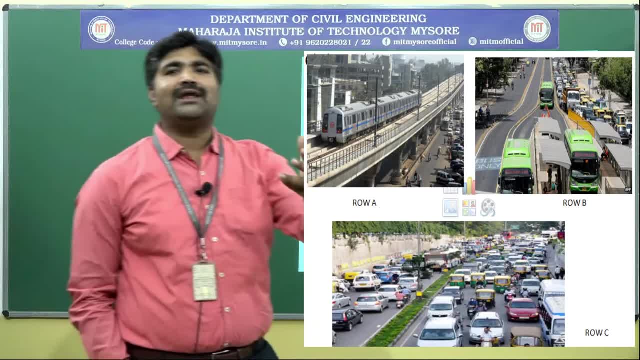 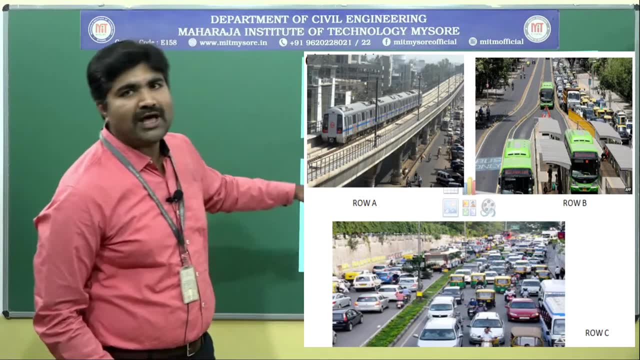 Great separated: Okay, This transit either moves through a tunnel or aerial structures. Aerial structures means that are the elevated structures, Means that are the flyovers. Okay, There will be no access for any other vehicles or persons, So there will be no congestion. 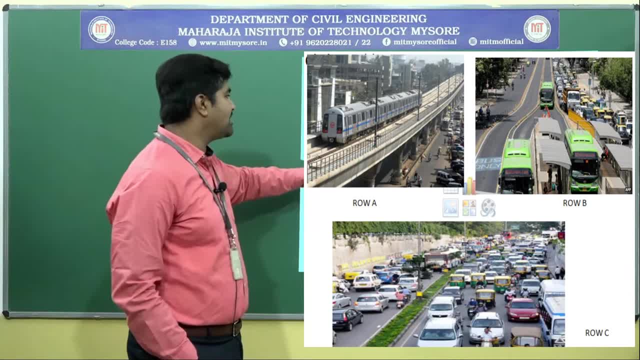 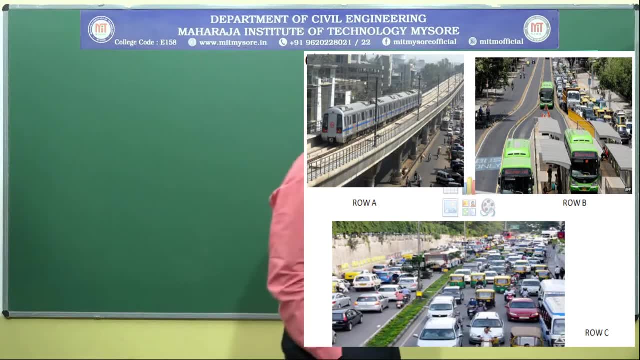 There will be faster movement of the vehicles. You can observe in the figure. This is the right of way, category A: Okay. Next right of way, category B: In this category: okay, the general in the where there will be a mixed traffic. 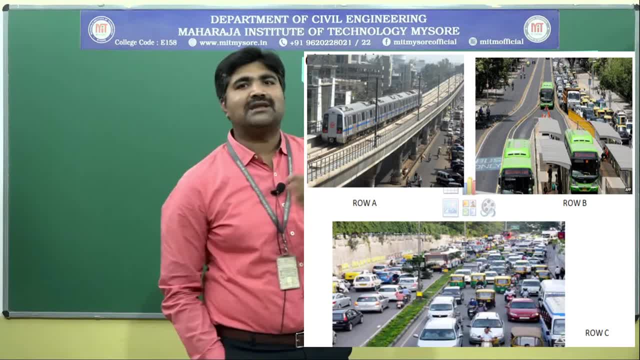 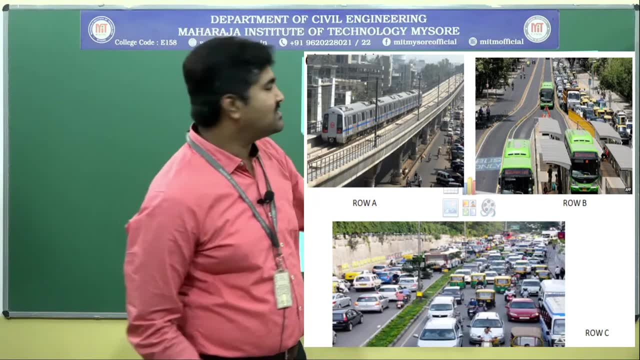 Okay, Here the bus. Okay, Here the bus transit. Okay, The mass transit will be separated longitudinally by providing the medians or curbs, or great separators. Okay, The mass transit will be separated Separate. Separate Lane are separate. 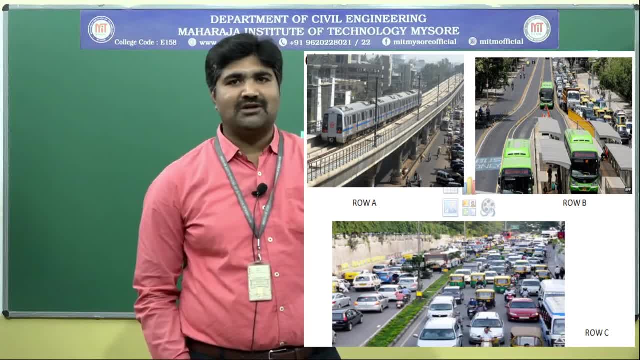 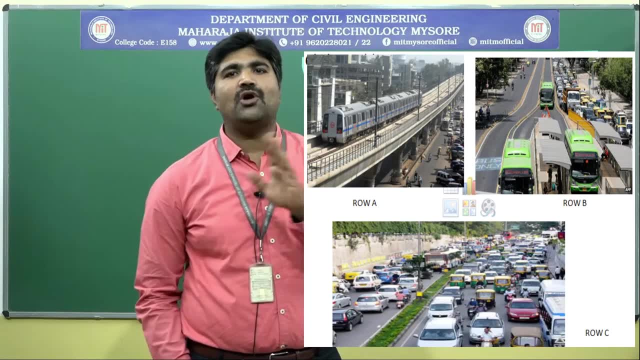 Track will be provided for the movement of mass transition. Okay. Mass transit- Orderly Okay. Bus- orderly Okay. Separate Tracker: Only there the bus movement will be allowed No access to other vehicles, So it increases the speed. 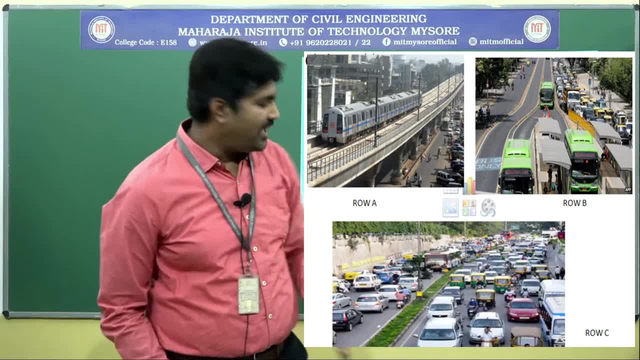 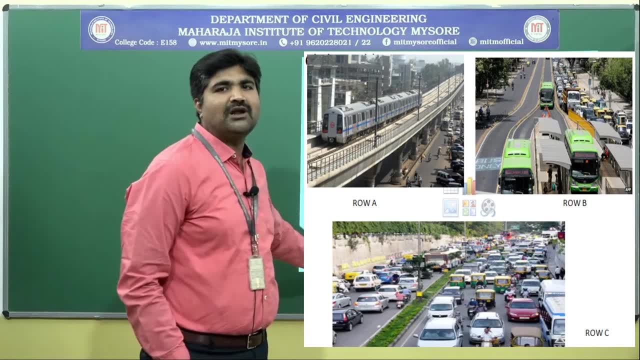 Okay, It increases the performance. It increases the performance of the mass transit. Okay. Next, in case of ROWC, right of way, category C. Here we can observe that are the public streets. General traffic will be there, mixed traffic. 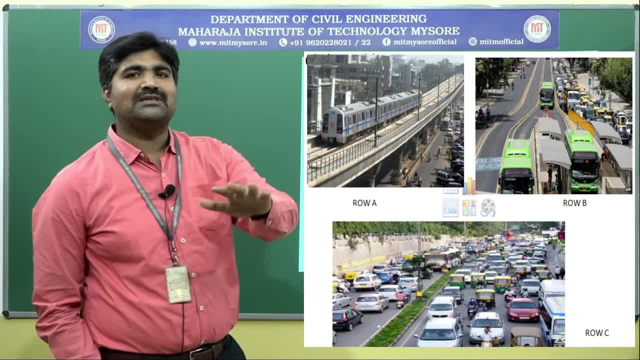 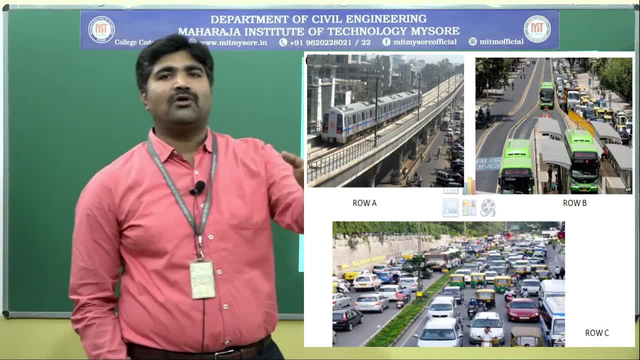 All vehicles will be there in a single lane. Okay Means in a single lane means it is in a track. All the vehicles will be operated, So there will be congestion. It takes more time, Okay. And also for public transportation because, as we know, the public transportation are large in size. 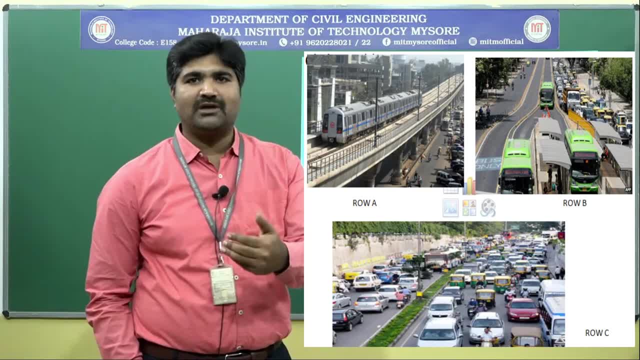 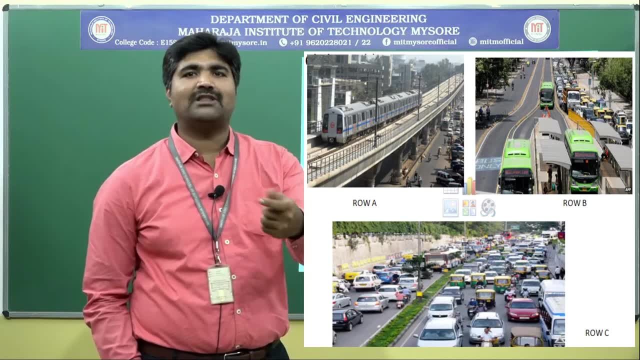 Okay, Bus when compared with the private vehicles, Maybe car or bike. Okay, When compared with that, this buses will have large in size. Okay, It will be difficult to maneuver. Difficult to maneuver means turning option or to handle Okay. 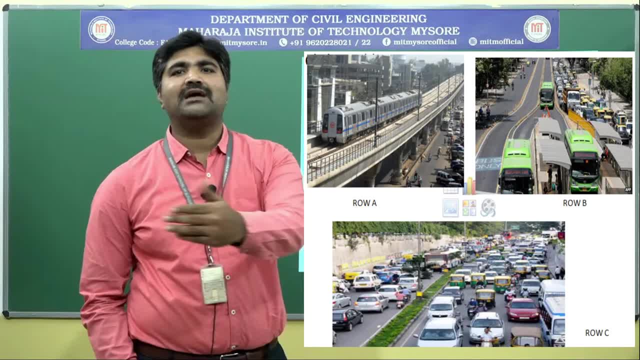 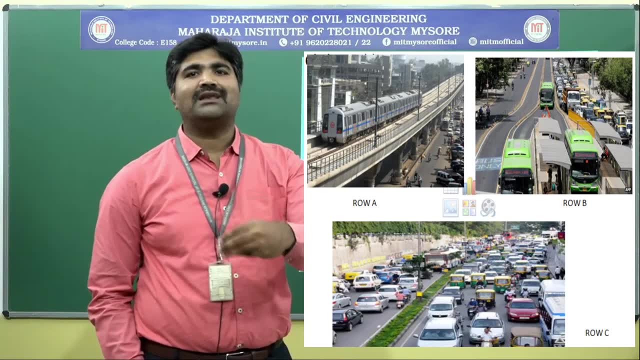 It will be very difficult, Right, If we have a bike or a car, we can easily turn, And our own vehicles means our two wheelers or four wheelers. We can travel speed. Okay, We can travel more speed. That is not possible for the mass transit. 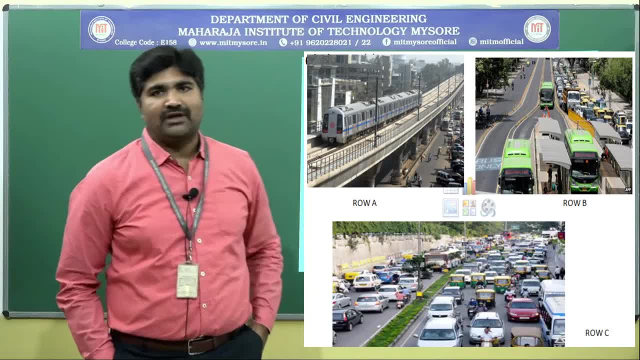 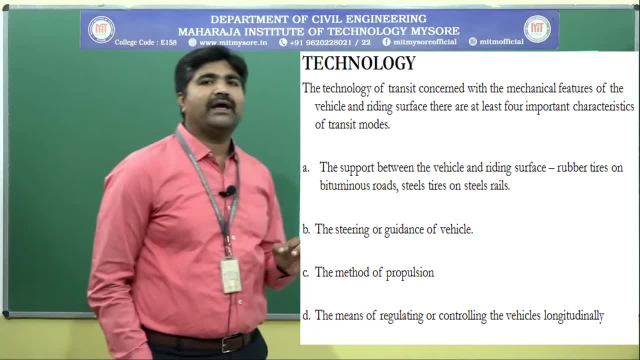 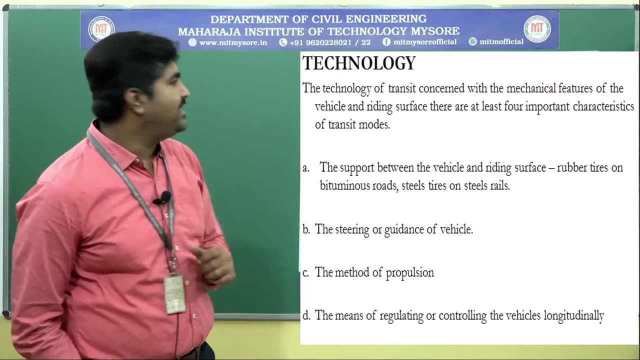 Buses are not possible In general Traffic, Okay. Next, Based on technology. The technology of transit concerned with the mechanical features of the vehicle and riding surface. Okay, It depends upon the mechanical features of the vehicle and riding surfaces, Okay. 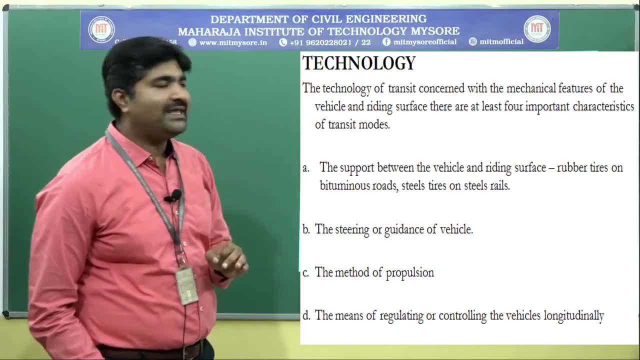 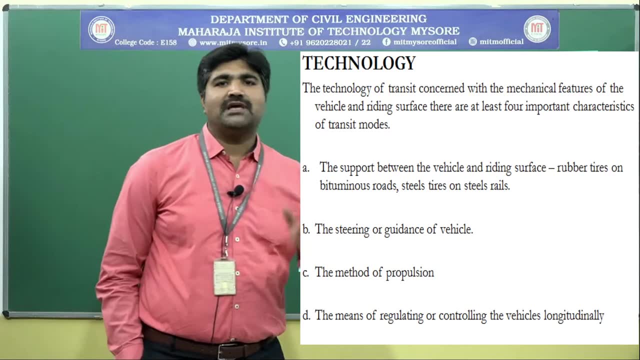 There are four characteristics. Okay, The first: The support between the vehicles. Okay, The support between the vehicles and riding surface. Okay, The rubber types on bituminous roads. See, as we know, the buses. What are the buses? There are rubber tires. 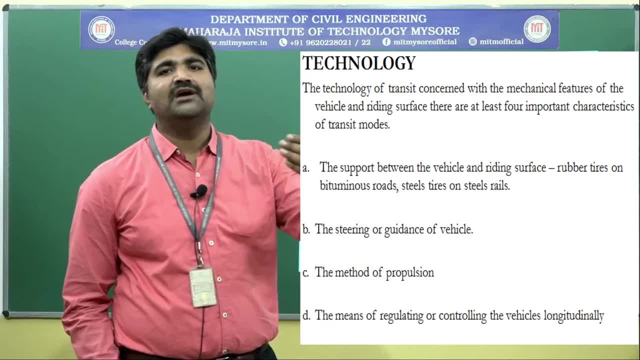 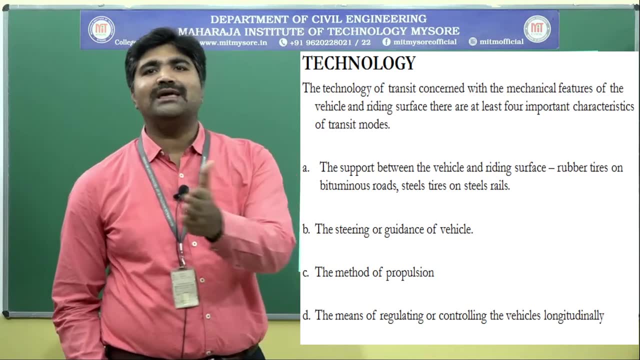 This will move on the hard surfaces. The hard surfaces means that are the bituminous surfaces or concrete surface. Okay, These pneumatic tires, rubber tires, cannot move on the smooth surface Right On the steel rail. It cannot move on the steel surface. 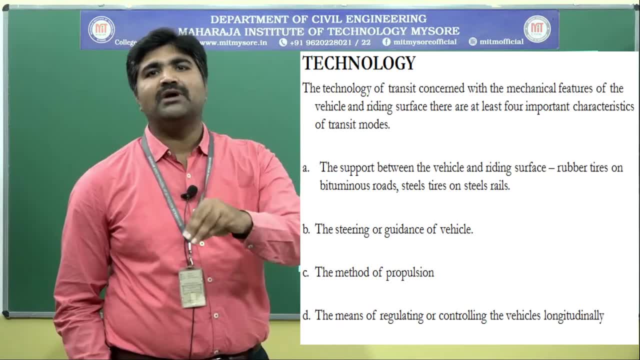 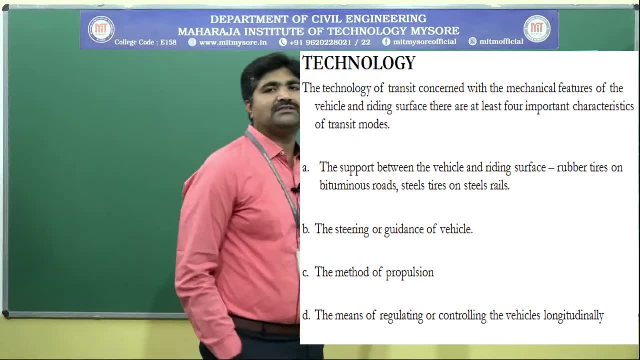 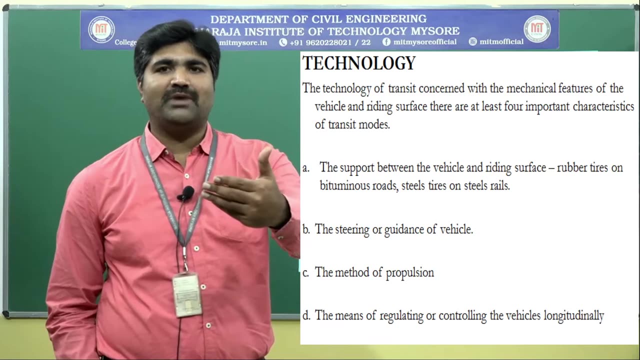 It requires some friction. Okay, Tire, Pneumatic surface requires some friction to move. It cannot move on the smooth surface. Okay. Next, Steel tires and steel wheels: See Tire and steel wheels That cannot move on the hard surfaces or bituminous surfaces or concrete road. 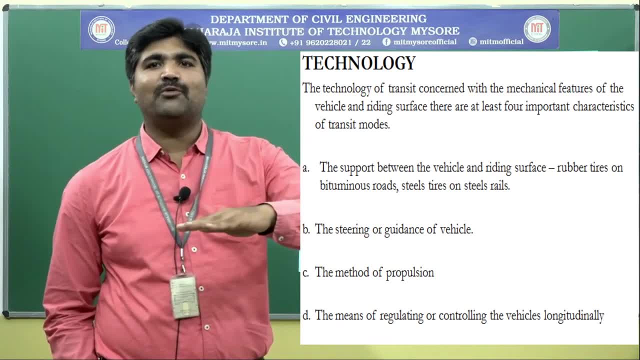 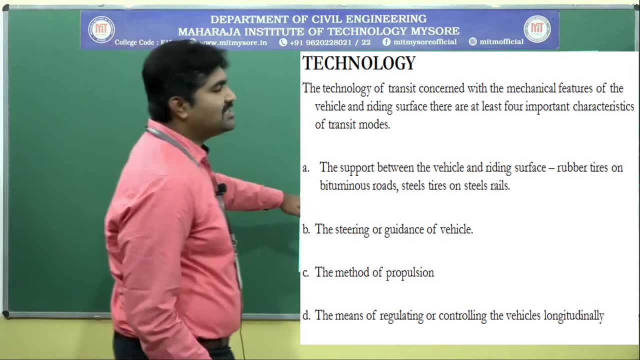 Because that has some friction. It resists the movement. So this steel rails will This steel wheels move on the steel rails. Okay, Next There will be steering or guidance of vehicles, As we know There will be For guiding purpose. 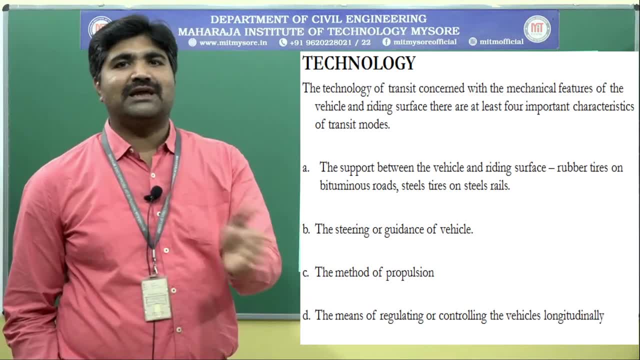 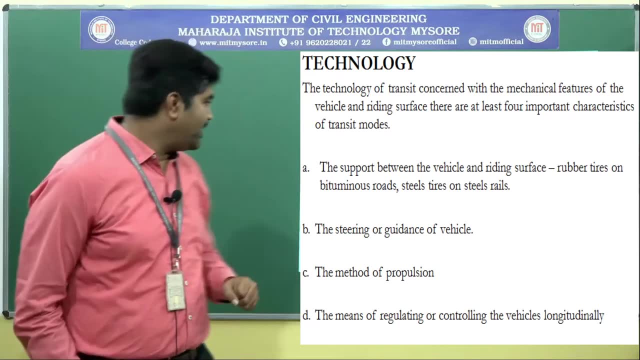 The steering will be there In the mass transit, In this rapid transit, Whether it is metro or monorail. What is there for this? There will be a. There will be a. automatic guidance will be provided. Okay, Next, The method of proportion. 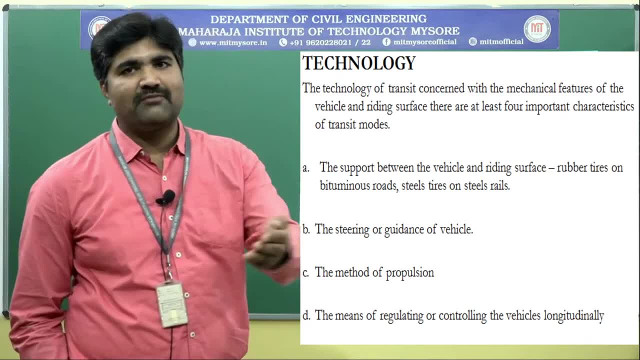 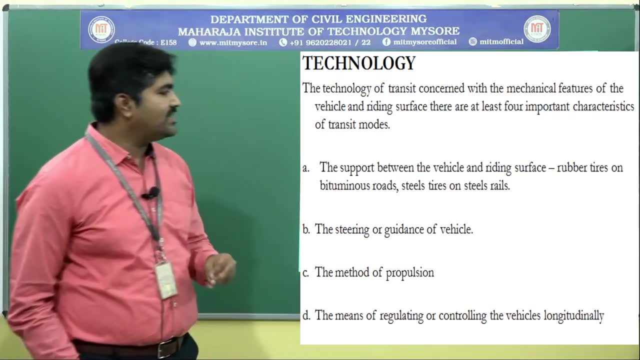 There will be change in engine For the bus. There will be different engines provided for metro and monorails. They have a electric traction, Okay. Lastly, The means of regulating or controlling the vehicles longitudinally. To control the vehicle longitudinally: 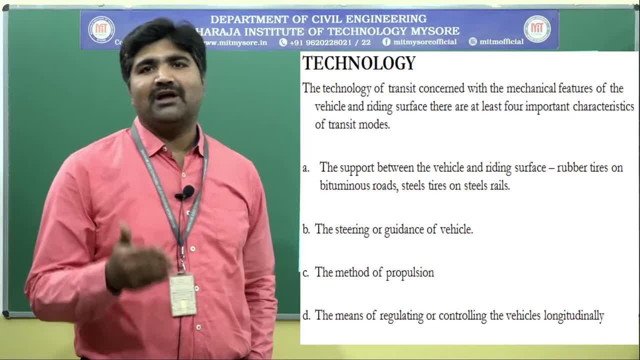 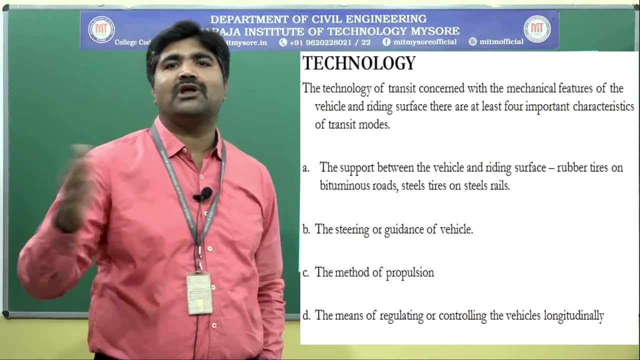 We will use different signal system: Right Surface transit, In surface transit, In road transit, There will be different signal system. Okay, Like this: This metro or monorail, They have a separate signaling system To control the movement of the vehicles. 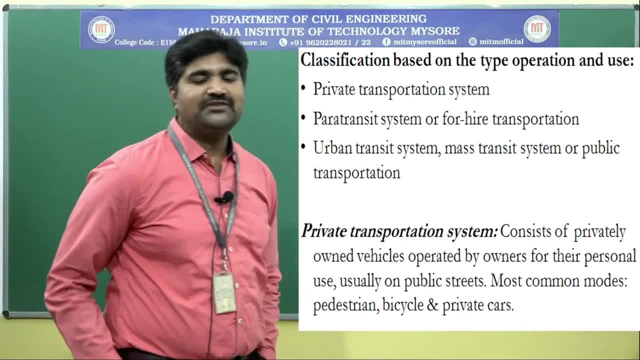 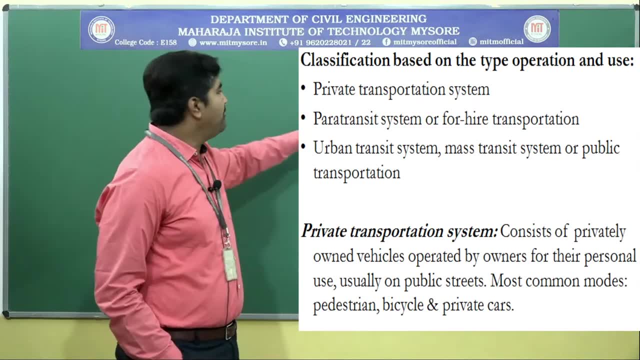 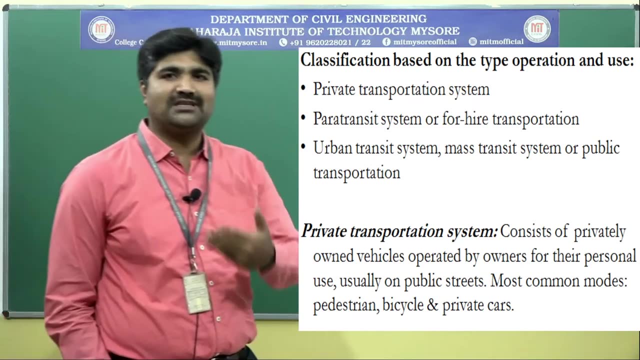 Okay. Next Classification based on the type of operation or type of service: Okay, Private transportation system, Paratransit or for air transportation. Okay, Urban transit system. or mass transit system or mass transportation. This is generally called Okay. 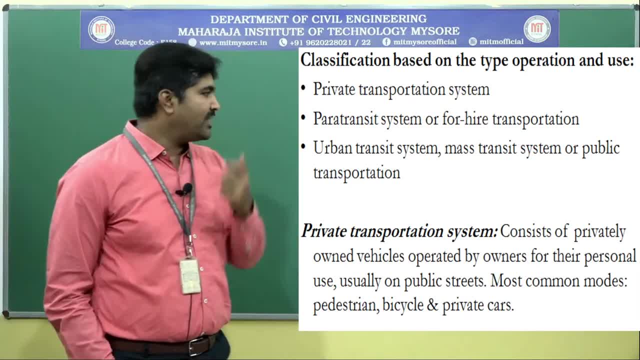 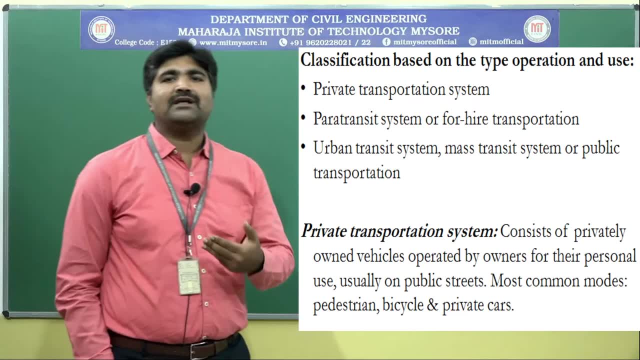 Private transportation system. What is private transportation system? Okay, See, Consists of privately owned vehicles operated by the owners for their personal use. Okay, Do you know what private vehicles are? Do you know what That are our cycles or bikes or cars? 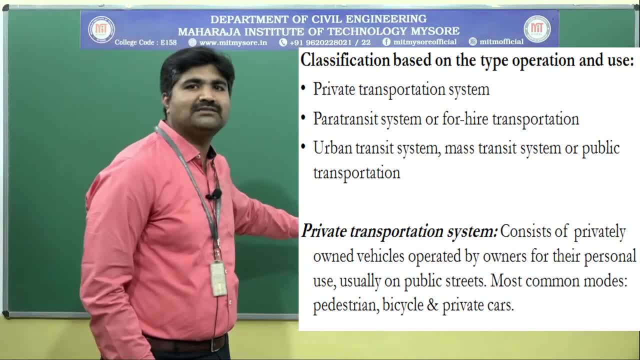 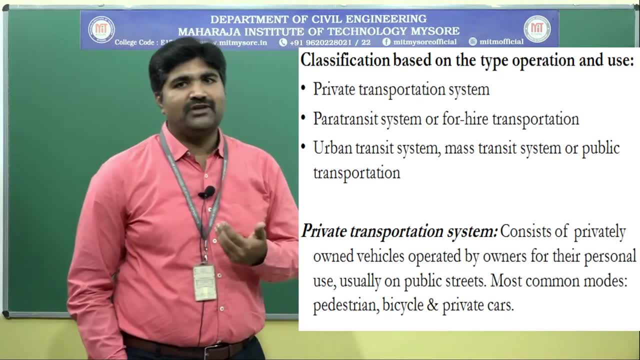 These are the personalized vehicles. We have more flexibility in case of personalized vehicles: Right The route that we need. We can run at the time that we need When we use the personalized vehicles. Next, Paratransit The term. 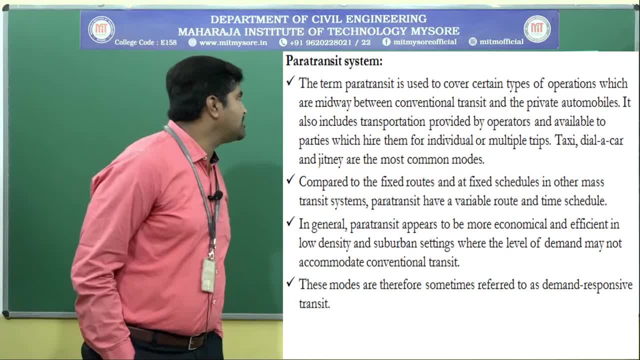 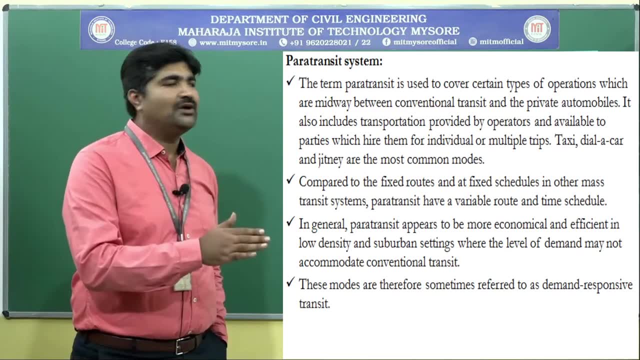 Paratransit is used to cover certain types of operation Which are midway between the conventional transit and the private automobile. Conventional transit means that is, the mass transit, Okay, And private automobiles means private transport- Our car and bikes- Okay. It also includes transportation provided by operators and available to parties. Okay, Paratransit. Actually, paratransit or air transportation means vehicles used for traffic. That may be Caps Or small cruisers That are the paratransit. 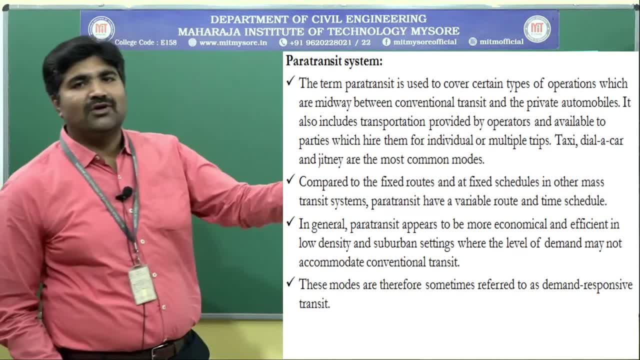 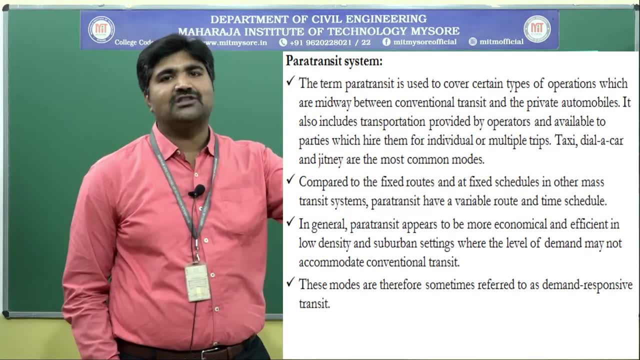 Okay, See Here, When compared with the mass transit. Okay, The mass transit. In case of mass transit, there will be rigidity. In case of fixed, There will be, The route will be fixed And also the schedule will be fixed. 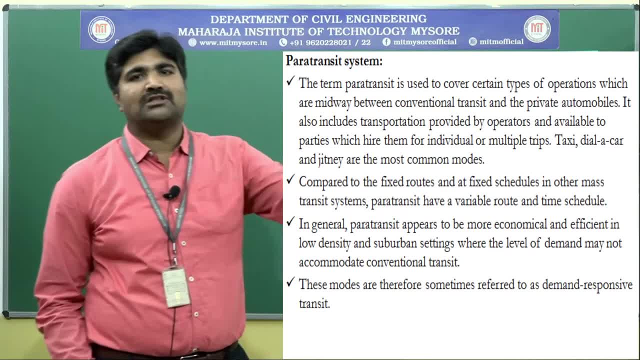 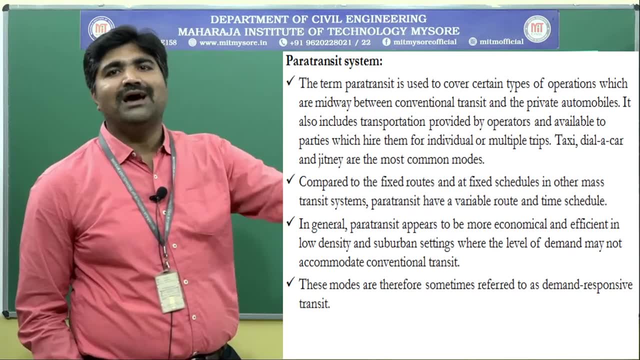 Right Train or bus. What happens? Route is fixed. It goes on the same route. No other route can be changed. Same way Schedule. If it is 11 o'clock, It is scheduled at 11. For that time it will run. 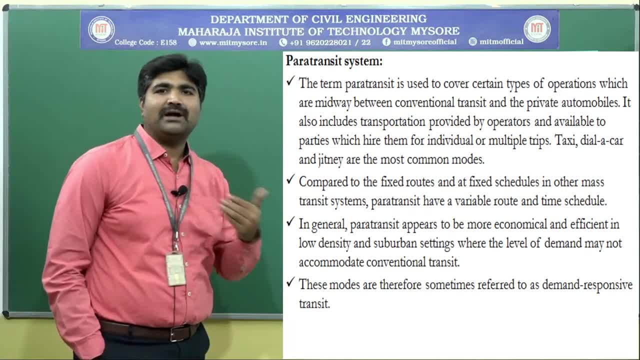 But in case of fire, transit For us, For the parties Who need the paratransit? Okay, That depends upon them. They can choose the route and the schedule. Okay, In general, Paratransit appears to be more economical and efficient in low density areas. 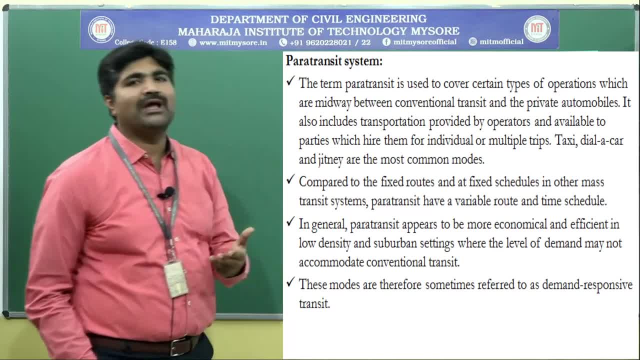 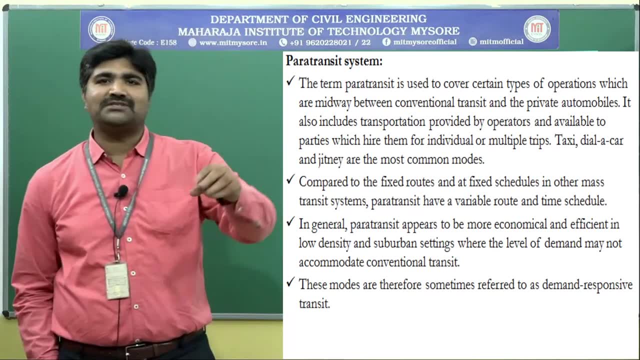 Okay. And in suburban areas: Okay. Low density areas Where the population is less, Where we are giving mass transit, That will be underused. Okay, Use the ugly. It will be lost. Economically, it will be uneconomical. 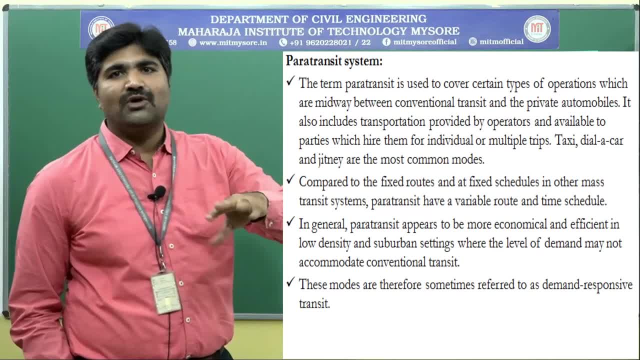 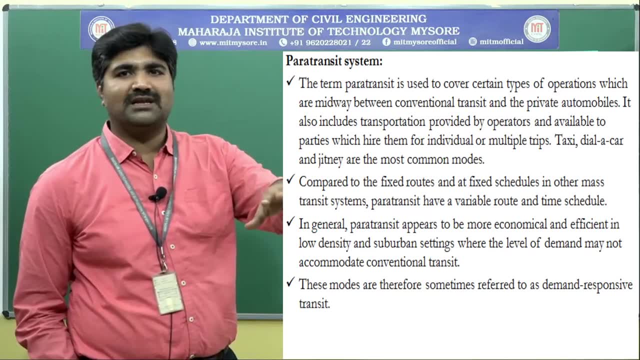 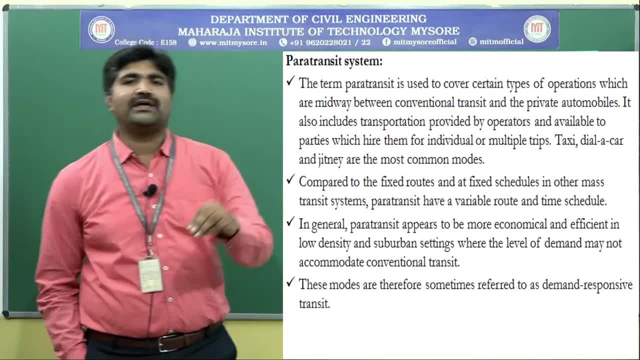 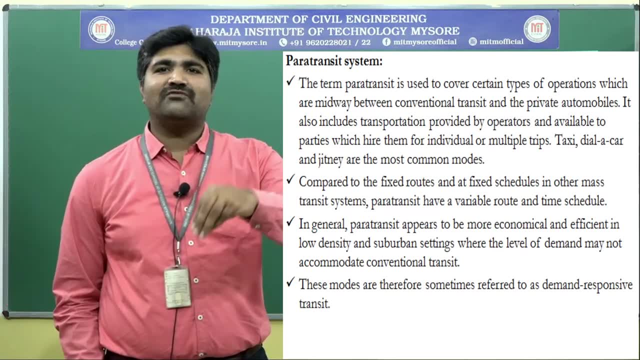 Okay, It will be uneconomical. Okay, And also suburban areas. If you take example Mandia district Or Ramnagar, These are the smaller districts. Okay, We cannot provide the public transportation for all the wards, Or we can't provide for all the areas. 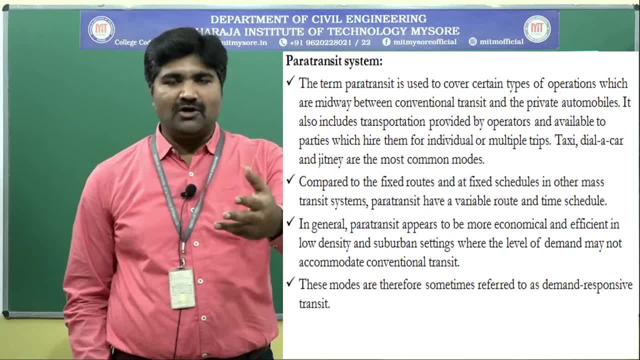 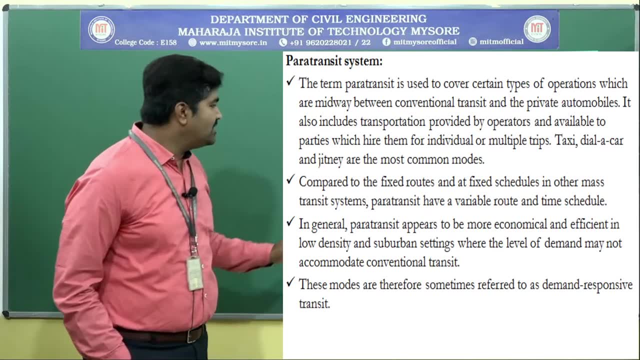 Due to the restriction of the land, Means, road width and all. Okay, There it is This type of high transportation. Okay, Paratransit will be more useful. Okay, These modes are therefore sometimes referred to as demand response. Okay. 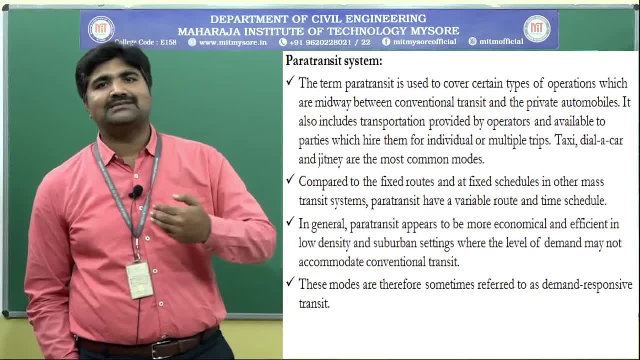 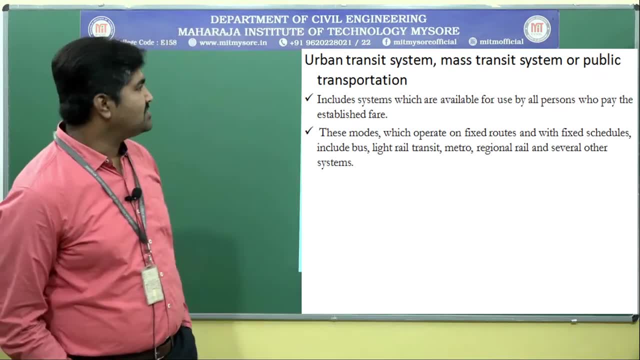 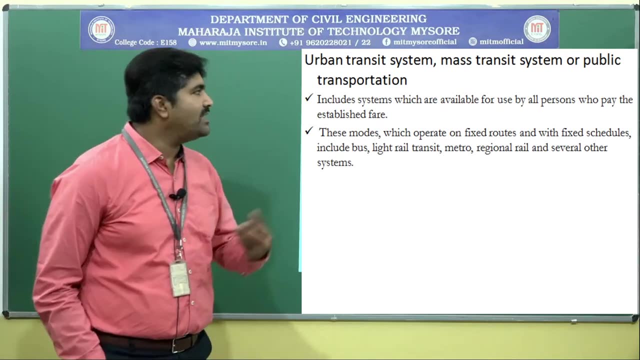 It will be more responsive to our demand. Okay, It will be more responsive to our demand. Okay, It will be more responsive to our demand. Okay. And next, Urban transit system or mass transit system or public transportation: Okay, See, this system includes which are available for use by all the persons who pay the prescribed. 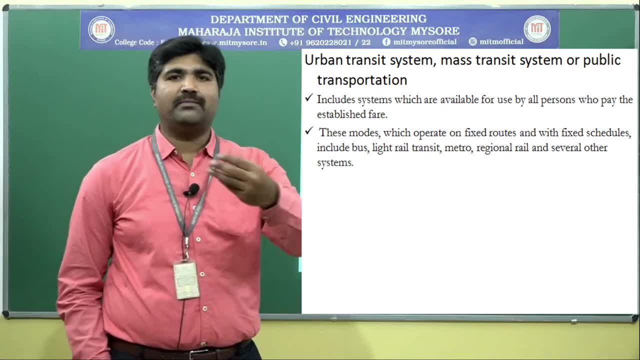 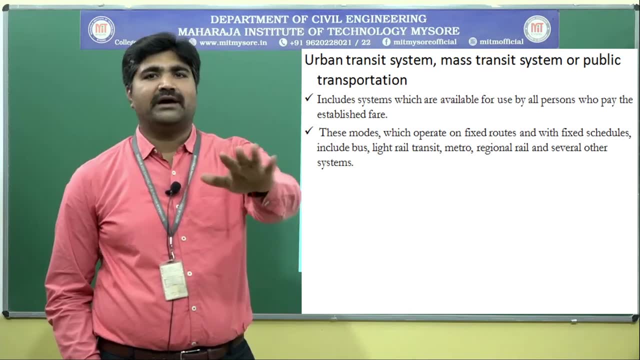 fare: Okay, There will be prescribed fee by paying that everybody can use. Okay. Public transportation: There will be equal access to all. Everybody can use by paying some fixed rate or the fixed fare. Okay, These modes, which operates on fixed modes and the fixed schedules will be there. 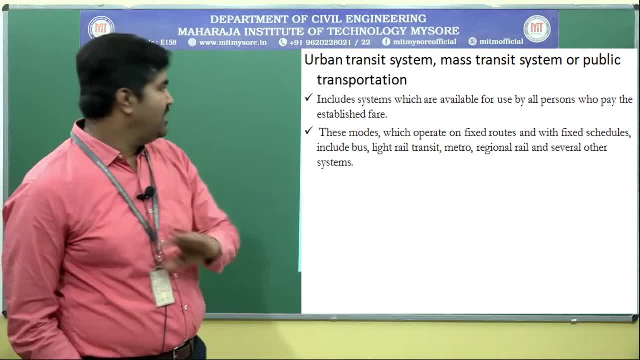 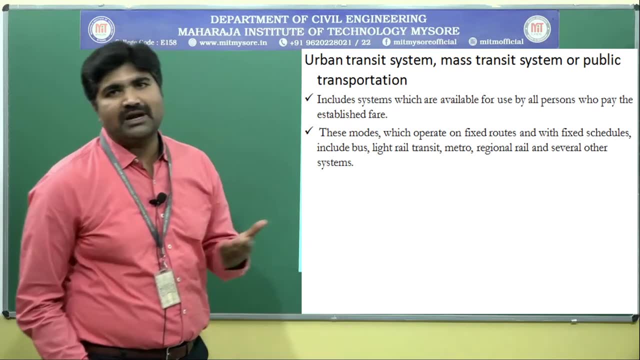 Okay, The route will be fixed and the schedules, the timing, will be fixed. Okay, This include bus, rail transit, metro, regional rail, several other system We know. suburban rail is there, Bangalore, you can take example, monorail is there. 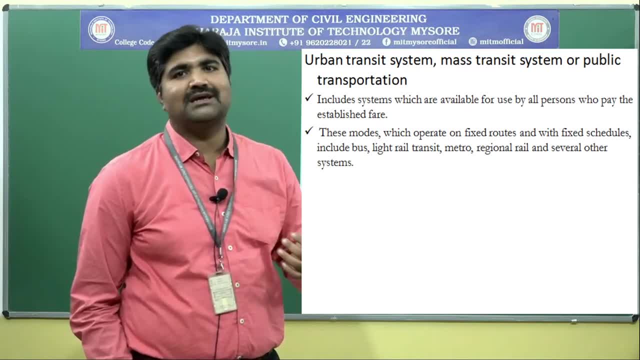 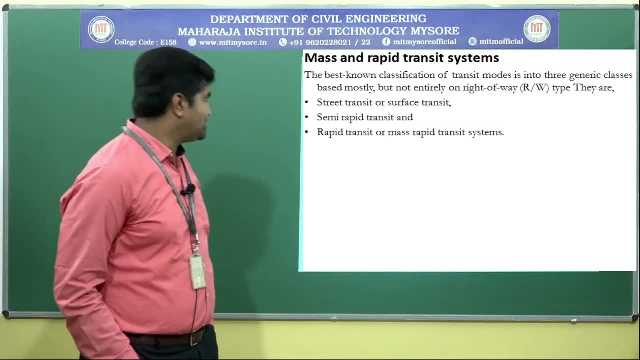 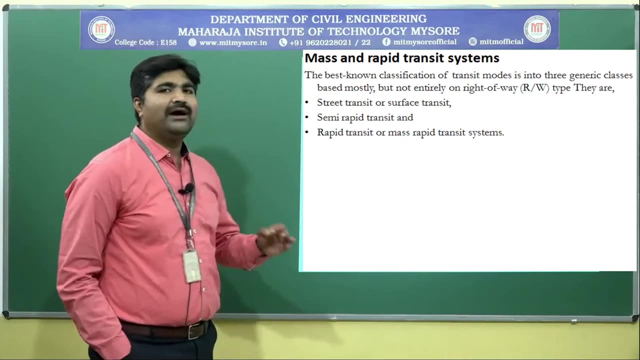 Suburban rail is there. Okay. Bangalore BMTC buses are there. These are the mass transit: Okay. Next, Mass and rapid transit system: Okay. The best known classification of transit modes into three generic classes based mostly, but not entirely, on right of way. Okay, They are street transit. Street transit means that are the surface transit. Okay, Next, Semi-rapid transit. Lastly, that is the rapid transit or mass rapid transit system: Street transit, as the name indicate. Street, as you know, surface transit, it is. 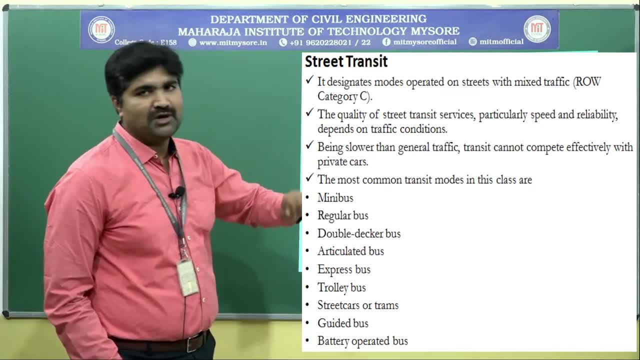 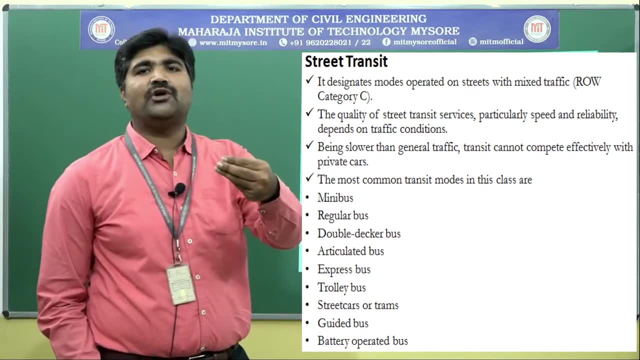 It designates. It designates modes operated on streets, Modes operated on roads, with mixed traffic which falls under a right of way category C. As we know, in right of way category C there will be a mixed traffic. Mixed traffic means all traffic. 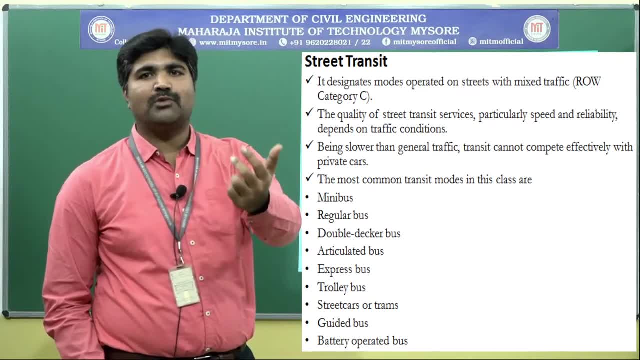 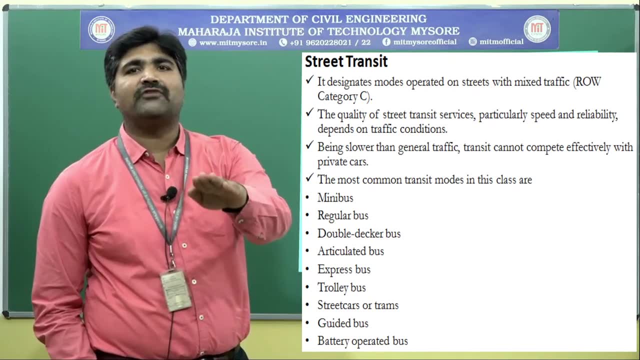 All vehicles. you know there will be movement. Okay, Slow moving vehicles, Bullock cart, cycle car, buses, trucks, everything will be there in the mixed traffic. Okay, That falls under the right of way. category C: The quality of street transit service, particularly speed and reliability. 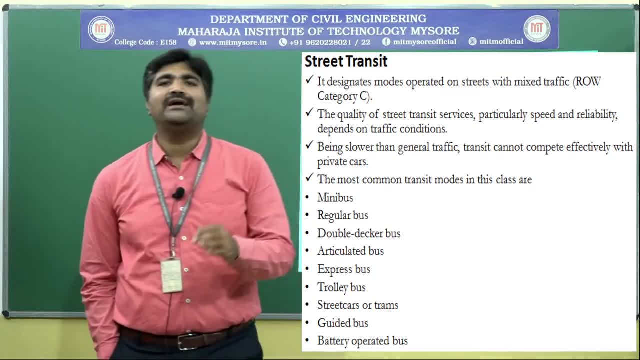 Depends upon the traffic condition. It depends upon the traffic condition Means, as we know, traffic. Now there is congestion. What happens? Speed automatically reduces. Level of service decreases. So reliability- What happens to our dependence on that? It will become less. 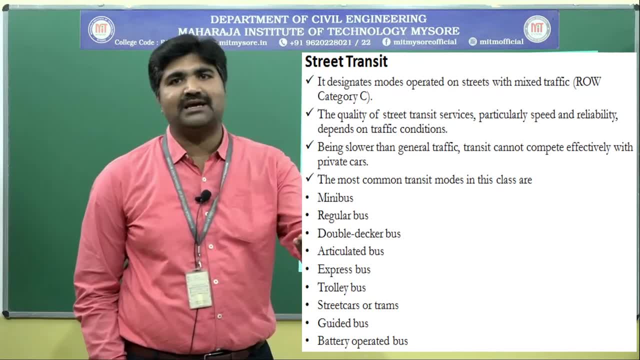 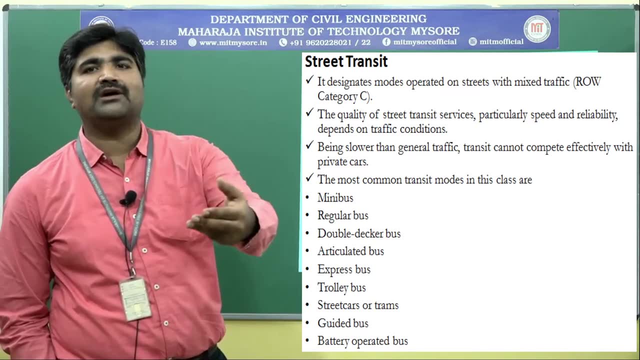 Because travel time increases, Then our dependence on mass transportation, Reliable, Decreases. Okay, Okay, This discourages to use the mass transportation. Okay, Next See Being slower than the general traffic. You see, You see, You see. 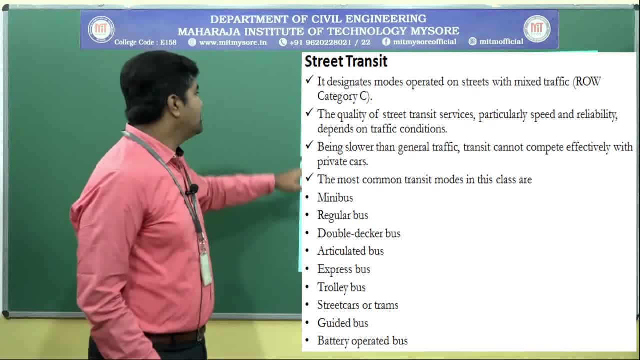 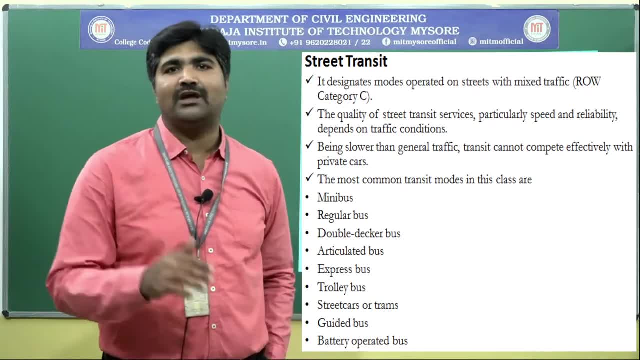 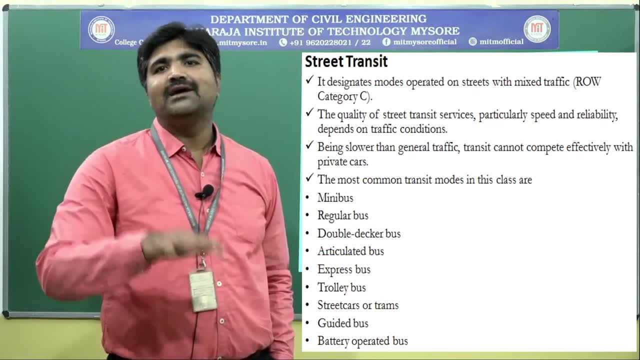 Okay, Buses were always of bigger size To man over To handle on the road. Okay, we cannot easily handle the buses. okay, Right Bus, we can't easily turn 2 wheeler, 4 wheeler easily, but it can't be turned. 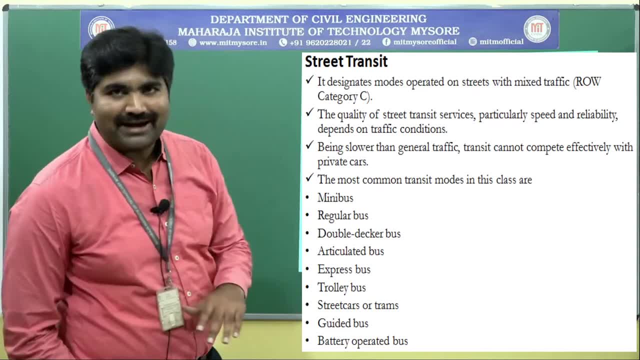 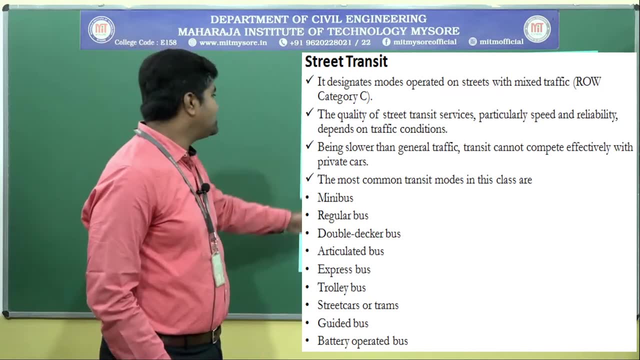 okay. So it has to be moved slowly when compared to the private transit service, So it takes more time. See: the most common transit modes in this class are: this class are okay. there are various transits: mini bus, regular bus- okay, double decker bus. 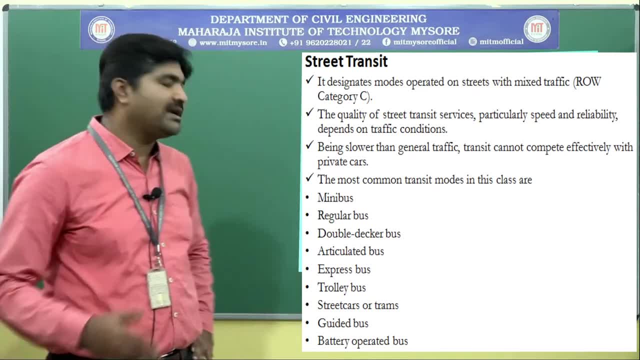 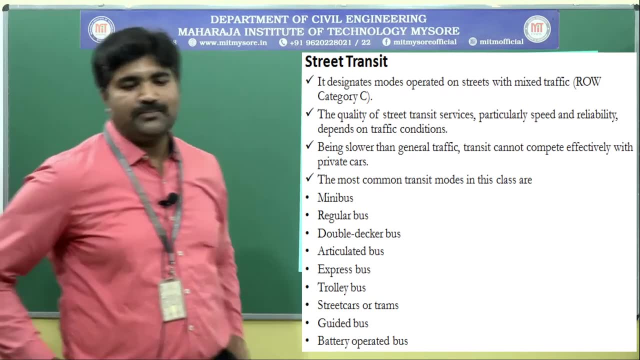 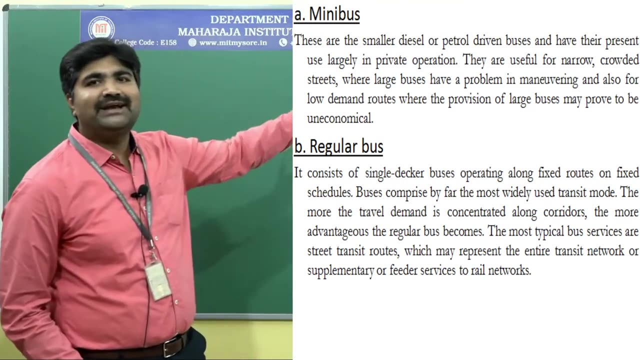 articulated bus, express bus: okay. trolleys. trams, guided bus, battery operated buses: these are the some of the vehicles which are used on the street transit, okay, okay. next, mini bus: okay, which falls under the street transit? okay, mini bus. see, these are the small diesel or petrol driven buses. okay, 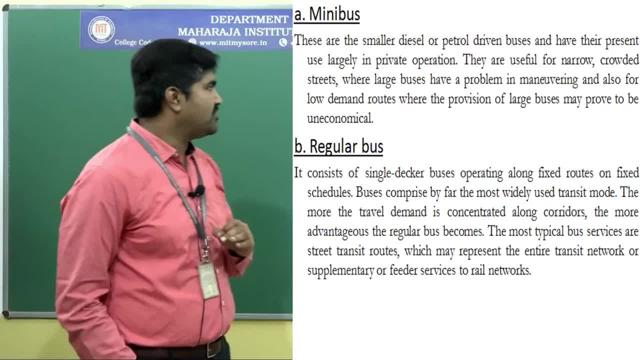 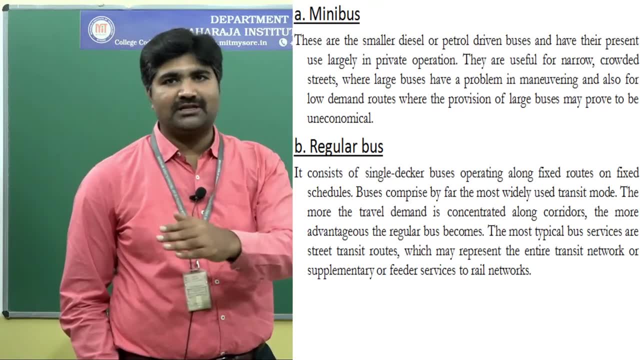 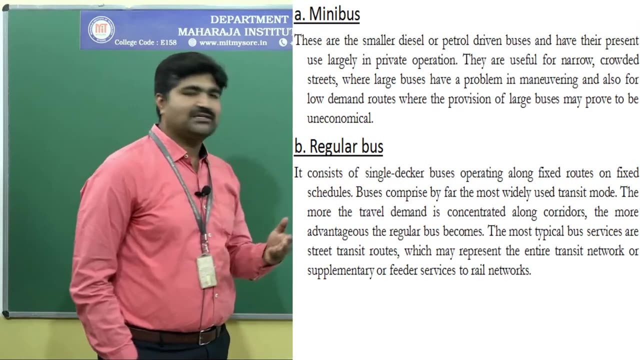 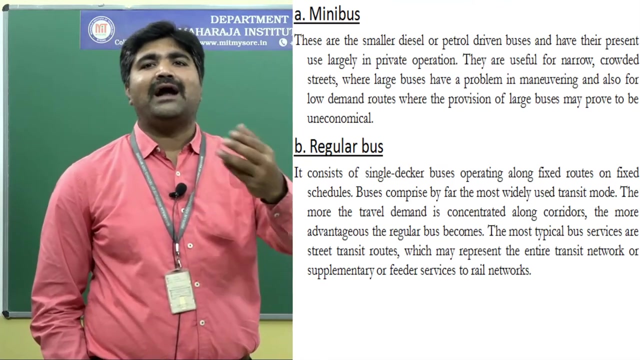 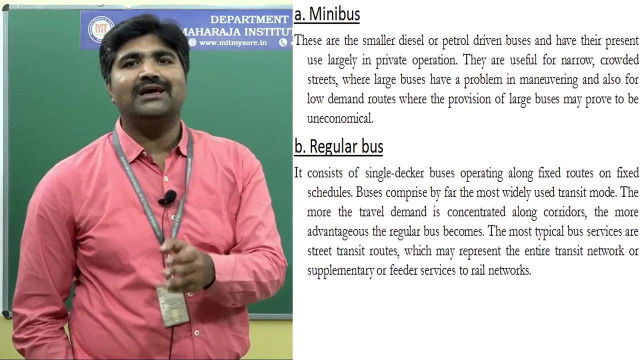 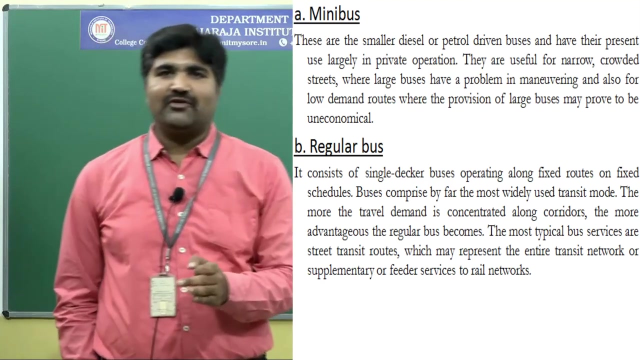 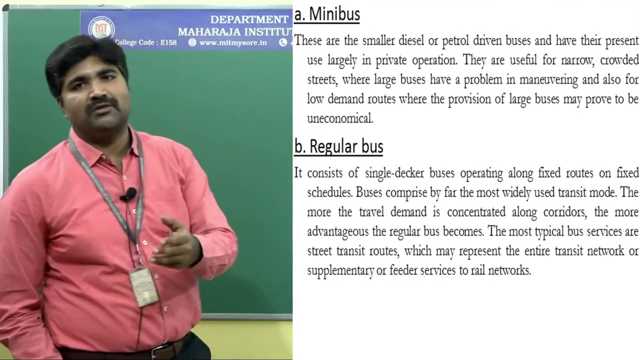 and they're present used largely in private operation, very cumbersome, difficult in the narrow streets. so at that time we will prefer the mini buses. and also, where the density will be less, okay, density of population will be less there. also there we will provide the mini bus instead of the regular buses. regular buses provided. 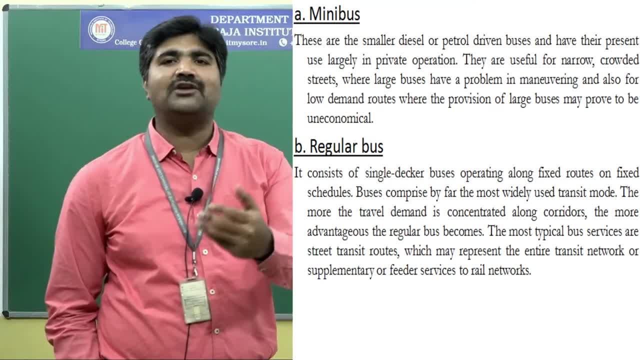 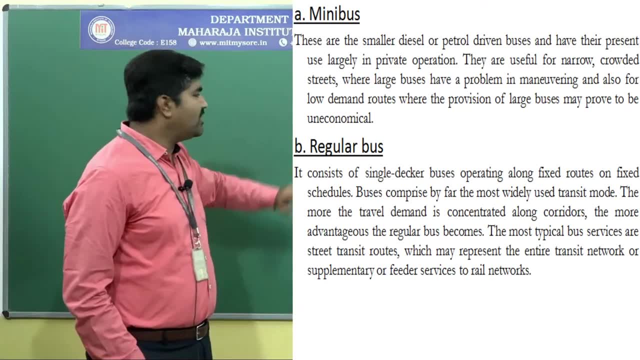 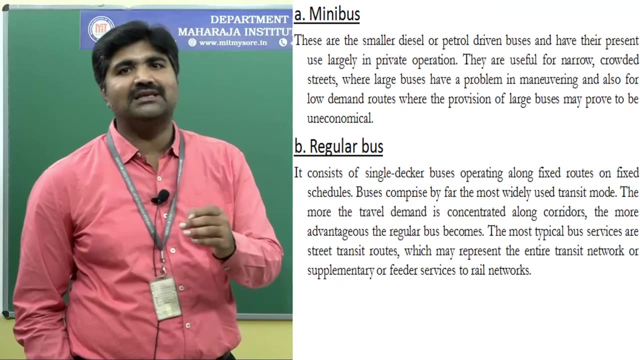 mass transportation. sufficient use, underused, it will be economical. okay, at that time also, we will provide the mini buses, okay, and next, regular bus, regular bus. regular bus. that are the city buses. now bus node is the mysore city bus or bengalore bmtc buses. that are the city buses. 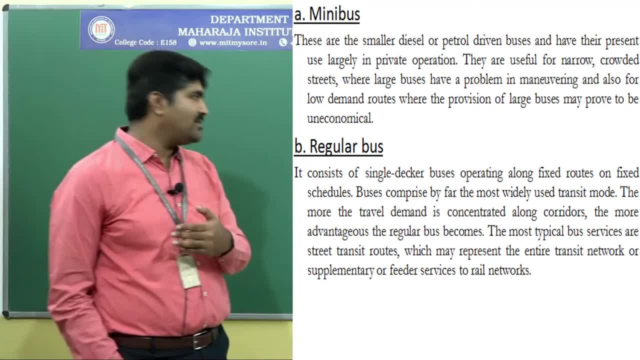 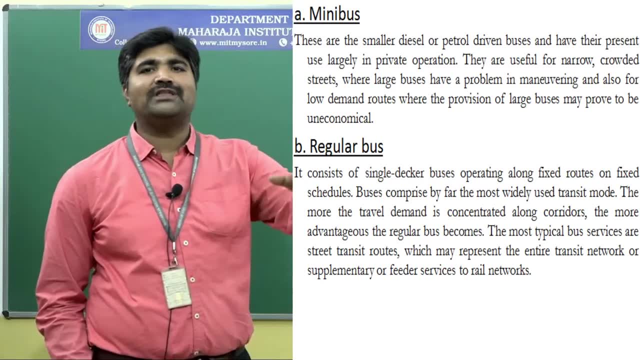 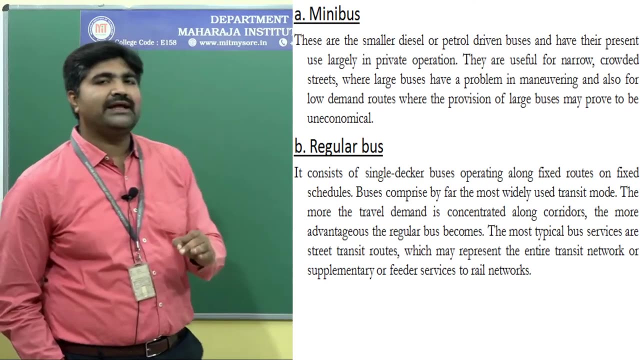 means that are the regular buses. okay, it consists of single decker buses, okay, operating along fixed routes. the routes are fixed and the schedule will be fixed. we have, we have to follow the schedule, okay, see, the most typical bus services are street transit routes, which represent the entire trans. 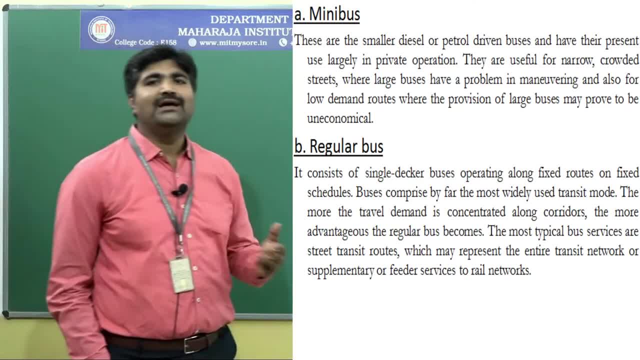 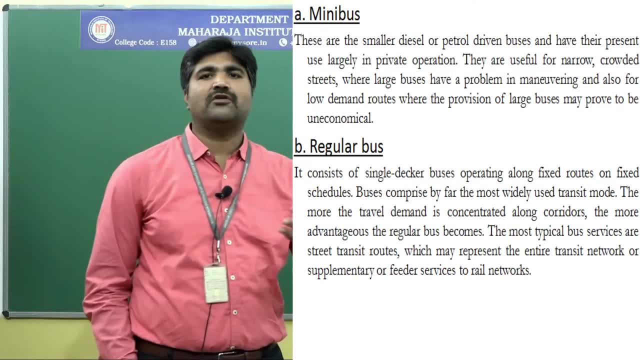 network, transit network or supplementary or feeder system. okay, this: regular buses may be usually used in the city buses, but in the city buses they are not used in the city buses for the regular trips, our day-to-day trips. that may be for school going trips or working. 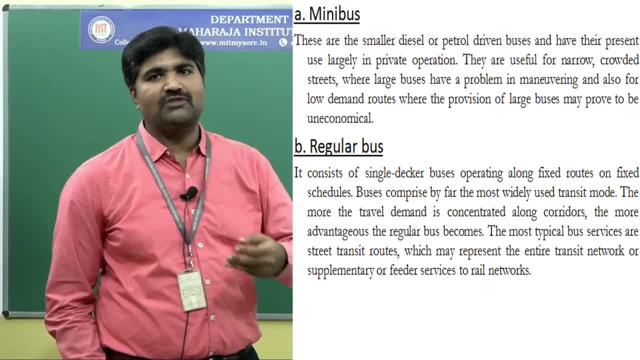 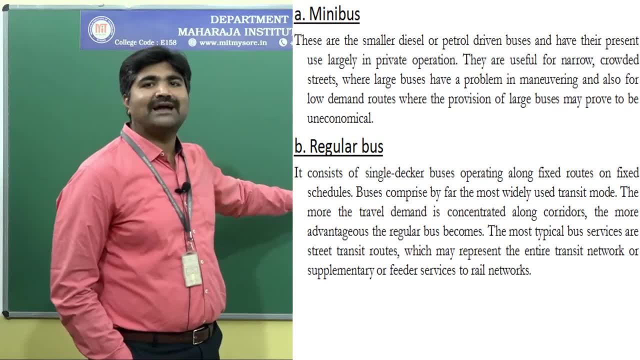 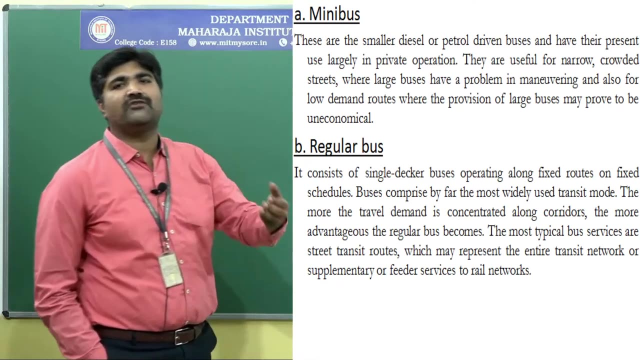 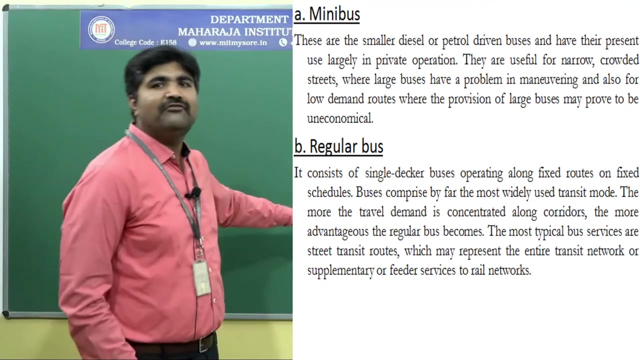 purpose trips or recreational purpose trips or social service trips, for that we will use the regular buses. and also this acts as a feeder system to other network, other transportation network which acts as a feeder system, other transportation network that may be railway network or airport or ports, for that all it acts as a feeder system, for that all it acts as a. 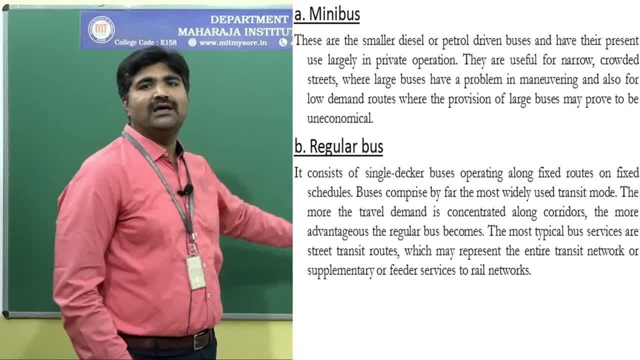 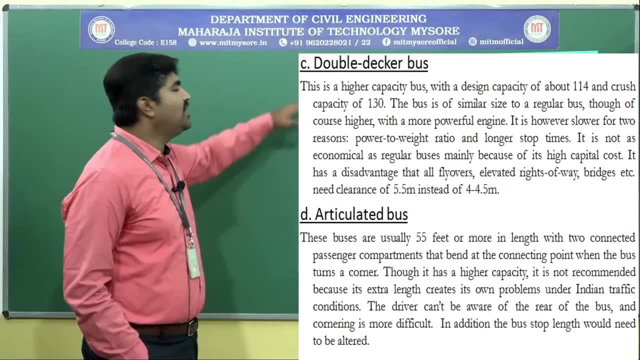 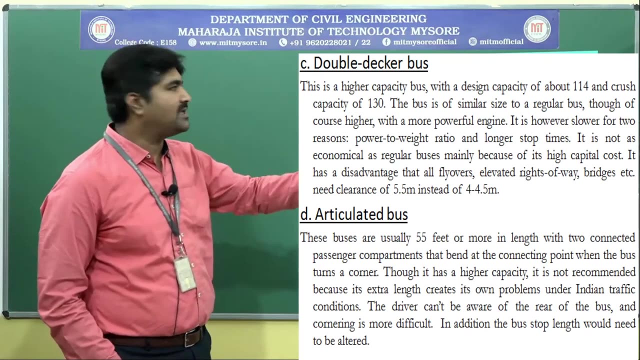 feeder system. okay, to reach the terminal station. this will help. okay. next, dapple decker bus: okay, as the name indicates, it has a. two deckers means two floors will be there. okay, this is a higher capacity bus when compared to the regular bus. this has a higher capacity. okay, with a design capacity. 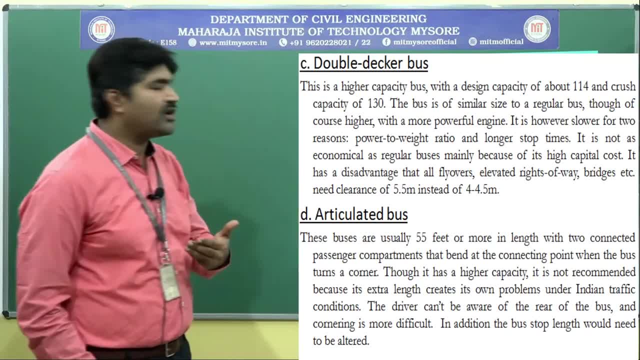 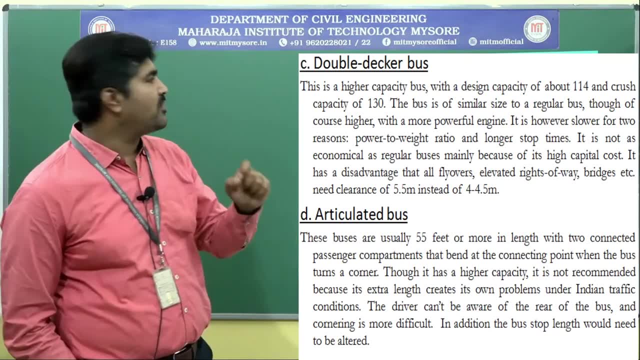 of about 114- 114 and crush capacity of around 130. okay, see, the bus is similar to regular bus, but there will be a two floors and it will be a feeder system. okay, to reach the terminal station. it is provided with a more powerful engine. okay, it will be provided with more powerful engine, it is. 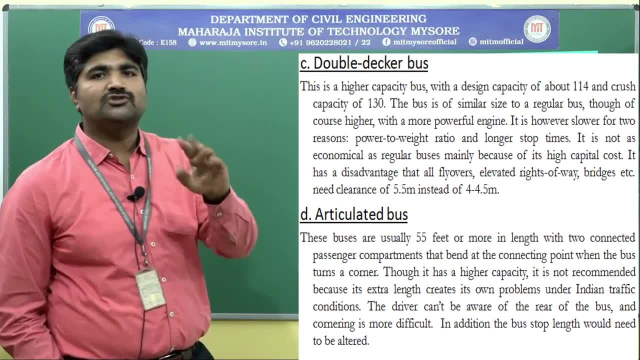 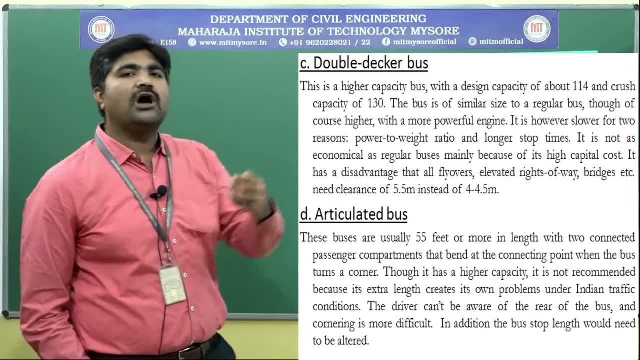 however slow, for two reasons. okay, for two reasons it will be slow. yeah, those are two reasons. so that is power to weight ratio means power to weight ratio, okay, and longer stop times. as we know, the capacity is higher, the more number of passengers can be accommodated here. okay, nearly. 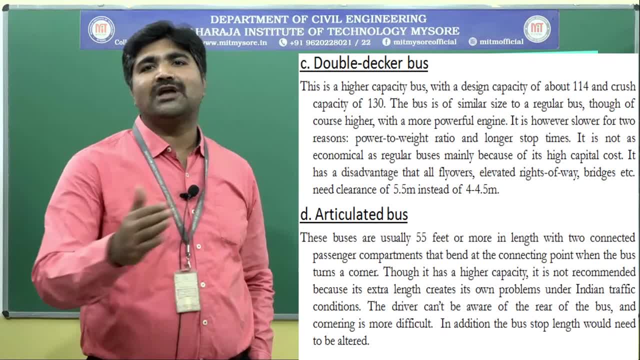 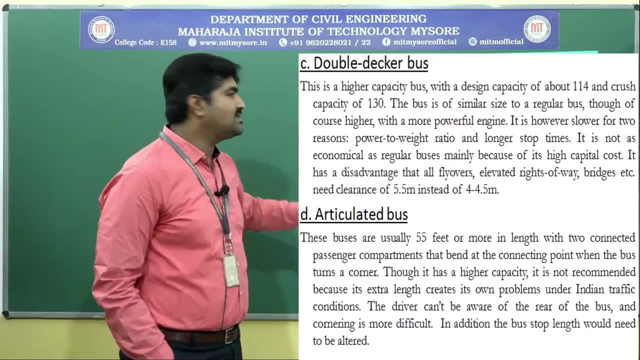 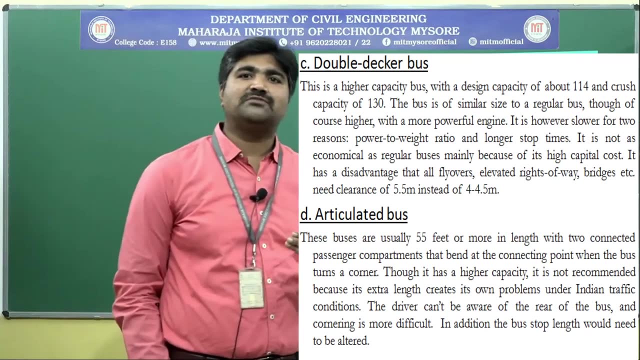 100 plus. okay, this passenger check-in and check-out ugly. it takes some more time. so there will be stoppages. time will be more in case of these buses. okay, it is not as economical as regular bus. okay, it is not as economical as the regular bus because the initial investment will be. 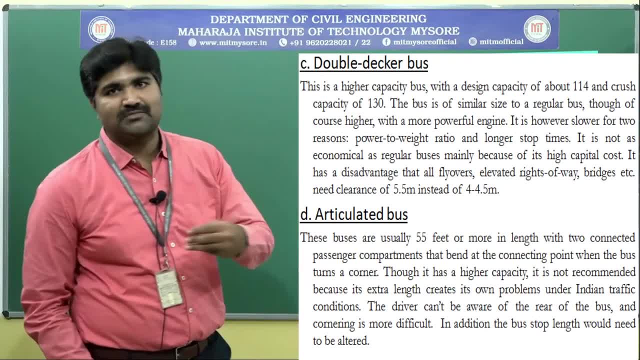 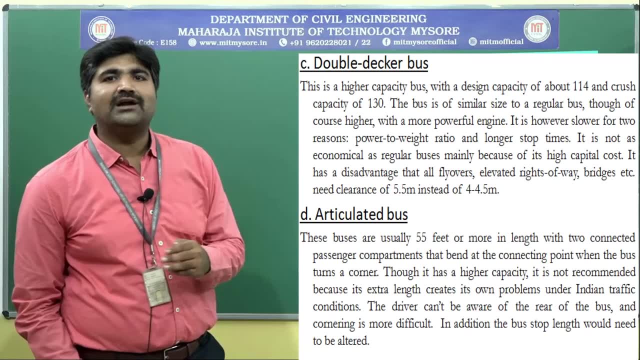 higher than than the regular bus. okay. initial investment cost, purchase cost to just see that. okay. and also there, that has some disadvantages. another disadvantages: so it cannot easily go through the flyover underpass because there will be a clearance. it requires some clearance of 5.5. 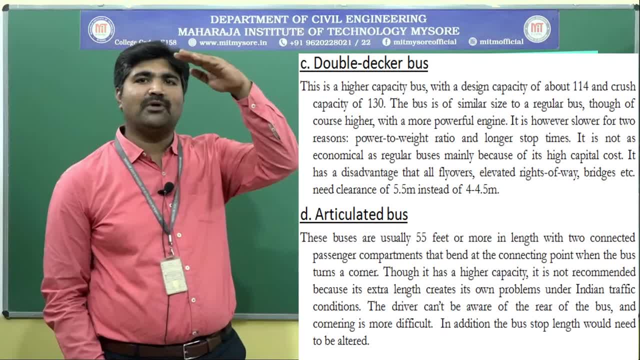 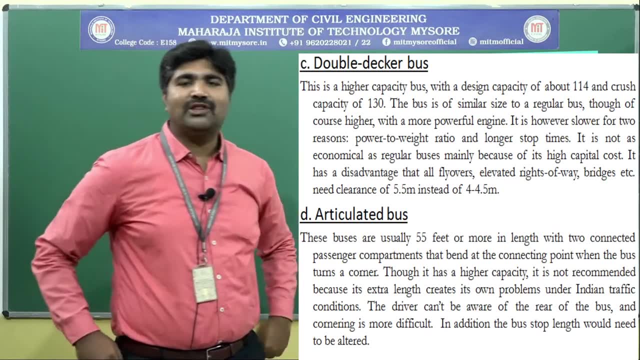 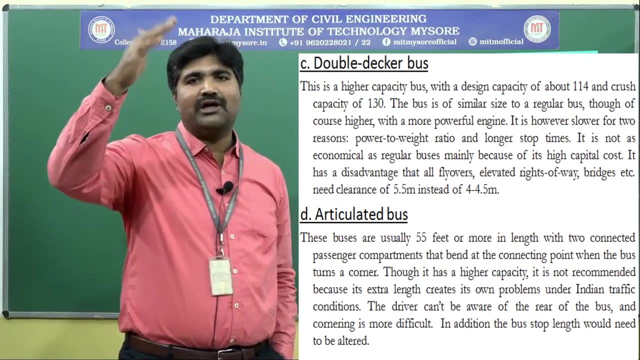 meter. okay, clearance here back, oh, clear. and cylinder to the top. okay, top surface of the bus. that will in, that will touch. okay, that won't allow the movement with a kid. yeah, so there will be sufficient clearance here back. oh, okay, as you know, double-decker passenger. I'd just hear to that, okay. 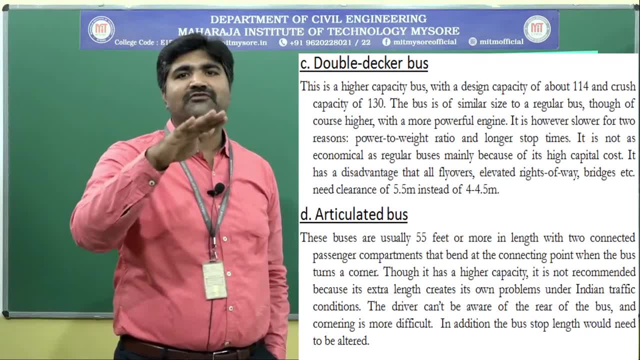 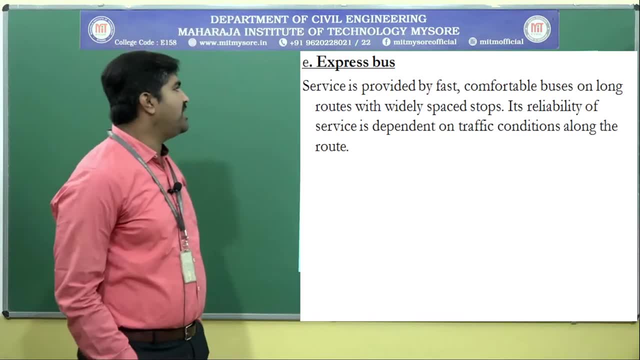 underpasses a Lala move ugly care, ha Gala. it requires some sufficient clearance here back, oh, okay. next, express bus. okay, service is provided by fast, comfortable buses on along the express bus. okay, service is provided by fast, comfortable buses on along the express bus. service is provided by fast, comfortable buses on along 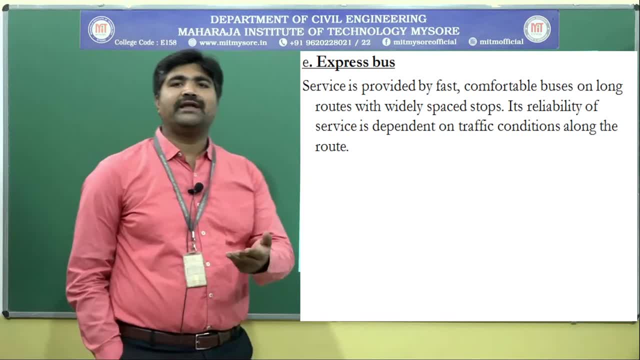 routes with widely spaced stops. okay, see, as you know, you can take example of bangalore airport bus routes with widely spaced stops. okay, see, as you know, you can take example of bangalore airport bus routes with widely spaced stops. okay, see, as you know, you can take example of bangalore airport bus from majestic to airport. they travel. 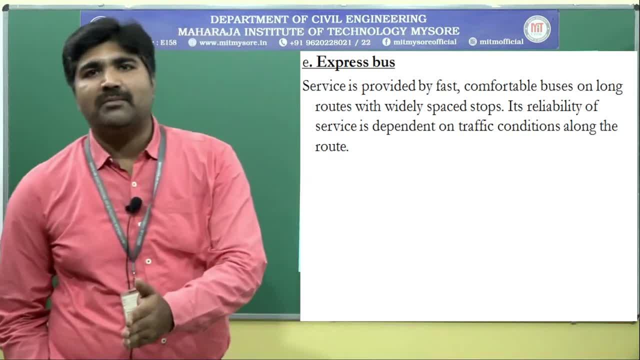 from majestic to airport. they travel from majestic to airport. they travel faster, at a faster rate, and also the stoppages will be faster, at a faster rate, and also the stoppages will be faster, at a faster rate, and also the stoppages will be minimum from majestic to airport. okay, there is. 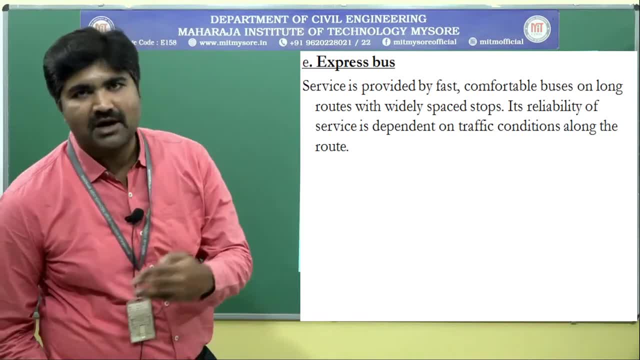 minimum from majestic to airport. okay, there is minimum from majestic to airport. okay, there is around 20 plus kilometer. is there? nearly around 30? around 20 plus kilometer? is there? nearly around 30? around 20 plus kilometer? is there? nearly around 30 kilometer is there. but stoppages will be very. 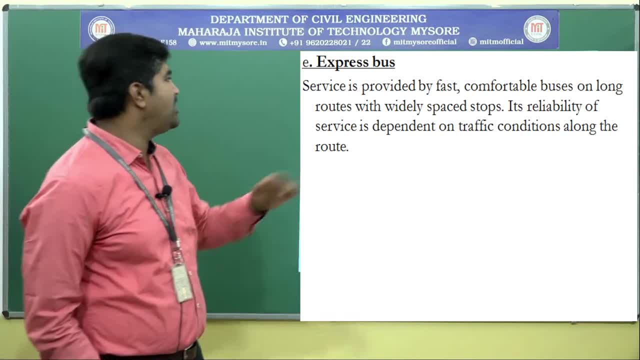 kilometer is there but stoppages will be very kilometer is there but stoppages will be very less frequently will stop model but less frequently will stop model but less frequently will stop model. but activity and its reliability of service activity and its reliability of service activity and its reliability of service is dependent on the traffic condition. 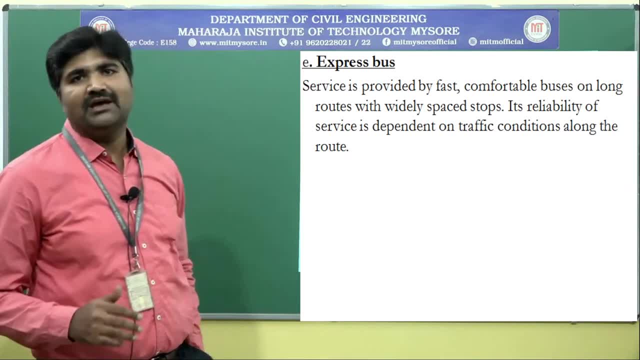 is dependent on the traffic condition, is dependent on the traffic condition. okay. reliability that depends upon the okay. reliability that depends upon the okay. reliability that depends upon the traffic condition: okay if congestion is traffic condition. okay if congestion is traffic condition. okay if congestion is not there, it will travel fast at the 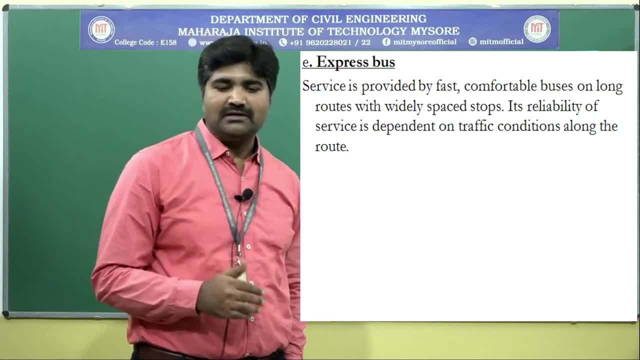 not there, it will travel fast at the not there, it will travel fast at the time. we can reliable on that, we can time. we can reliable on that, we can time. we can reliable on that. we can depend upon that. okay, next semi rapid. depend upon that. okay, next semi rapid. 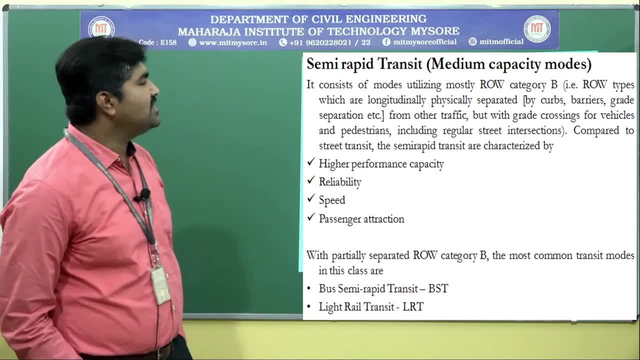 depend upon that. okay, next, semi rapid transit system. okay, this mode utilize transit system. okay, this mode utilize transit system. okay, this mode utilize mostly right-of-way category B, as we mostly right-of-way category B, as we mostly right-of-way category B, as we know, right-of-way category B and Reno. 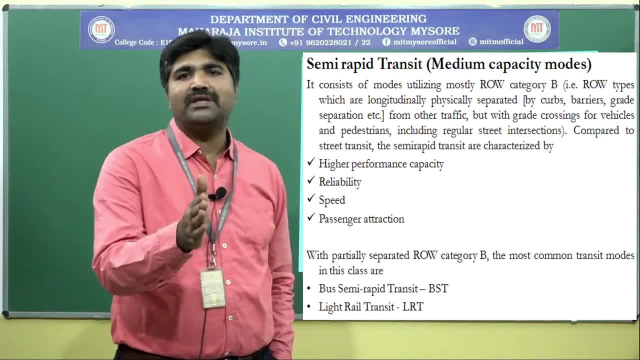 know right-of-way category B and Reno know right-of-way category B and Reno this: there, the mass transit will be this. there, the mass transit will be this. there, the mass transit will be separated from the general traffic. okay, separated from the general traffic. okay, separated from the general traffic. okay, general traffic in the mass transit in a 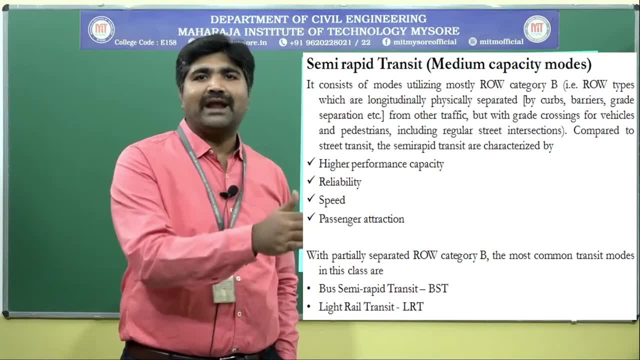 general traffic in the mass transit in a general traffic in the mass transit in a separate modality, by providing the separate modality, by providing the separate modality, by providing the separate line of a separate track, by separate line of a separate track, by separate line of a separate track, by providing the barriers of the inner. 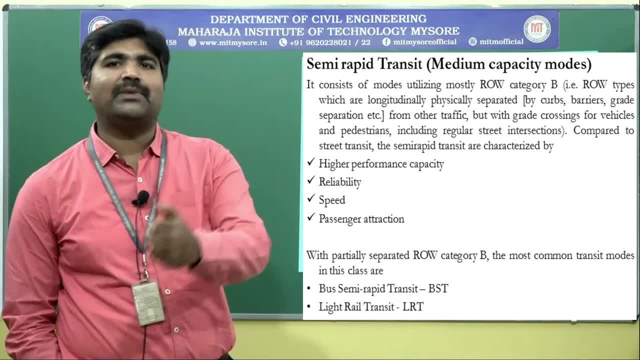 providing the barriers of the inner. providing the barriers of the inner curbs. okay, like medians of a great curbs. okay, like medians of a great curbs. okay, like medians of a great separation. provide money, separate track separation. provide money, separate track separation. provide money, separate track- at was a plate line. provide modality for. 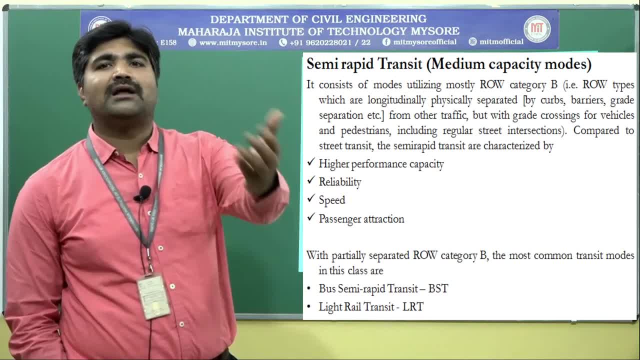 at was a plate line. provide modality for at was a plate line. provide modality for mass transit that may be for bus skir. mass transit that may be for bus skir. mass transit that may be for bus skir. Bodo atwa. light rail transit- light rail. 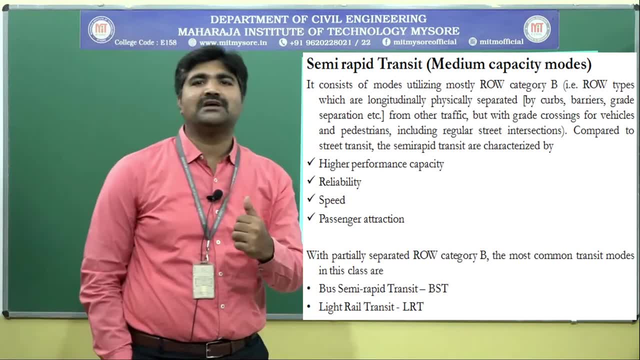 Bodo atwa light rail transit- light rail. Bodo atwa light rail transit- light rail transit and rate tramps okay earlier in transit and rate tramps okay earlier in transit and rate tramps okay earlier in. from British times also, we are using. from British times also, we are using. 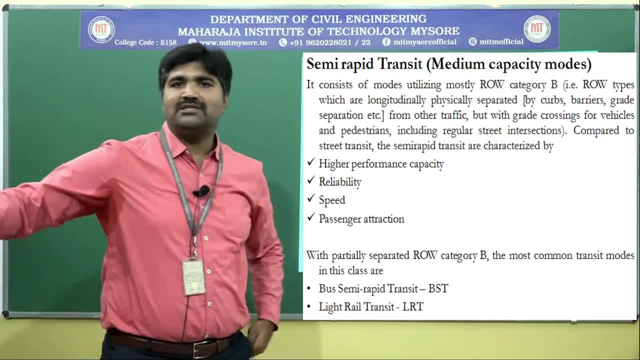 from British times also. we are using tramps in India that may be in Calcutta, tramps in India that may be in Calcutta, tramps in India that may be in Calcutta, tramps and a normal general road level. tramps and a normal general road level. 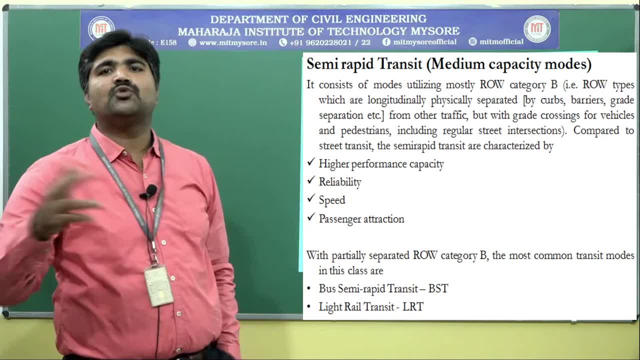 tramps and a normal general road level. road alert racks here today, Elena Chico. road alert racks here today, Elena Chico. road alert racks here today, Elena Chico, trying smaller trains with two or four. trying smaller trains with two or four. trying smaller trains with two or four wagons, with two or four cars. okay, bogies. 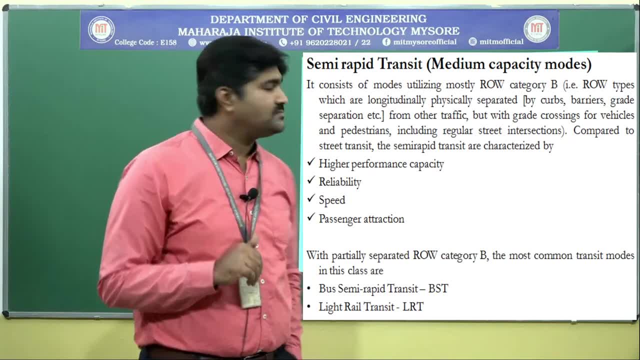 wagons with two or four cars: okay, bogies. wagons with two or four cars: okay, bogies, what are third of it? okay, that are the what are third of it. okay, that are the what are third of it. okay, that are the tramps. okay, see this. have higher. 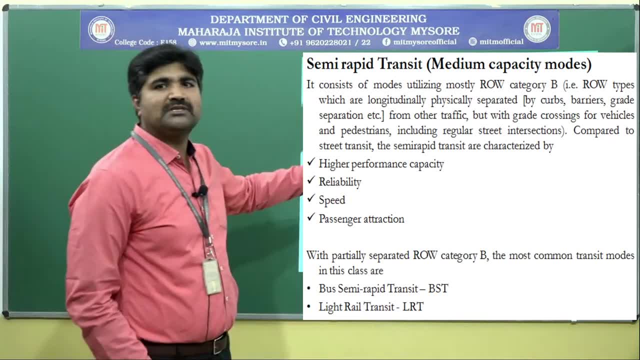 tramps. okay, see this, have higher tramps. okay, see this. have higher performance than the street transit. okay, performance than the street transit. okay, performance than the street transit. okay, this has a year performance. this mass, this has a year performance. this mass, this has a year performance. this mass transit, this semi-rapid transit, has some. 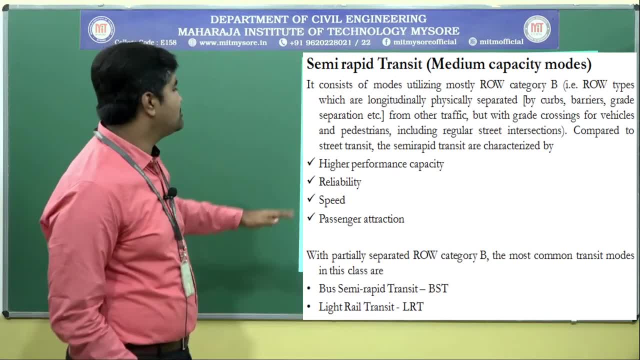 transit. this semi-rapid transit has some transit. this semi-rapid transit has some advantages on the street transit. which advantages on the street transit? which advantages on the street transit? which are that advantages? okay, it has a year. are that advantages? okay, it has a year. are that advantages? okay, it has a year performance capacity. okay, due to. 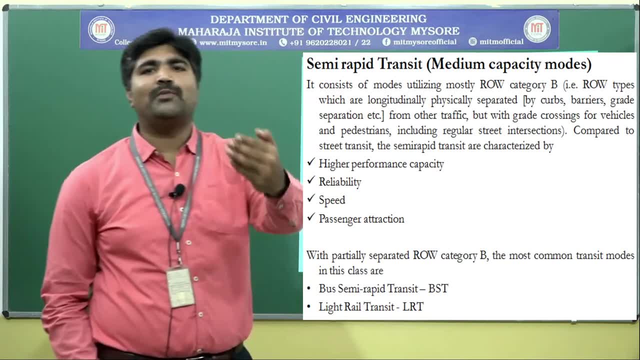 performance capacity. okay, due to performance capacity. okay due to separate track: separate track. provide separate track. separate track. provide separate track. separate track. provide medicine in the NAC today, faster medicine in the NAC today. faster medicine in the NAC today. faster movement will be there. there will be no. 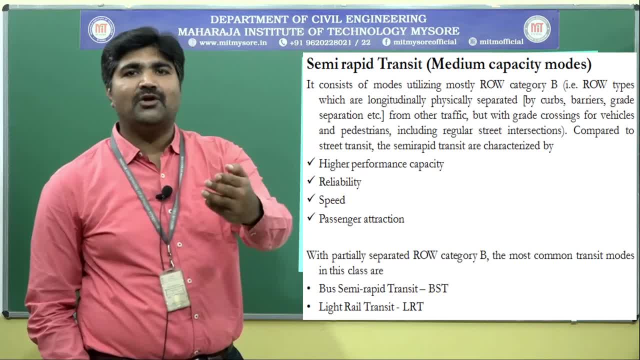 movement will be there. there will be no movement will be there. there will be no congestion. okay, there will be no congestion. okay, there will be no congestion. okay, there will be no disturbances to the movement. okay, so, the disturbances to the movement, okay. so the disturbances to the movement, okay. so the performance will be higher, the capacity. 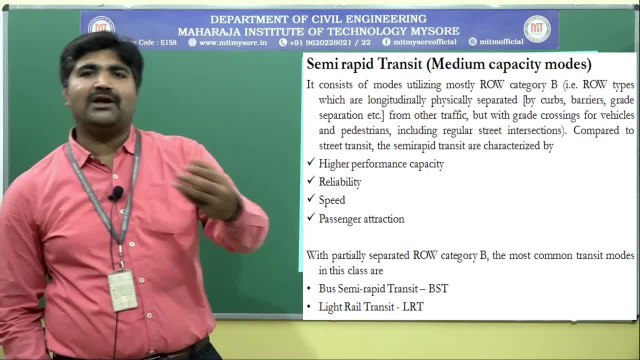 performance will be higher. the capacity performance will be higher. the capacity increases. next, reliability: we can increases. next reliability we can increases. next reliability: we can reliable on that. depend on that. okay. the reliable on that depend on that. okay. the reliable on that depend on that. okay. the time taken will be less. okay. the 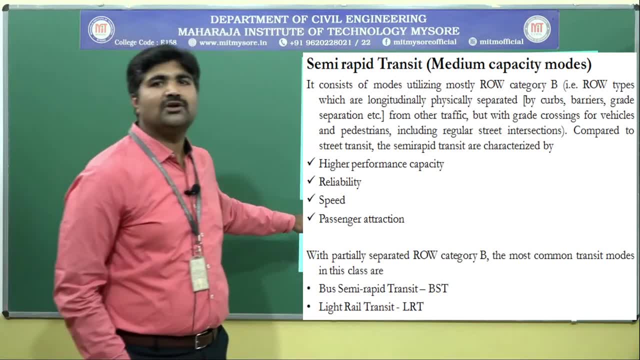 time taken will be less okay. the time taken will be less okay. the passengers will reliable on that. okay, passengers will reliable on that. okay, passengers will reliable on that. okay, next speed, as I told there will be a next speed. as I told there will be a next speed. as I told there will be a separate track. okay, only the buses, only. 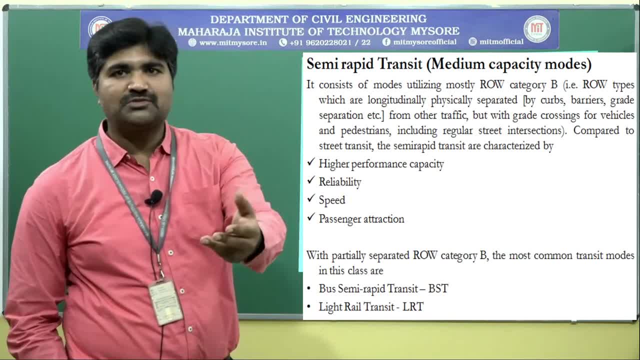 separate track. okay, only the buses, only separate track. okay, only the buses, only the trams will move on that track. so the trams will move on that track. so the trams will move on that track. so there will be more speed, okay, and this. there will be more speed, okay, and this. 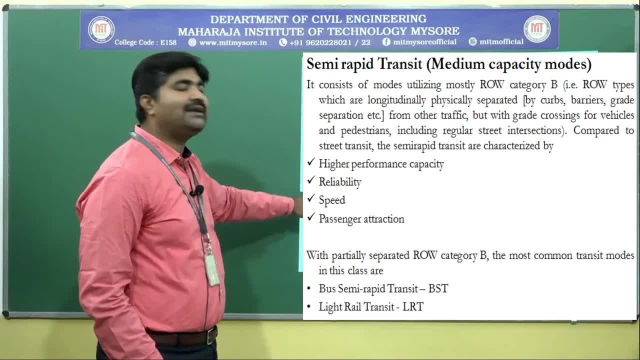 there will be more speed. okay, and this three, this, whatever the this three, three this, whatever the this three, three this, whatever the this three characteristics are that that attracts. characteristics are that that attracts. characteristics are that that attracts the passenger. okay, as we provide the the passenger. okay, as we provide the. 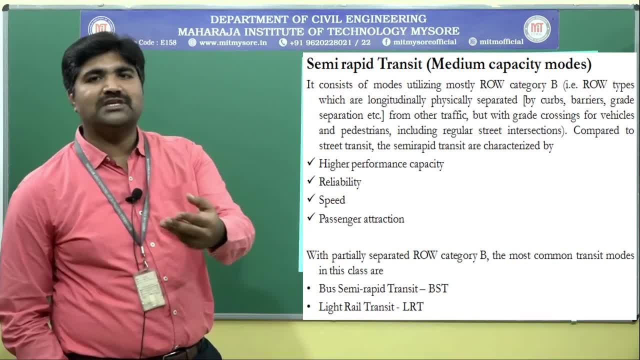 the passenger. okay, as we provide the high-performance. okay, faster rate, early high-performance. okay, faster rate, early high-performance. okay, faster rate early. would add to the time. save our Daga. would add to the time. save our Daga would add to the time. save our Daga atwa cost. save our the gain activity that. 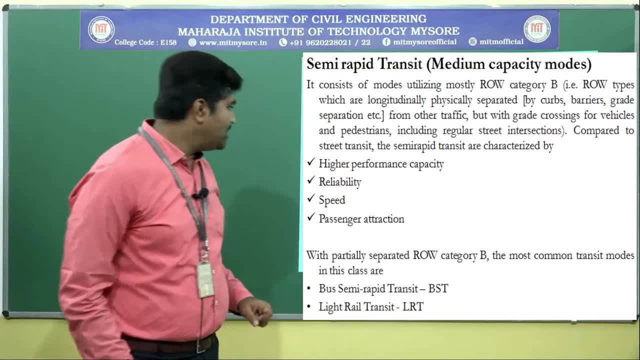 atwa cost. save our the gain activity. that atwa cost. save our the gain activity. that will attract automatically attracts the will attract automatically attracts the will attract automatically attracts the passengers. okay with partially separated passengers. okay with partially separated passengers. okay with partially separated. right-of-way category be the most common. 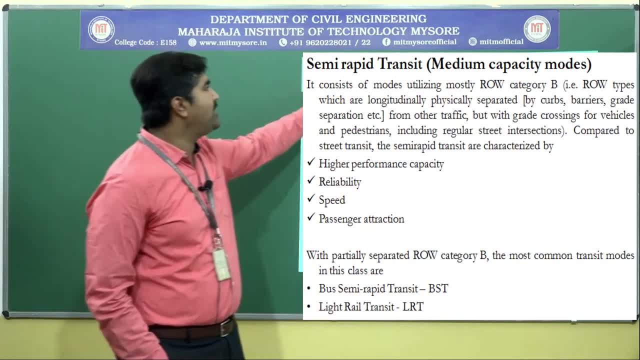 right-of-way category be the most common right-of-way category, be the most common transit modes in this class. okay, Israel, transit modes in this class. okay, Israel, transit modes in this class. okay, Israel, baron to the semi-rapid transistor. baron to the semi-rapid transistor. 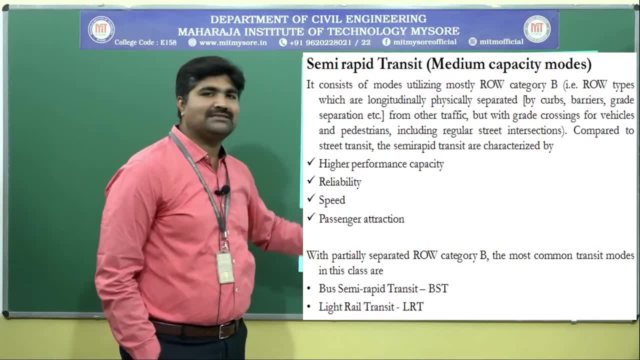 baron to the semi-rapid transistor. baron to the vehicle shadow that are the bus. baron to the vehicle shadow that are the bus. baron to the vehicle shadow that are the bus. semi-rapid transit- okay, bus rapid. semi-rapid transit- okay, bus rapid. 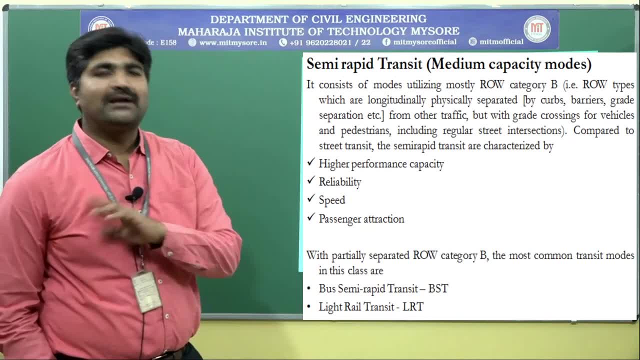 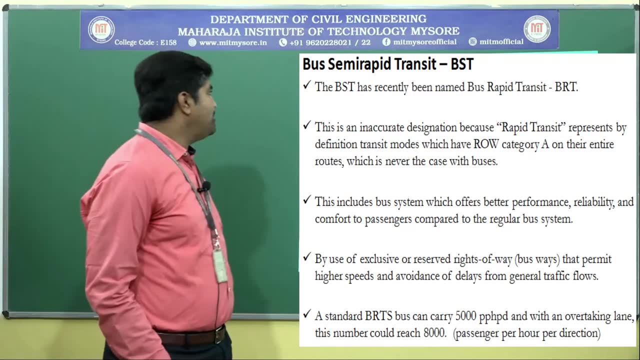 semi-rapid transit: okay. bus rapid transit system at the altar. okay. light transit system at the altar: okay, light transit system at the altar. okay, light rail transit system: okay. bus semi-rapid rail transit system: okay. bus semi-rapid rail transit system: okay. bus semi-rapid transit system: okay, the bus transit, the. 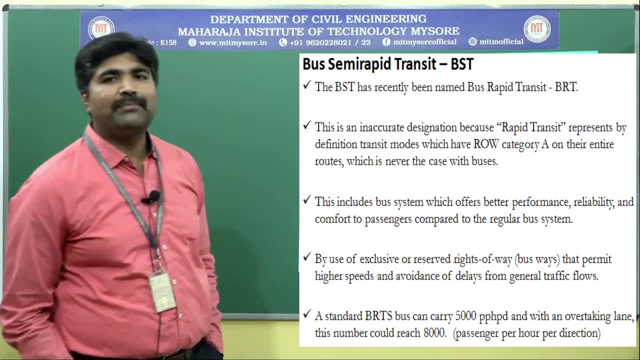 transit system: okay, the bus semi-rapid transit system. okay, the bus semi-rapid transit, as recently has been named bus transit. as recently has been named bus transit. as recently has been named bus rapid transit system. okay, this has been rapid transit system. okay, this has been. 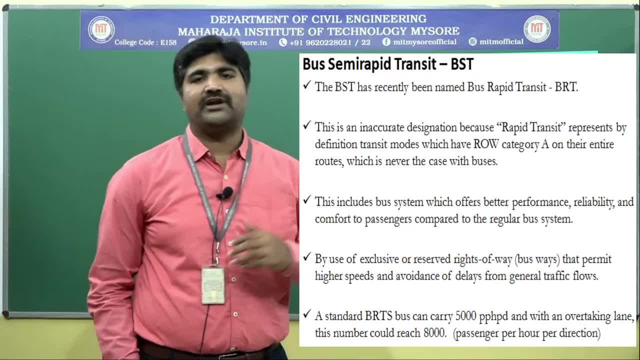 rapid transit system. okay, this has been recently provided in our state. that is recently provided in our state. that is recently provided in our state. that is simply ugly Darbar district for a simply ugly Darbar district, for a simply ugly Darbar district, for a distance of about 15 kilometer. okay, see, 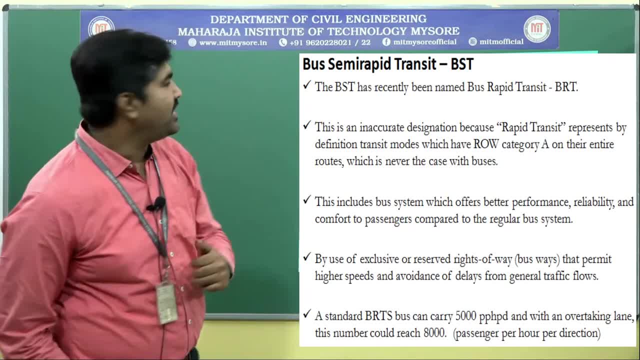 distance of about 15 kilometer. okay, see, distance of about 15 kilometer. okay, see, they have provided this separate track. they have provided this separate track. they have provided this separate track for the movement of the buses. okay, see, for the movement of the buses. okay, see. 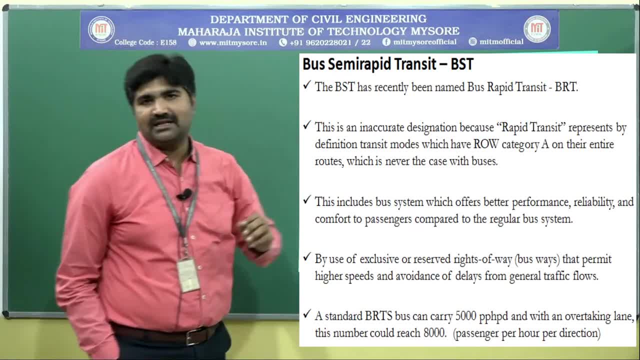 for the movement of the buses. okay, see, this is an inaccurate designation. okay, this is an inaccurate designation. okay, this is an inaccurate designation. okay, in our rapid transit. until the way that in our rapid transit, until the way that in our rapid transit, until the way that is the inaccurate designation, because the 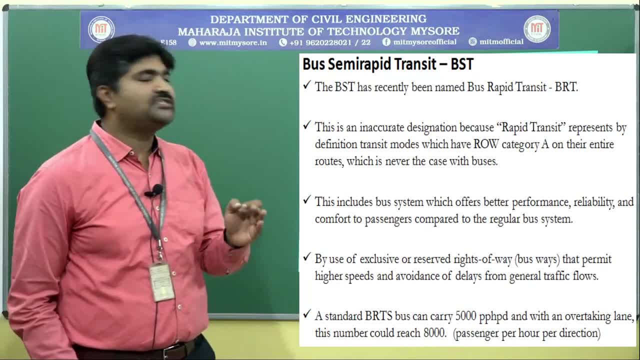 is the inaccurate designation because the is the inaccurate designation because the rapid transit represents, by definition, rapid transit represents by definition, rapid transit represents, by definition, transit modes which are right of a transit modes which are right of a transit modes which are right of a category, a okay right of a category, Lee. and. 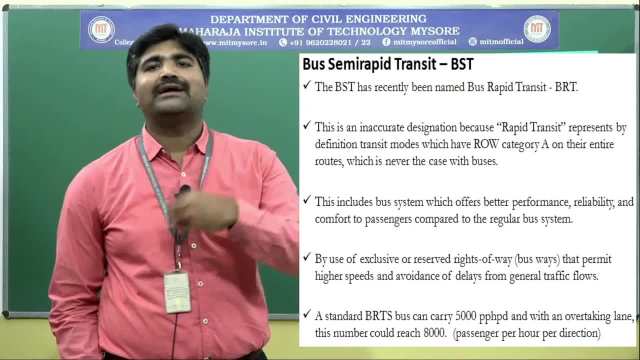 category a: okay, right of a category: Lee. and category a- okay, right of a category: Lee. and the bar on the vehicle. so that may be the bar on the vehicle. so that may be the bar on the vehicle. so that may be metro, monorail. okay, they are travel at a. 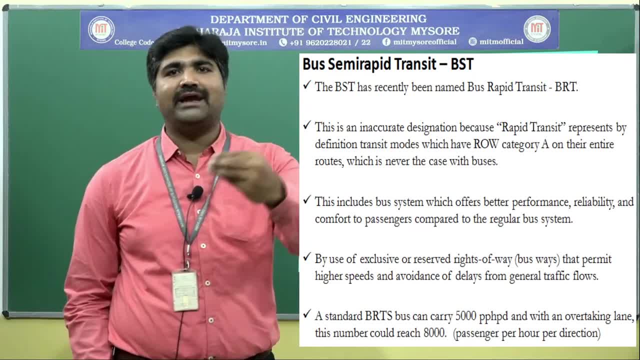 metro monorail. okay, they are travel at a metro monorail. okay, they are travel at a faster rate. Alva- right of a category- faster rate. Alva- right of a category- faster rate. Alva right of a category- liberal on the door. I a category- liberal. 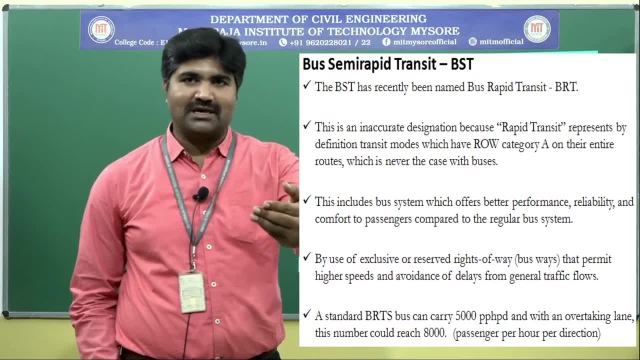 liberal on the door. I a category liberal, liberal on the door. I a category liberal on the vehicle. you know faster it okay on the vehicle. you know faster it okay on the vehicle. you know faster it okay, faster readily move up to them, but that, faster readily move up to them, but that. 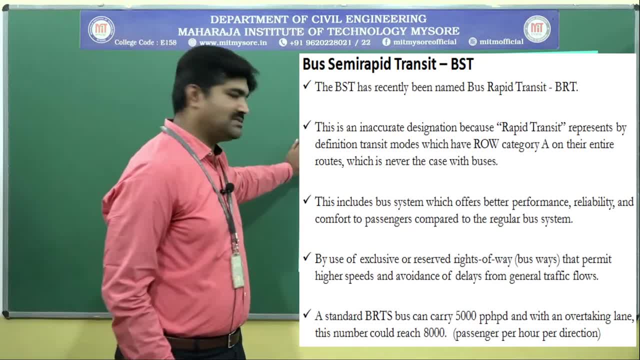 faster, readily move up to them. but that is not exactly at one. never true. in is not exactly at one. never true in is not exactly at one. never true in cases of buses: okay. next, this includes cases of buses. okay next, this includes cases of buses. okay next, this includes bus system which offers better. 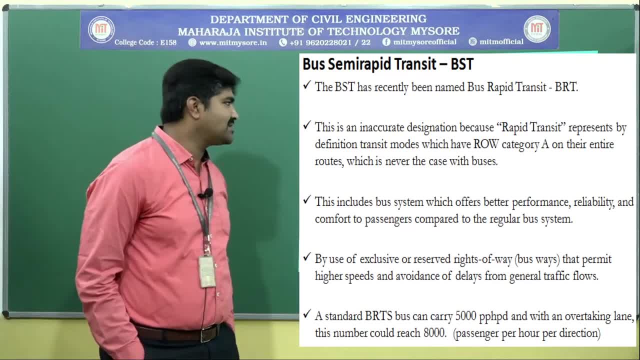 bus system which offers better bus system which offers better performance, reliability and comfort to performance, reliability and comfort. to performance, reliability and comfort to passengers. compared to regular bus passengers. compared to regular bus passengers. compared to regular bus system. see the regular buses. that travels system. see the regular buses. that travels. 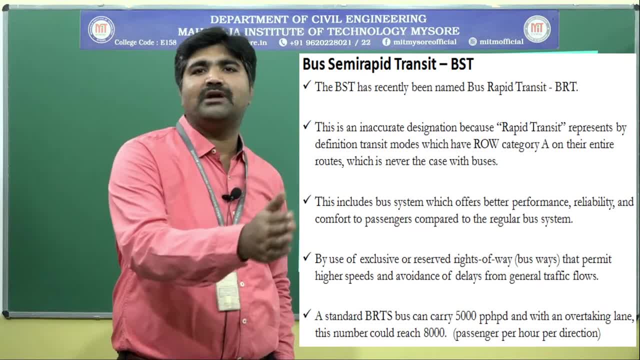 system. see the regular buses that travels with the mixed traffic here. there will, with the mixed traffic here. there will, with the mixed traffic here there will be a separate track for the movement of be a separate track for the movement of be a separate track for the movement of the buses, so it provides by a high 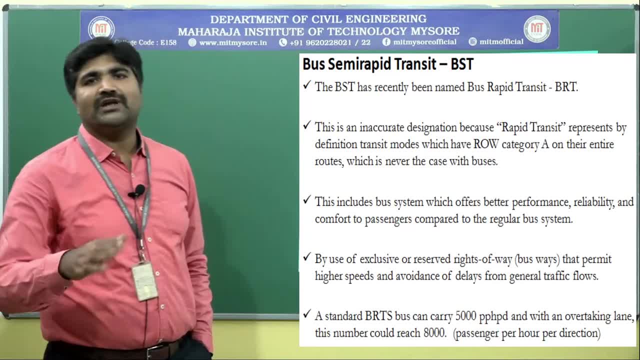 the buses, so it provides by a high the buses, so it provides by a high performance, reliability and comfort to performance. reliability and comfort to performance. reliability and comfort to passengers when compared to regular bus passengers, when compared to regular bus passengers when compared to regular bus. okay, by use of exclusive or reserved. 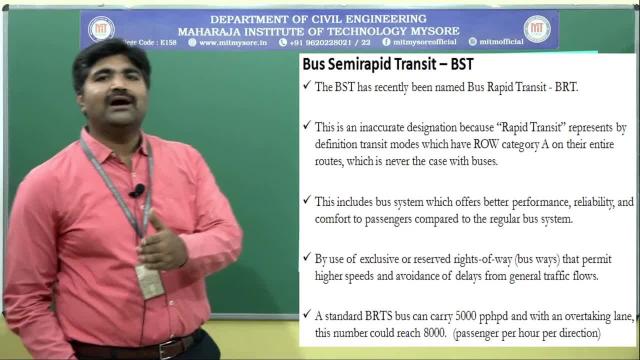 okay by use of exclusive or reserved. okay by use of exclusive or reserved right-of-way that permits IR space, as I. right-of-way that permits IR space, as I right-of-way that permits IR space. as I told, there will be a reserved right-of-way. told there will be a reserved right-of-way. 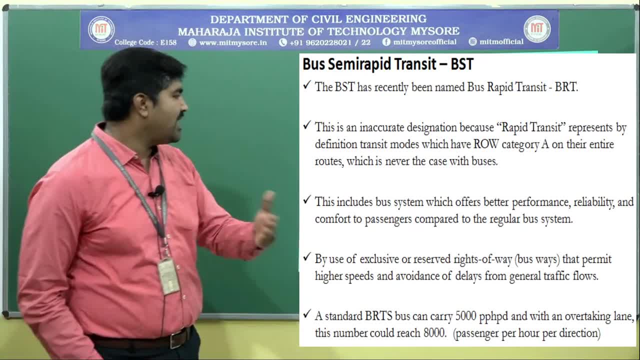 told there will be a reserved. right-of-way reserved track will be there, okay. reserved track will be there, okay. reserved track will be there, okay. that permits the IR speed and avoids the. that permits the IR speed and avoids the. that permits the IR speed and avoids the delays from the general traffic there. 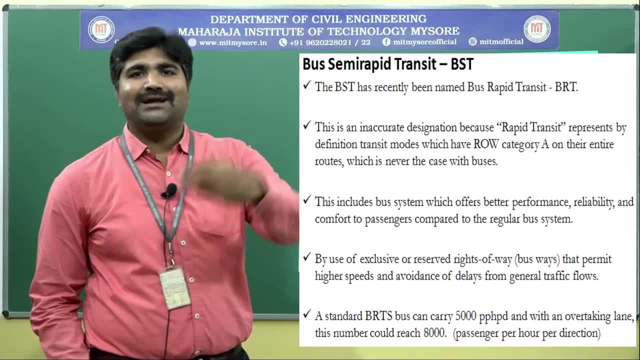 delays from the general traffic there. delays from the general traffic, there will be no access to general traffic. so will be no access to general traffic. so will be no access to general traffic. so it travels at high speed, okay, lastly a. it travels at high speed, okay, lastly a. 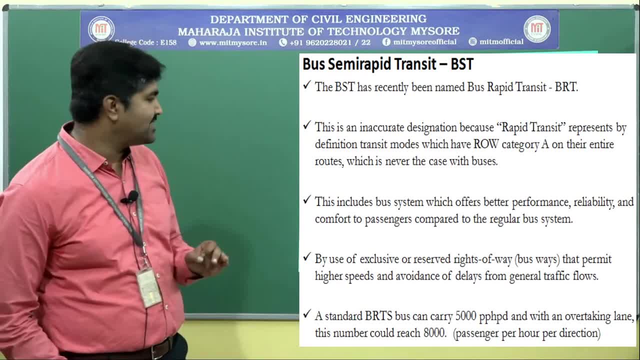 it travels at high speed okay. lastly, a standard BRTS bus: okay, bus transit standard: BRTS bus: okay, bus transit standard BRTS bus: okay, bus transit system. bus can carry 5,000 passenger per system bus can carry 5,000 passenger per. system bus can carry 5,000 passenger per hour per direction: okay. 5,000 passenger hour per direction: okay. 5,000 passenger hour per direction: okay, 5,000 passenger per hour per direction when we include. per hour per direction when we include. 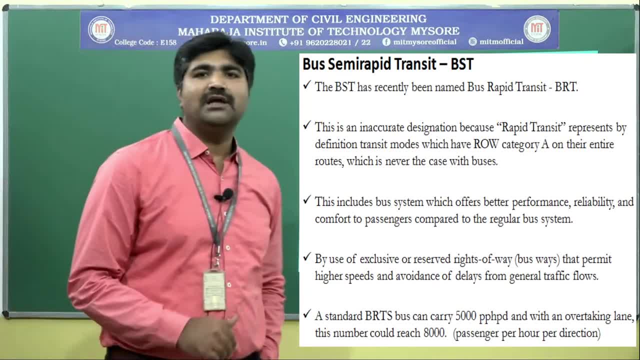 per hour per direction, when we include the overtaking line also. it can carry the overtaking line also. it can carry the overtaking line also. it can carry about of about 8,000 passengers. okay, about of about 8,000 passengers. okay, about of about 8,000 passengers. okay, 8,000 passenger per hour per direction. 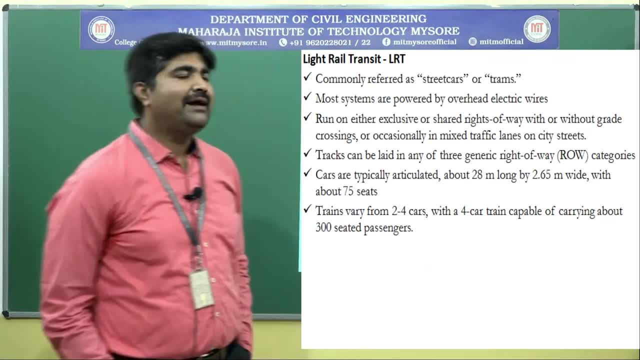 8,000 passenger per hour per direction. 8,000 passenger per hour per direction: okay. next light rail transit system: okay, okay. next light rail transit system, okay, okay. next light rail transit system: okay. commonly referred as streetcars at what? commonly referred as streetcars at what? 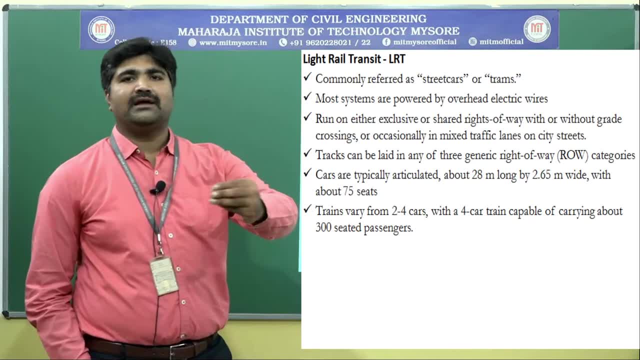 commonly referred as streetcars. at what tramps? okay tramps and the other, okay, tramps, okay tramps and the other, okay, tramps and the other, okay, tramps and the other, okay, that are operated early India, that are operated early India, that are operated early India, the little market operated, okay, you can. 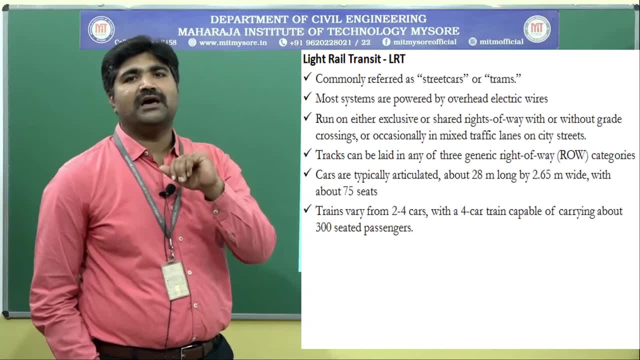 the little market operated okay. you can. the little market operated okay. you can see in the Kolkata at what channel, okay, see in the Kolkata at what channel, okay. see in the Kolkata at what channel, okay, from British times they are operating in. from British times they are operating in. 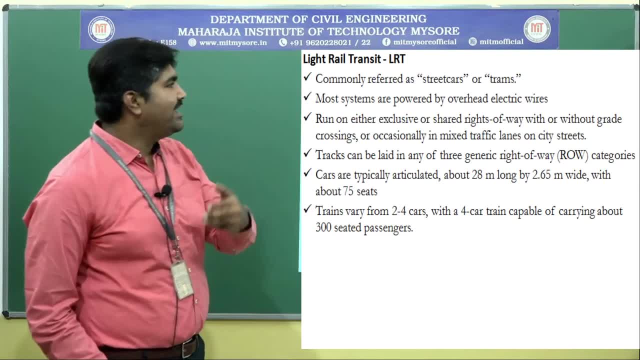 from British times. they are operating in India also. okay, see, the more systems are India also. okay, see, the more systems are India also. okay, see, the more systems are powered by overhead electric wires. okay, powered by overhead electric wires: okay. powered by overhead electric wires: okay, by using the electric traction they are. 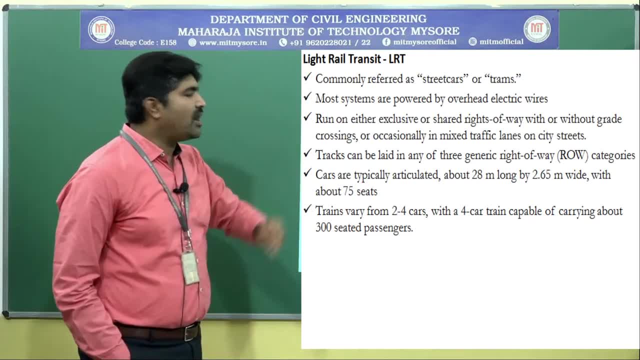 by using the electric traction. they are by using the electric traction. they are operated- okay. see, they run either on: operated- okay, see they run. either on operated- okay, see they run either on exclusive or shared right of way: okay, exclusive or shared right of way- okay. exclusive or shared right of way- okay, there may be great. separated, you go to. 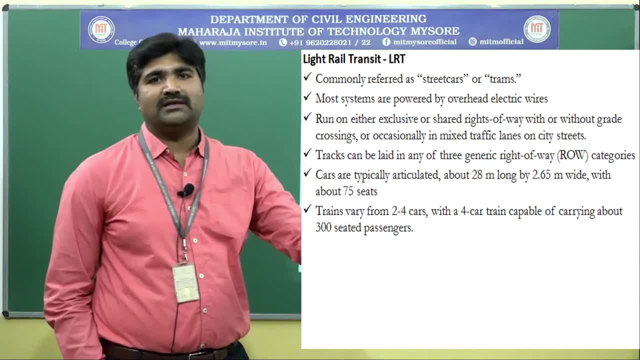 there may be great separated you go to. there may be great separated you go to Ottawa from general traffic in the Ottawa, from general traffic in the Ottawa from general traffic in the separate track. provide matter for that separate track. provide matter for that separate track. provide matter for that? yeah, and next tracks can be laid in any. 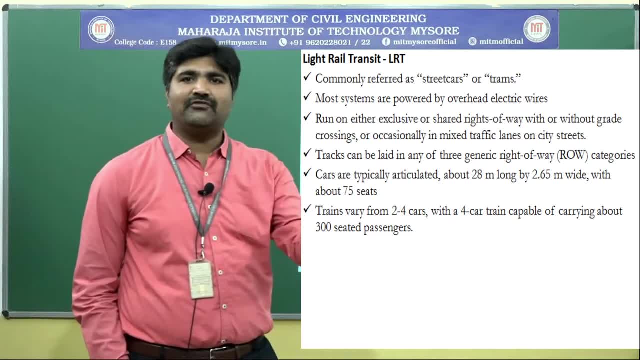 yeah and next tracks can be laid in any. yeah and next tracks can be laid in any. three generic right of a category. either three generic right of a category, either three generic right of a category. either it falls under the right of a category a. it falls under the right of a category a. 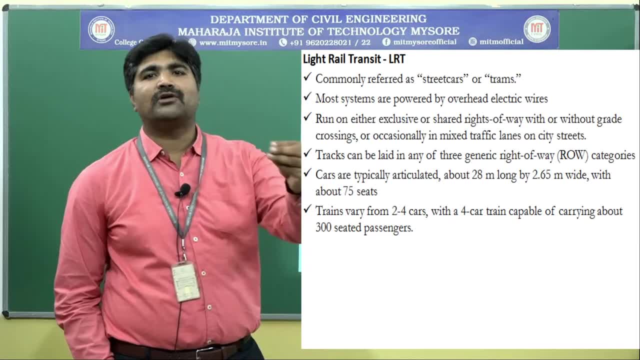 it falls under the right of a category a or a right of category B or a right of or a right of category B or a right of or a right of category B or a right of category C. morel L Baker track provide. category C- morel L Baker track provide. 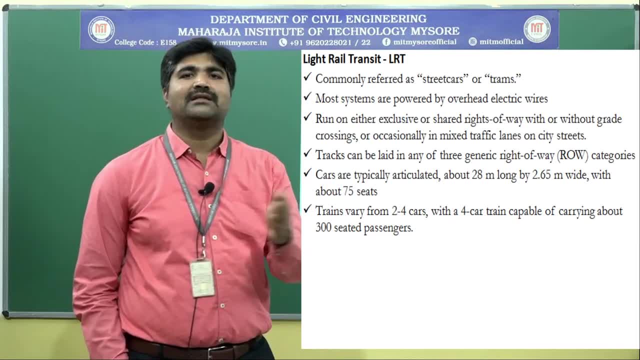 category C: morel L Baker track provide more Bodo but I keep the right of way. more Bodo, but I keep the right of way more Bodo, but I keep the right of way. category C: Leap and reenacted it there. category C: Leap and reenacted it there. 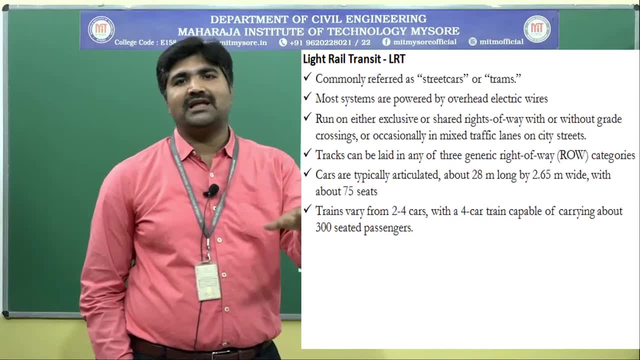 category C, Leap, and reenacted it there. that will be a separate track, but where that will be a separate track. but where that will be a separate track. but where that Junction L bertha, that okay traffic. that Junction L bertha, that okay traffic. that Junction L bertha, that okay traffic. cross our becker, there will be blockage. 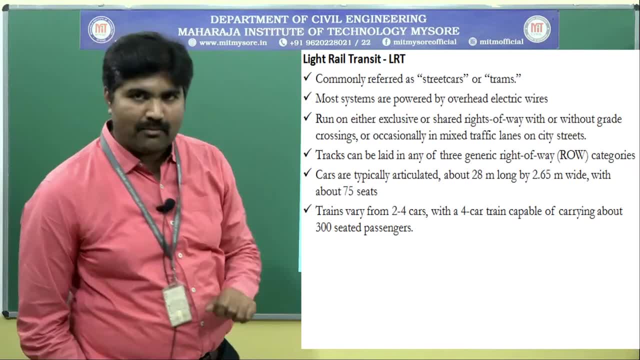 cross our becker, there will be blockage. cross our becker, there will be blockage of the other traffic. other mixed of the other traffic, other mixed of the other traffic, other mixed traffic in Bertha that will be blocked. traffic in Bertha that will be blocked. 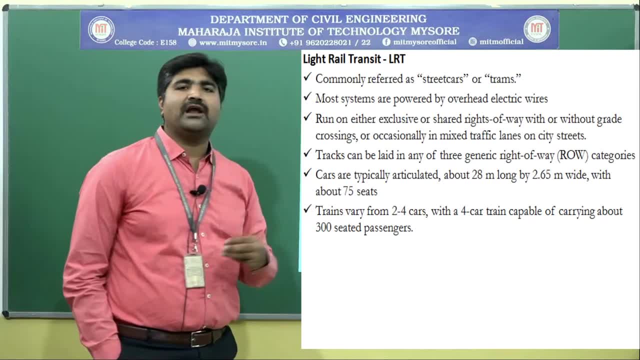 traffic in Bertha that will be blocked, okay. next see, the cars are typically okay. next see, the cars are typically okay. next see, the cars are typically articulated. articulated means they are articulated, articulated means they are articulated. articulated means they are customized. okay about the to the cars. 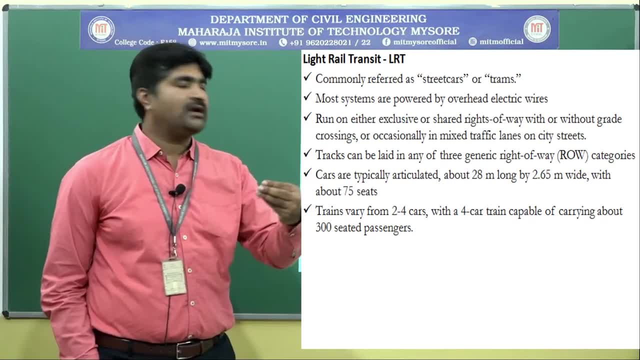 customized okay about the to the cars. customized okay about the to the cars means the wagons at the bogies. okay, it means the wagons at the bogies. okay, it means the wagons at the bogies. okay, it has a length of two point, sorry, 28 meter. 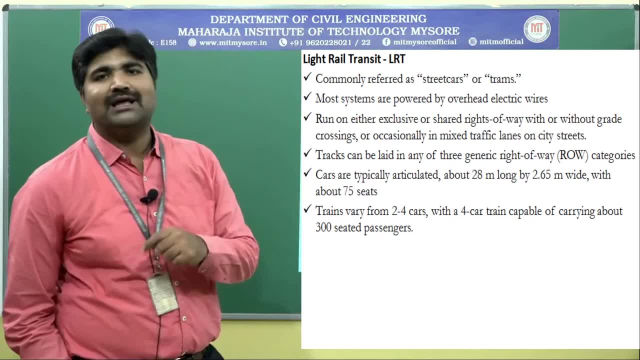 has a length of two point, sorry, 28 meter. has a length of two point, sorry, 28 meter long. okay, width of two point six five long. okay, width of two point six five long. okay, width of two point six five meter. okay, the length is 28 meter and. 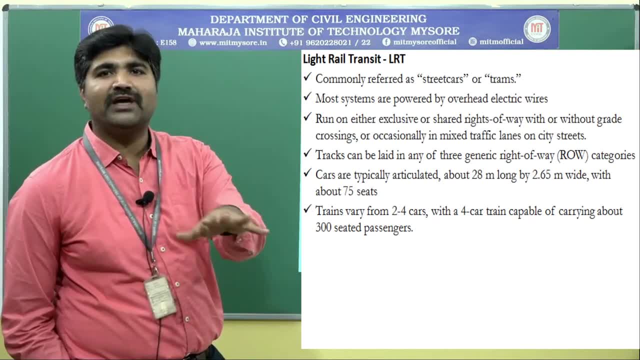 meter. okay, the length is 28 meter and meter. okay, the length is 28 meter and the width is two point six five meter. the width is two point six five meter. the width is two point six five meter. okay, this is the dimension of the. okay, this is the dimension of the. 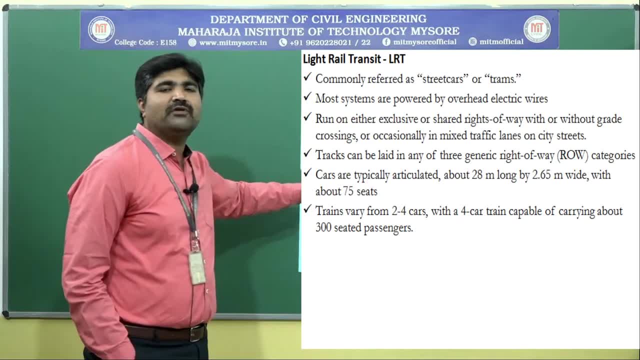 okay, this is the dimension of the wagons. are bogies? okay with about seating? wagons are bogies- okay with about seating. wagons are bogies. okay with about seating capacity of about 75 seats. there will be capacity of about 75 seats there will be. 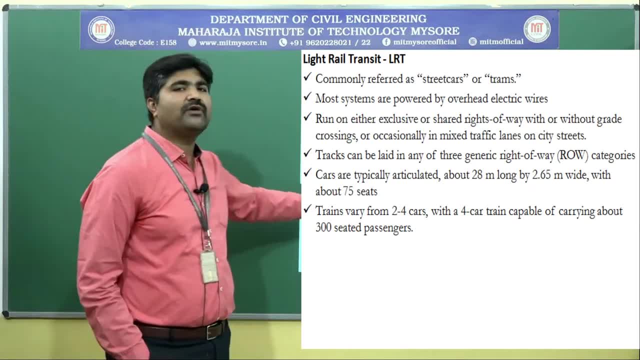 capacity of about 75 seats. there will be a seating capacity of 75 seats. okay, the a seating capacity of 75 seats. okay, the a seating capacity of 75 seats. okay. the trains vary from two to four cars. okay, trains vary from two to four cars. okay. 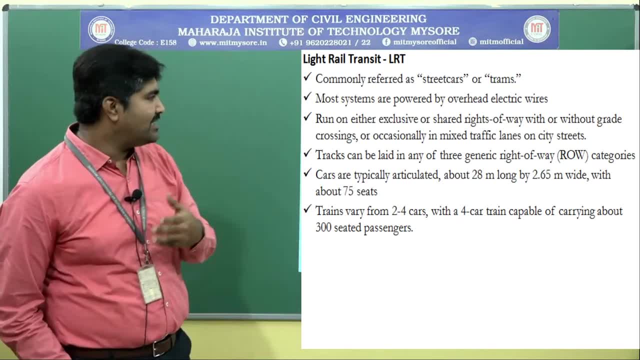 trains vary from two to four cars. okay, here the trams. okay, they carry two. to here the trams. okay, they carry two. to here the trams. okay, they carry two. to four trains. okay, the tram with a four car, four trains. okay, the tram with a four car. okay, that capable of carrying about 300. 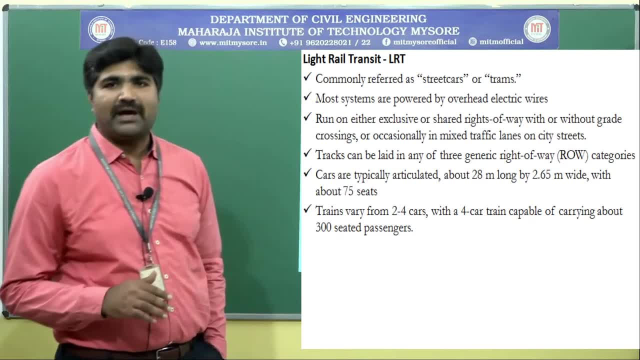 okay that capable of carrying about 300. okay that capable of carrying about 300 seated passengers. okay at a time. it can seated passengers. okay at a time. it can seated passengers. okay at a time. it can take about 300 passengers. okay next. take about 300 passengers, okay next. 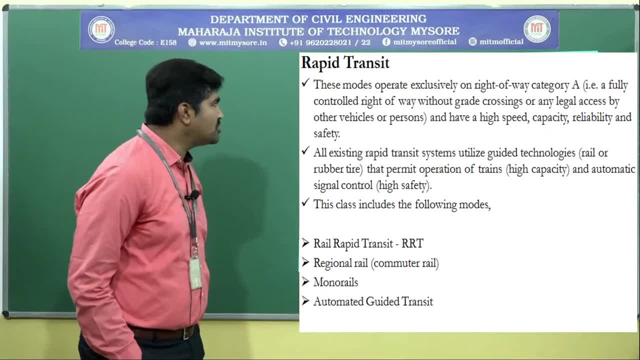 take about 300 passengers. okay, next, rapid transit. see this: modes operate rapid transit. see this: modes operate rapid transit. see this: modes operate exclusively on right of a category, as we, exclusively on right of a category, as we exclusively on right of a category, as we know. right of category. yeah, that is the. 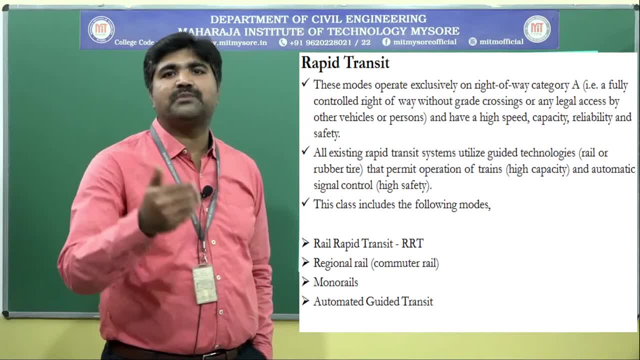 know right of category. yeah, that is the know right of category. yeah, that is the exclusive system. okay, atwa freeway and exclusive system. okay, atwa freeway and exclusive system. okay, atwa freeway and security atway expressway. there will be. security atway expressway, there will be. 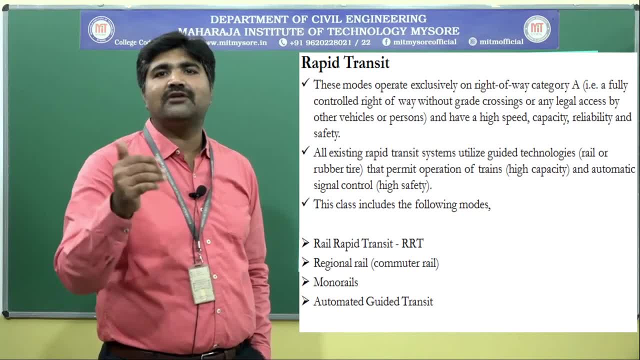 security atway expressway. there will be no disturbances, okay. there will be no, no disturbances, okay. there will be no, no disturbances, okay. there will be no legal access to any other vehicles. are legal access to any other vehicles? are legal access to any other vehicles? are persons. so here the vehicle will move at. 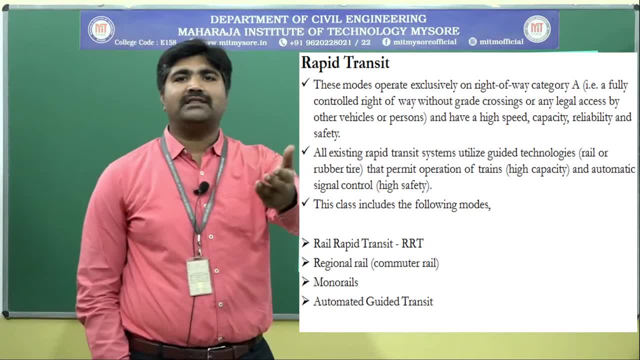 persons. so here the vehicle will move at persons. so here the vehicle will move at a faster rate. okay, there, that vehicle, a faster rate. okay, there, that vehicle, a faster rate. okay, there, that vehicle will move, either by using the tunnel at will move, either by using the tunnel at. 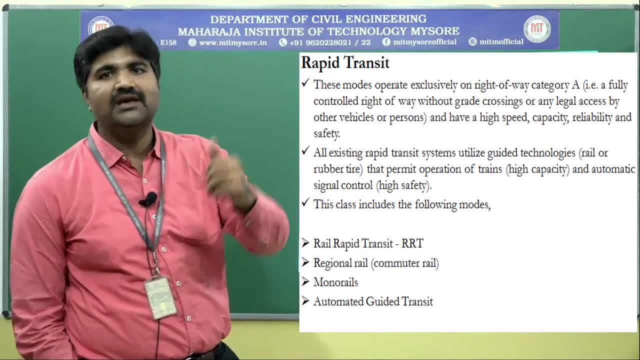 will move either by using the tunnel at. why aerial structures here real? why aerial structures here, real? why aerial structures here real? structures under that are the elevated structures. under that are the elevated structures. under that are the elevated structures that are the flyovers okay. structures that are the flyovers okay. 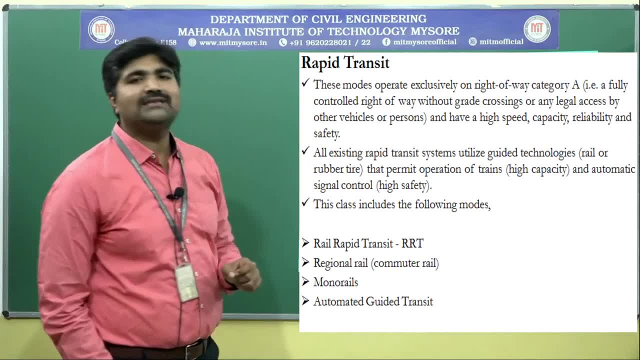 structures that are the flyovers. okay, see the all the existing rapid transit. see the all the existing rapid transit. see the all the existing rapid transit system. utilize the guided- okay, guided system. utilize the guided- okay guided system. utilize the guided- okay, guided technologies. guided technology means technologies. guided technology means. 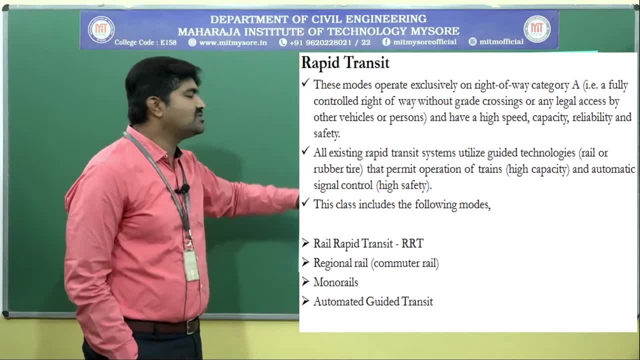 technologies. guided technology means automatic operation will be there, okay. automatic operation will be there, okay. automatic operation will be there, okay. next, this class includes the following: next, this class includes the following: next, this class includes the following modes: the following modes are the that modes: the following modes are the that: 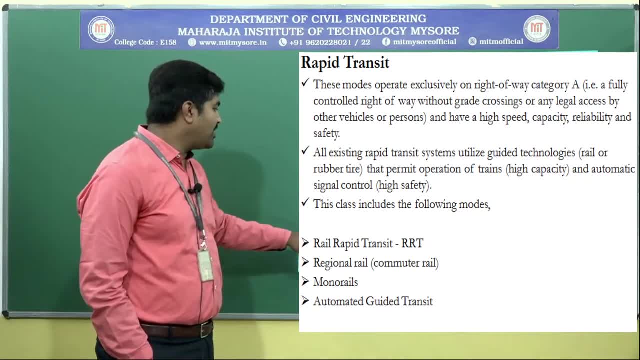 modes. the following modes are the that are the rail rapid transit: okay. are the rail rapid transit: okay. are the rail rapid transit: okay. regional rail: okay. monorail automated regional rail: okay. monorail automated regional rail: okay. monorail automated guide guided transit. see the rail rapid. 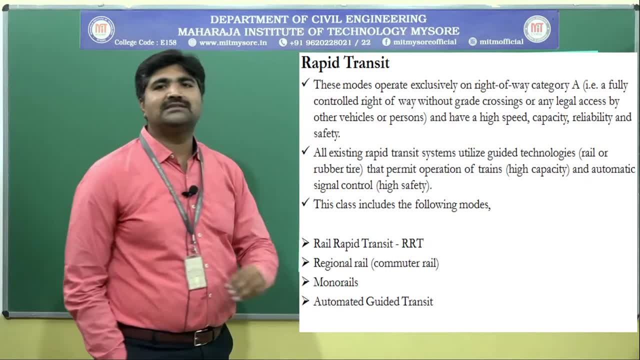 guide: guided transit. see the rail rapid guide: guided transit. see the rail rapid transit. that is the metro rail. okay, transit, that is the metro rail. okay, transit, that is the metro rail. okay, regional realm- is that is the suburban regional rail? is that is the suburban regional rail? is that is the suburban rail? okay, we know the monorail. okay, rapid. 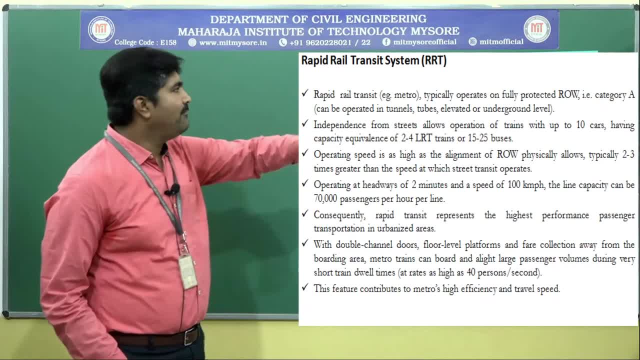 rail: okay, we know the monorail- okay. rapid rail: okay, rapid rail transit system. okay, rapid rail rail transit system. okay, rapid rail rail transit system. okay, rapid rail transit, as I told it is a metro, okay. transit, as I told it is a metro, okay. transit, as I told it is a metro, okay, typically operates on fully protected. 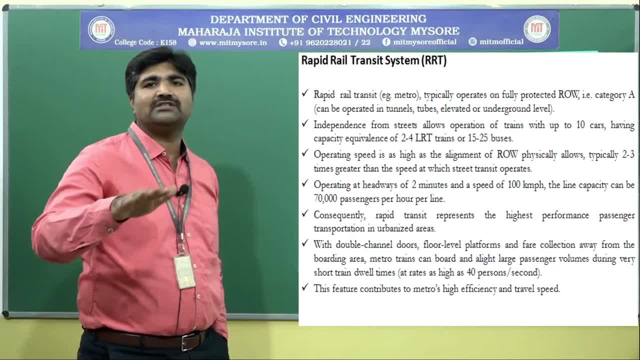 typically operates on fully protected. typically operates on: fully protected right-of-way- okay, fully protected right right-of-way- okay, fully protected right-of-way, although the right-of-way right-of-way, although the right-of-way right-of-way, although the right-of-way, which falls under category a, that is a. 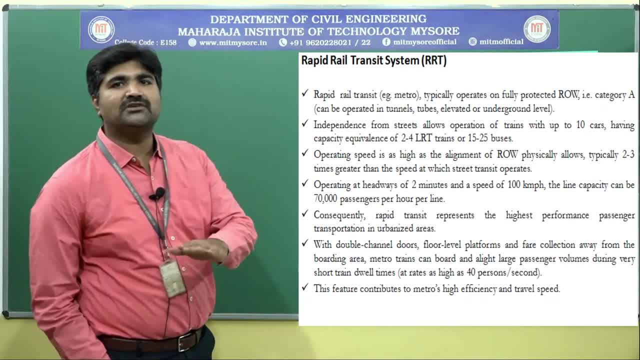 which falls under category a, that is a which falls under category a. that is a freeway- okay, exclusive way. there will be freeway. okay, exclusive way. there will be freeway. okay, exclusive way. there will be no disturbances of any other vehicles, of no disturbances of any other vehicles of. 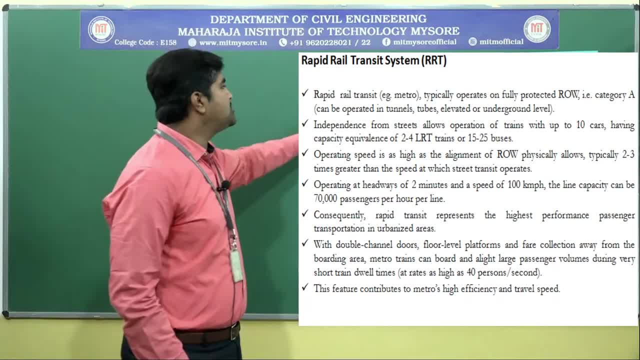 no disturbances of any other vehicles of the barren persons. they cannot enter the barren persons. they cannot enter the barren persons, they cannot enter. their independence from streets allows their independence from streets. allows their independence from streets. allows operation of trains with up to 10 cars. operation of trains with up to 10 cars. 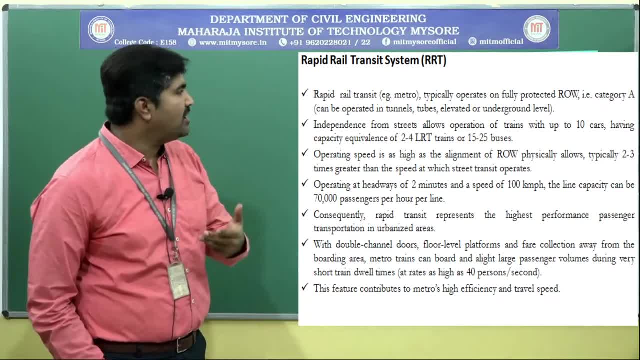 operation of trains with up to 10 cars having capacity equivalence to 2 to 4 LRT, having capacity equivalence to 2 to 4 LRT, having capacity equivalence to 2 to 4 LRT or 15 to 25 buses. okay, that is. 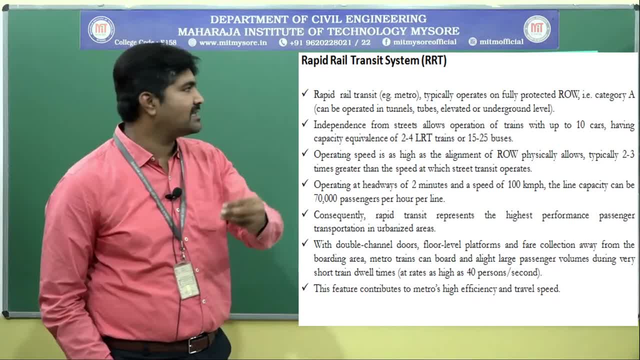 or 15 to 25 buses, okay, that is. or 15 to 25 buses, okay, that is. independent from the general traffic: okay, independent from the general traffic- okay, independent from the general traffic, okay. freeway system here, other in the freeway system here, other in the freeway system here, other in the energy there. they operate more than year near. 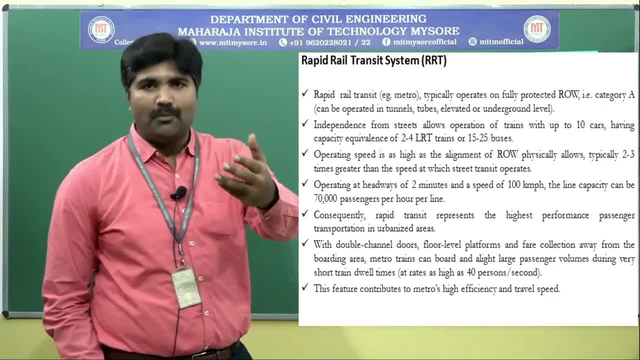 energy there they operate more than year. near energy there they operate more than year. near to 8 to 10 cars. 8 to 10 cars. miss. 8 to 8 to 10 cars. 8 to 10 cars miss. 8 to 8 to 10 cars. 8 to 10 cars miss. 8 to 10 bogies. okay, this increases the 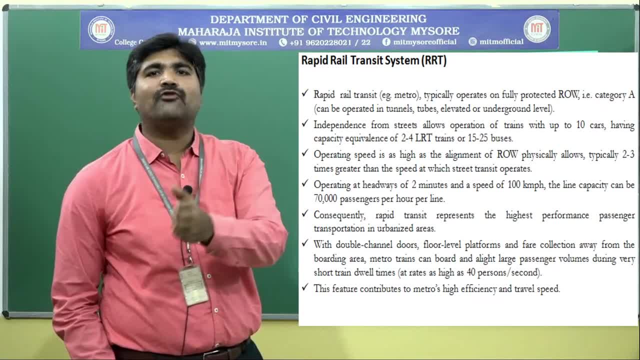 to 10 bogies. okay, this increases the to 10 bogies. okay, this increases the capacity when compared to okay. this will capacity when compared to okay. this will capacity when compared to okay. this will be equal to 2 to 4 LRT. 2 to 4 LRT. and. be equal to 2 to 4 LRT, 2 to 4 LRT and be equal to 2 to 4 LRT. 2 to 4 LRT and there 2 to 4 light rail transit. at what? there 2 to 4 light rail transit. at what? there 2 to 4 light rail transit. at what? 15 to 25 buses- okay, are the 15 to 25. 15 to 25 buses- okay are the 15 to 25. 15 to 25 buses- okay are the 15 to 25 buses- ain't carry Martha it okay at a. 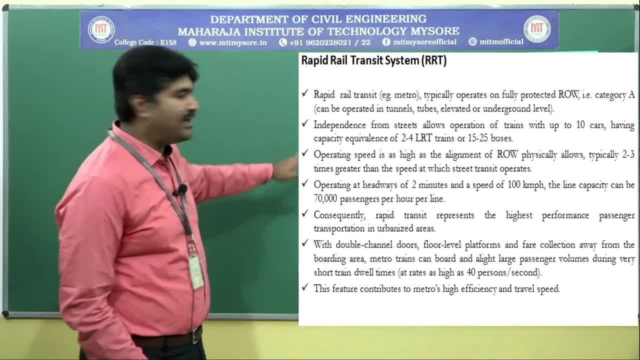 buses ain't carry Martha it okay at a buses ain't carry Martha it okay at a time. this will carry okay. that is the time this will carry okay. that is the time this will carry okay. that is the advantages of this Metro and also advantages of this Metro and also. 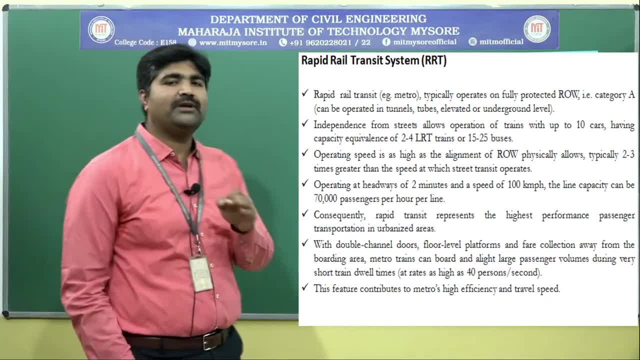 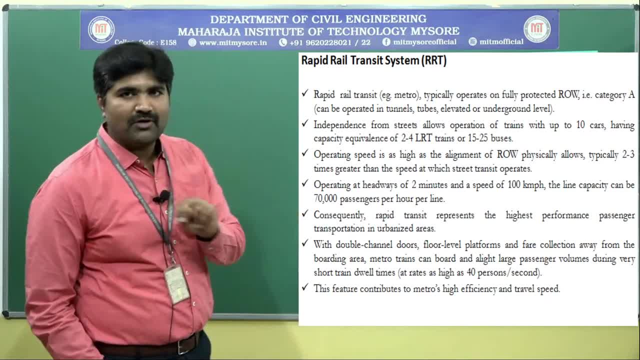 Reno, that is the frequency, that time. Reno, that is the frequency, that time. gap between the one train to next time, gap between the one train to next time, gap between the one train to next time: that is the 8-way gap. okay, that is two. that is the 8-way gap. okay, that is two. 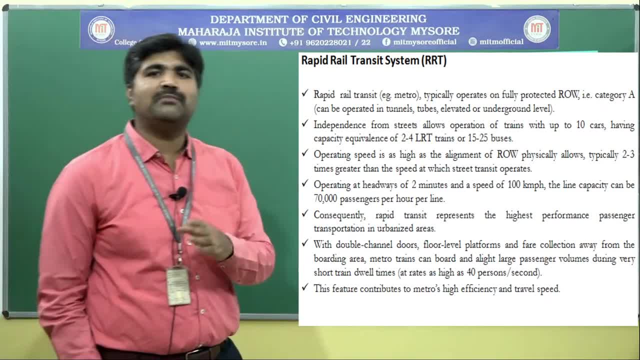 that is the 8-way gap. okay, that is two minutes and a speed of 100 kilometer per minutes. and a speed of 100 kilometer per minutes and a speed of 100 kilometer per hour- okay, this is not possible in case hour: okay, this is not possible in case. 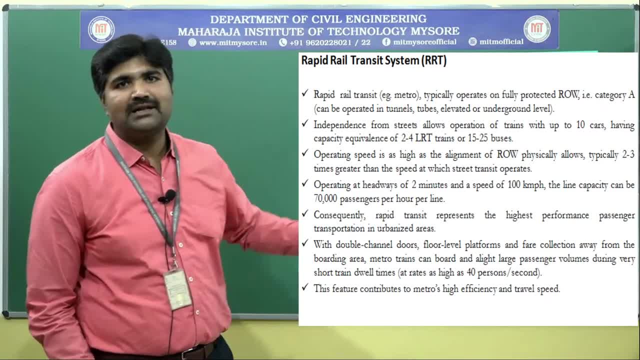 hour. okay, this is not possible in case of buses. all 100 kilometer per hour of buses, all 100 kilometer per hour of buses, all 100 kilometer per hour. rich ugly kagala, but that is possible in. rich ugly kagala, but that is possible in. 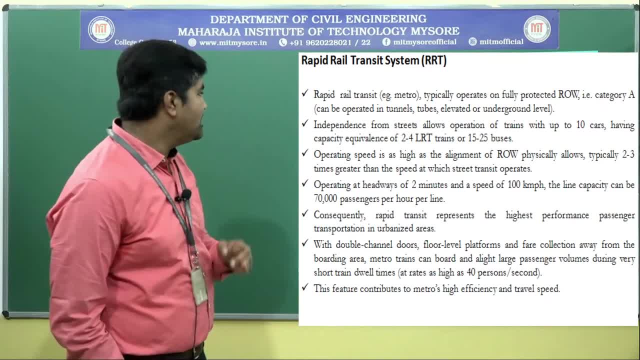 rich ugly kagala. but that is possible in case of Metro. okay, the line capacity can case of Metro. okay, the line capacity can case of Metro. okay, the line capacity can be 70,000 passenger per hour per line. be 70,000 passenger per hour per line. 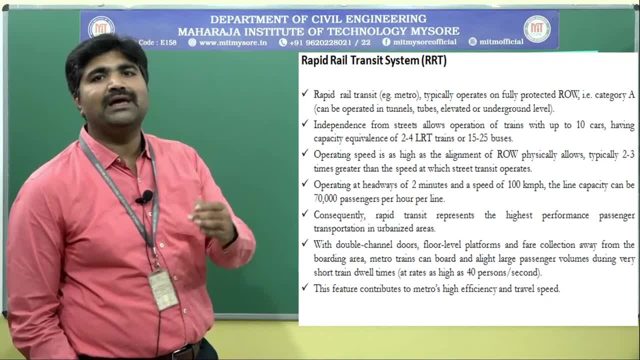 be 70,000 passenger per hour per line: okay. 70,000 person miss the passenger: okay. 70,000 person miss the passenger: okay, 70,000 person miss the passenger. can be carried per hour per length: okay, can be carried per hour per length, okay. 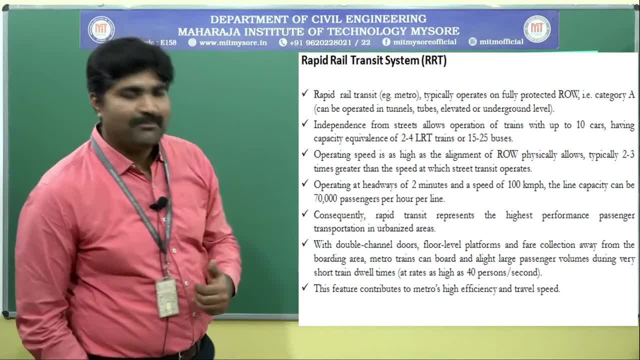 can be carried per hour per length. okay, if we consider the both the direction it. if we consider the both the direction it, if we consider the both the direction it: carries 1 lakh plus passengers per hour. carries 1 lakh plus passengers per hour. carries 1 lakh plus passengers per hour per length. okay, next, consequently rapid. 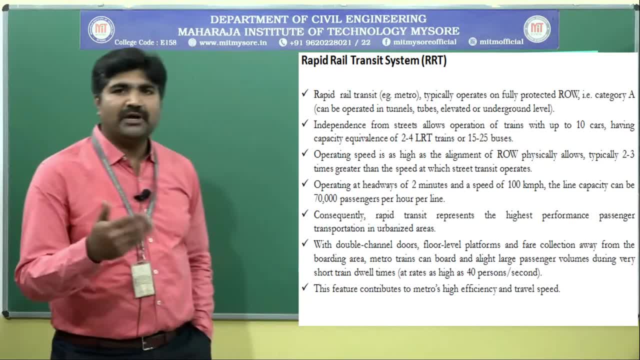 per length: okay next. consequently, rapid per length: okay next. consequently, rapid transit represents the highest transit, represents the highest transit, represents the highest performance. passenger transportation in performance. passenger transportation in performance. passenger transportation in urbanized areas: okay, we have studied now urbanized areas: okay, we have studied now. 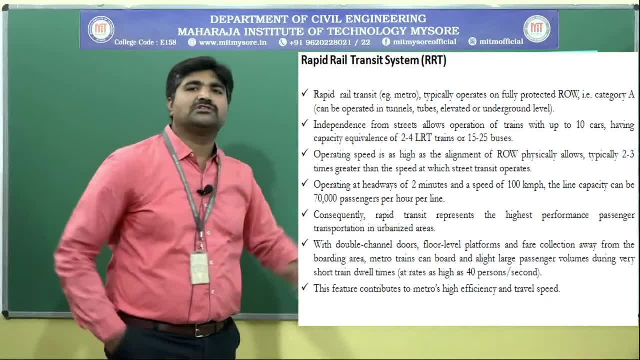 urbanized areas. okay, we have studied now. okay, when we consider the both the okay, when we consider the both the okay, when we consider the both the direction. okay, we double channel doors direction. okay, we double channel doors direction. okay, we double channel doors. okay, we have seen the Metro. Metro not 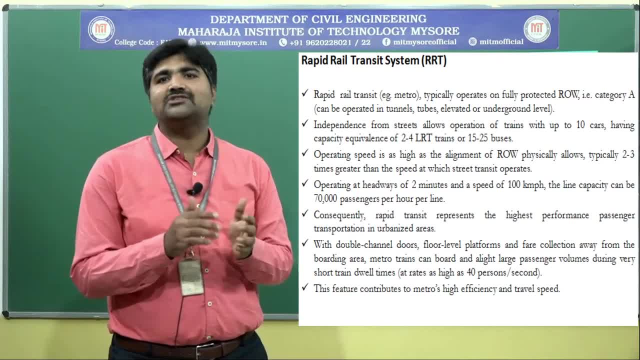 okay, we have seen the Metro Metro, not okay, we have seen the Metro Metro, not either. go doctor there, there will be either. go doctor there, there will be, either go doctor there, there will be. double channel doors: okay, this will easy. double channel doors: okay, this will easy. 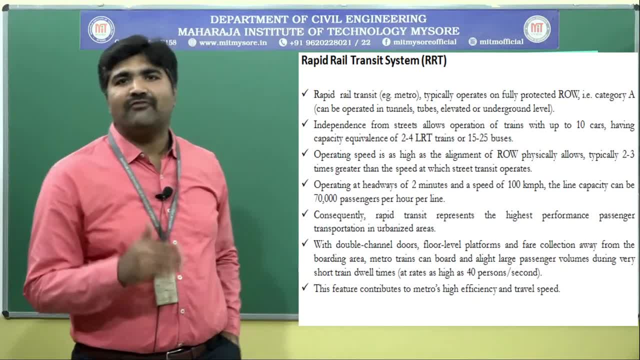 double channel doors. okay, this will easy for ease out the passenger to check in. for ease out the passenger to check in. for ease out the passenger to check in and check out very at a faster rate. okay, and check out very at a faster rate. okay, and check out very at a faster rate. okay, per second there may be 40 persons can. 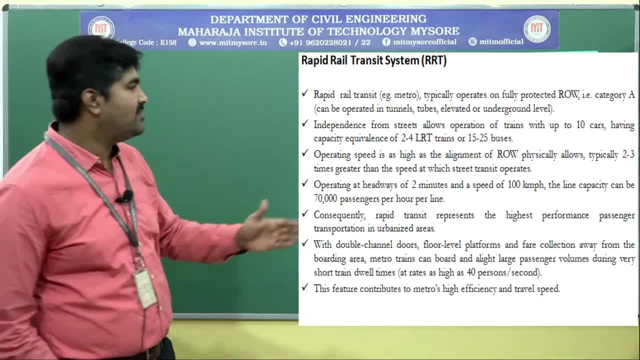 per second. there may be 40 persons can. per second there may be 40 persons can be check-in and check out. but like did be check-in and check out, but like did be check-in and check out, but like did, yeah, at a faster rate and there will be. 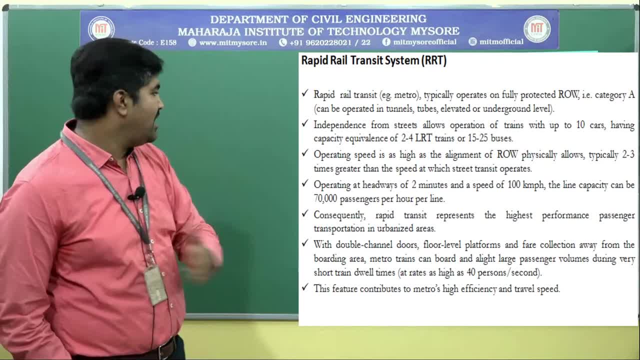 yeah, at a faster rate. and there will be- yeah, at a faster rate, and there will be separate. you know separate fare separate. you know separate fare separate. you know separate fare. collection room here today and also collection room here today and also collection room here today and also boarding area separated there. there will. 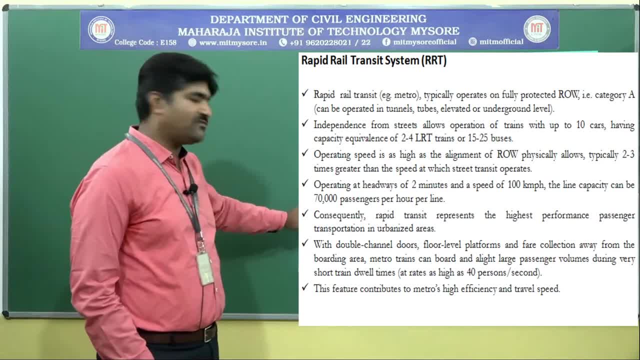 boarding area separated there. there will boarding area separated there. there will be passenger waiting room separated to be passenger waiting room separated to be passenger waiting room separated to them. okay, that is the advantages of this. them okay, that is the advantages of this. them okay. that is the advantages of this. and this feature contributes to Metro a. 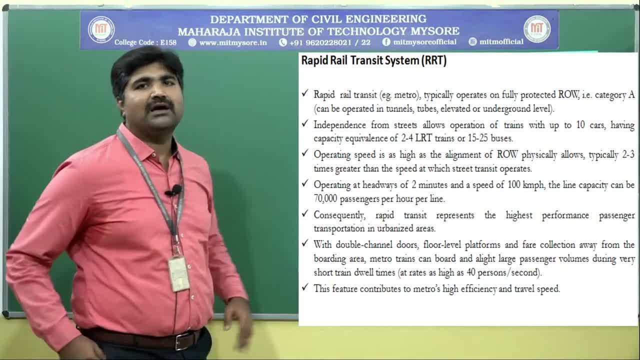 and this feature contributes to Metro a and this feature contributes to Metro a year efficiency and travel speed in year efficiency and travel speed in year efficiency and travel speed in urban Alva. you have Bangalore before urban Alva. you have Bangalore before urban Alva. you have Bangalore before providing this Metro from Genghis to 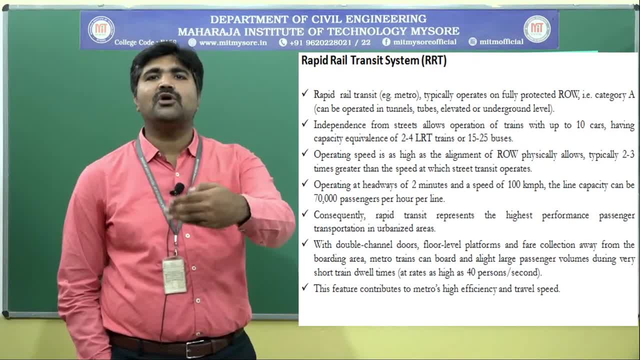 providing this Metro from Genghis to providing this Metro from Genghis to majestic travel. medley can active around majestic travel. medley can active around majestic travel. medley can active around. it takes it was taking 40 minutes to one. it takes it was taking 40 minutes to one. 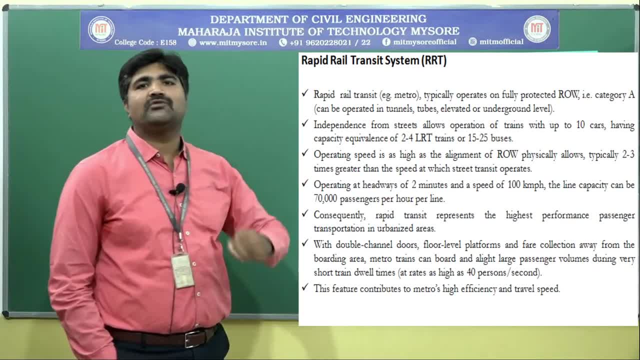 it takes. it was taking 40 minutes to one hour by Metro. now it has been decreased. hour by Metro. now it has been decreased. hour by Metro. now it has been decreased. okay, within 20 to 25 minutes we can. okay, within 20 to 25 minutes we can. 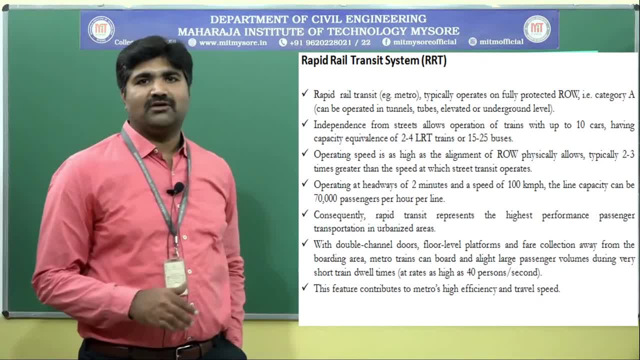 okay. within 20 to 25 minutes, we can. within 20 minutes, we can reach the. within 20 minutes, we can reach the. within 20 minutes, we can reach the. majestic, okay, city center in Bangalore. majestic, okay, city center in Bangalore. majestic, okay, city center in Bangalore: okay, this is because of the efficiency. 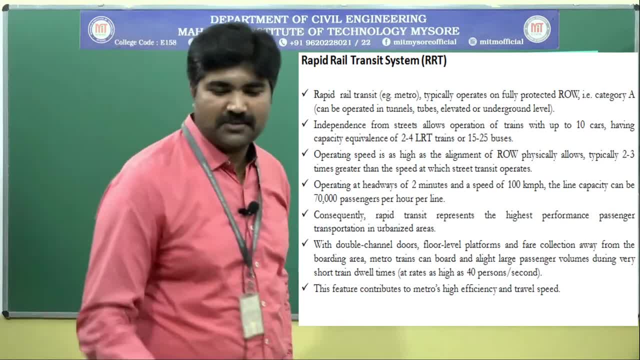 okay, this is because of the efficiency. okay, this is because of the efficiency of the Metro. because of the IR speed. okay of the Metro, because of the IR speed. okay of the Metro, because of the IR speed. okay. next mono rails: okay, mono rails as. next mono rails: okay, mono rails as. 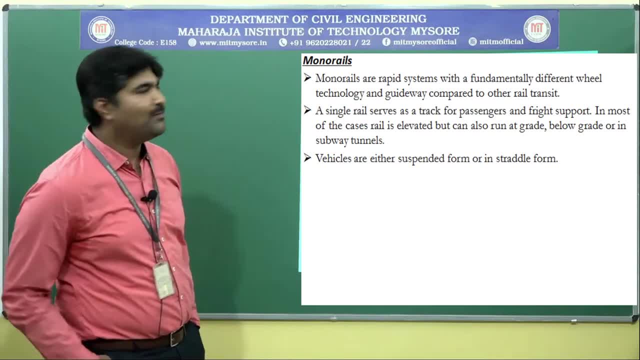 next, mono rails: okay, mono rails, as the name indicates mono rail, there will be. the name indicates mono rail, there will be. the name indicates mono rail, there will be single rail, that is the mono rail. okay, single rail, that is the mono rail. okay, single rail, that is the mono rail. okay, mono rails are rapid system with a 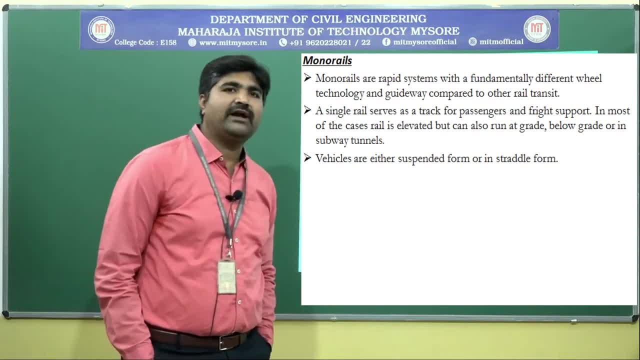 mono rails are rapid system with a mono rails are rapid system with a fundamentally different wheel technology, fundamentally different wheel technology, fundamentally different wheel technology. there will be a different wheel. there will be a different wheel. there will be a different wheel technology and guideway compared to other. 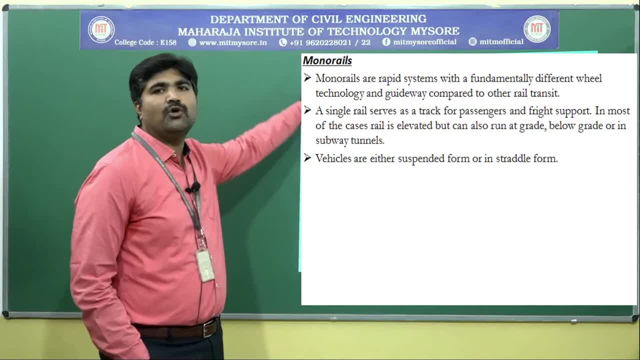 technology and guideway compared to other technology and guideway compared to other rail transit. okay, see a single rail as I rail transit. okay, see a single rail as I rail transit. okay, see a single rail, as I told, mono rail means single rail, single. told mono rail means single rail, single. 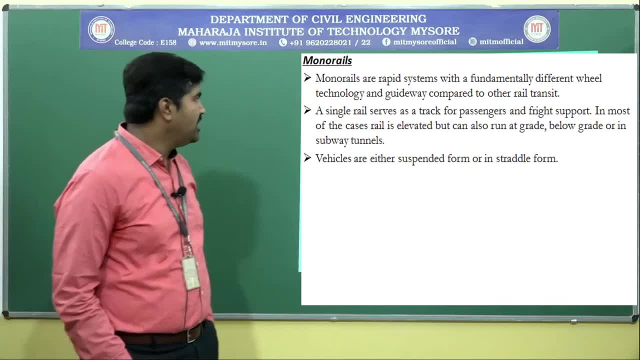 told. mono rail means single rail. single rail serves as a track for passengers. rail serves as a track for passengers. rail serves as a track for passengers and freight support in most of the cases and freight support in most of the cases and freight support in most of the cases. rail is elevated but can also at a great 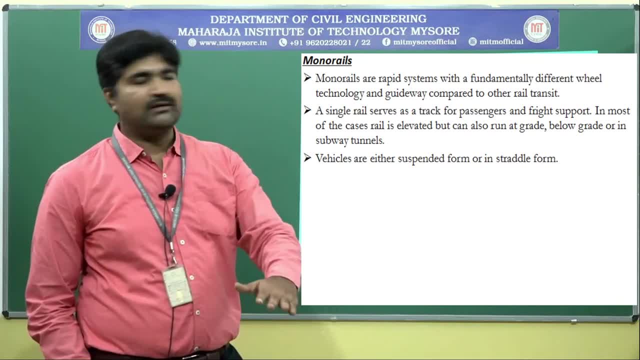 rail is elevated, but can also at a great rail is elevated, but can also at a great below grade. okay, below grade means it is below grade. okay, below grade means it is below grade. okay, below grade means it is underground level. okay, great, separated. underground level. okay, great, separated. 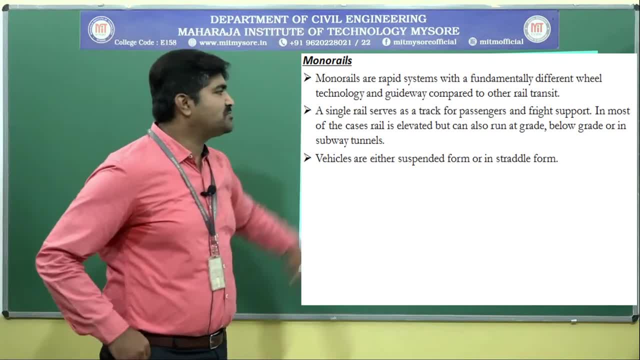 underground level. okay, great, separated means elevated, that is the flyover. means elevated, that is the flyover. means elevated, that is the flyover. vehicles are either suspended form or in vehicles are either suspended form or in. vehicles are either suspended form or in straddle form. okay, here the vehicles may. 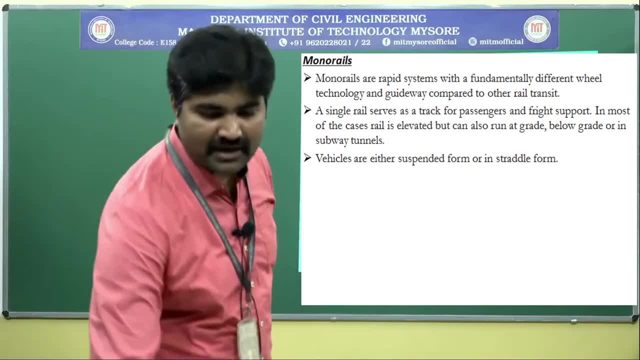 straddle form. okay, here the vehicles may straddle form. okay, here the vehicles may be in suspended form or in the straddle. be in suspended form or in the straddle. be in suspended form or in the straddle form you can observe in the figure. okay, 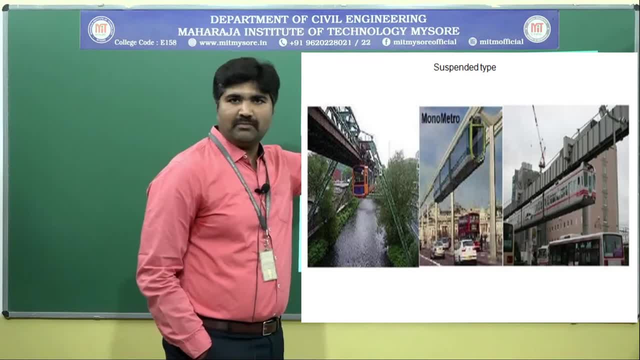 form you can observe in the figure. okay, form you can observe in the figure. okay, see, this is the suspended form. okay, there see, this is the suspended form. okay, there see, this is the suspended form. okay, there will be a horizontal beam. okay, will be a horizontal beam, okay. 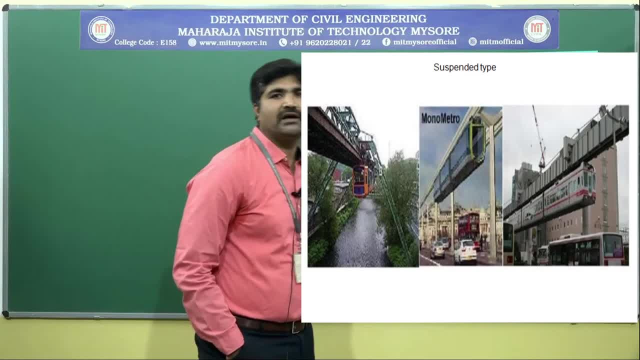 will be a horizontal beam. okay, horizontal beam is the other case. horizontal beam is the other case. horizontal beam is the other case. suspended- the vehicle you can observe. suspended- the vehicle you can observe. suspended- the vehicle you can observe here. okay, the vehicles will be suspended here. okay, the vehicles will be suspended. 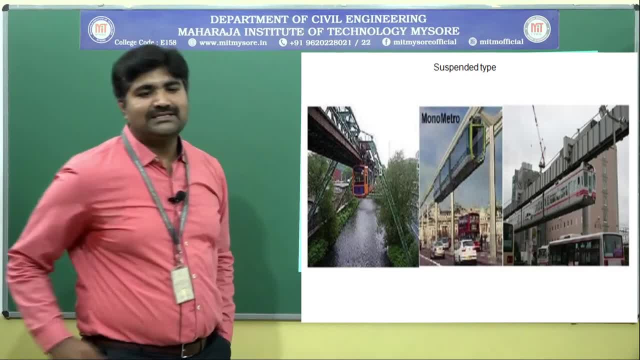 here. okay, the vehicles will be suspended. to this horizontal horizontal beams. okay, to this horizontal horizontal beams. okay, to this horizontal horizontal beams. okay, straddle under, okay, okay, this is the straddle under, okay, okay, this is the straddle under, okay, okay, this is the straddle. okay. over the beams: okay, the. 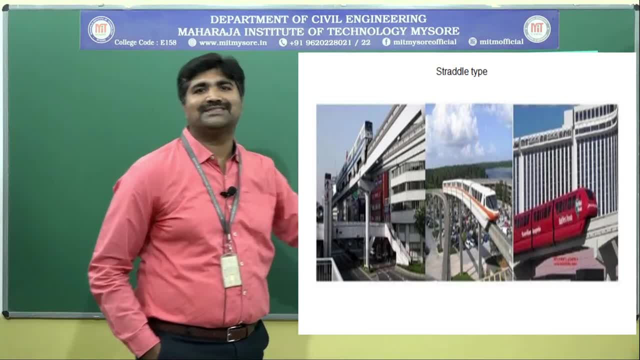 straddle. okay, over the beams. okay, the straddle. okay, over the beams. okay, the monorail that will travel over the beams, monorail that will travel over the beams, monorail that will travel over the beams, over the horizontal beams. this is the over the horizontal beams, this is the. 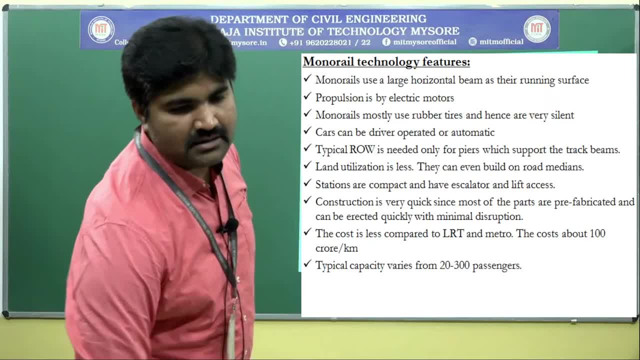 over the horizontal beams. this is the straddle form. okay, monorail technology, straddle form. okay, monorail technology, straddle form. okay, monorail technology features: okay, see the monorail use a features. okay, see the monorail use a features. okay, see the monorail use a large horizontal beam means 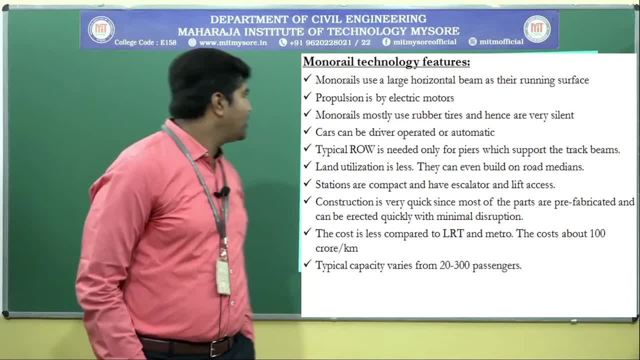 large horizontal beam means large horizontal beam means lengthy horizontal beam as their running, lengthy horizontal beam as their running, lengthy horizontal beam as their running surface. okay, propulsion is by electric surface. okay, propulsion is by electric surface. okay, propulsion is by electric motors: okay, electric traction, okay, which motors? okay, electric traction, okay, which. 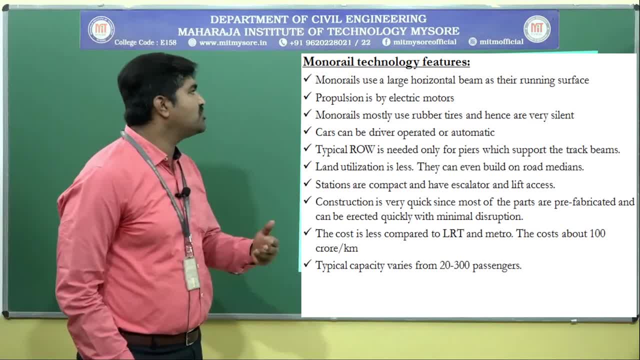 motors: okay. electric traction: okay. which is pollution free: okay. environmental is pollution free: okay. environmental is pollution free, okay. environmental friendly: okay. monorails mostly use friendly: okay. monorails mostly use friendly: okay. monorails mostly use rubber types: okay, hence the it creates rubber types. okay, hence the it creates. 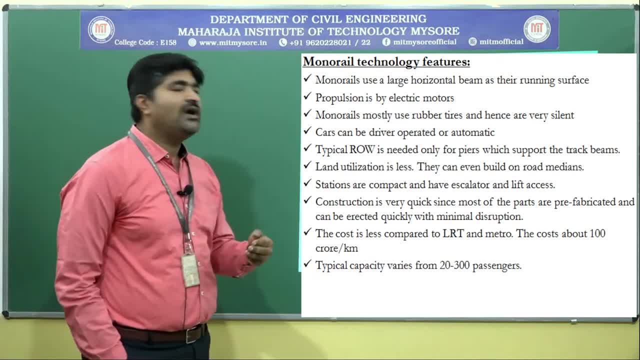 rubber types okay. hence the. it creates less noise. it is very silent, okay. cars- less noise, it is very silent, okay. cars- less noise, it is very silent, okay. cars can be driver operated at automatic can be driver operated at automatic can be driver operated at automatic. many today is automatically operated okay. 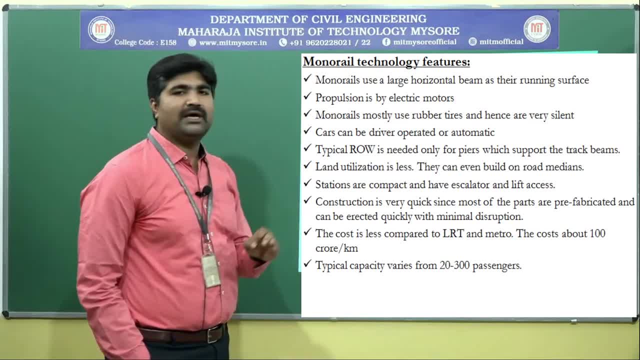 many today is automatically operated. okay, many today is automatically operated: okay. next typical. next typical. next typical write-off is needed only for peers. okay, write-off is needed only for peers. okay, write-off is needed only for peers. okay, the width required will be very less as the width required will be very less as. 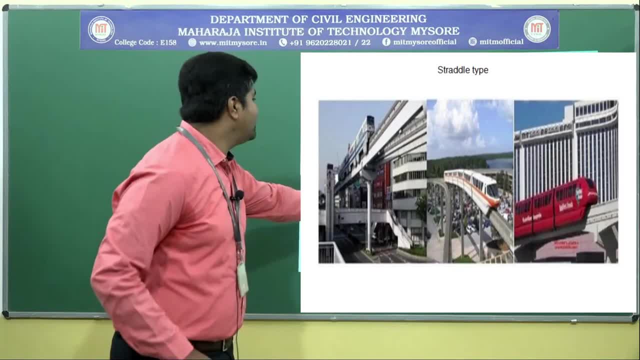 the width required will be very less, as we have seen in the figure you can. we have seen in the figure you can. we have seen in the figure you can observe in this figure: okay, only the observe in this figure. okay, only the observe in this figure. okay, only the peers. for this we need a space, okay, to. 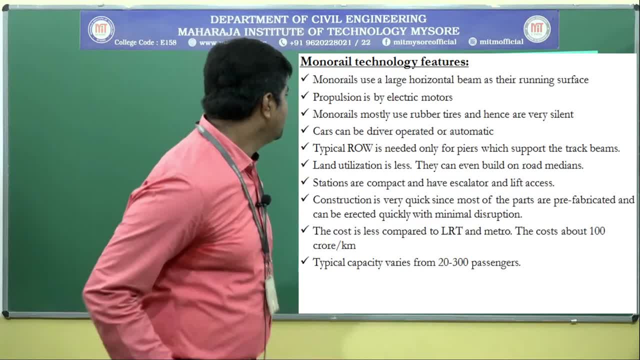 peers for this. we need a space okay, to peers for this. we need a space, okay, to construct this, construct this, construct this, okay, okay, okay. land utilization is very less because, as land utilization is very less, because, as land utilization is very less, because, as you have seen in the figure, it needs. 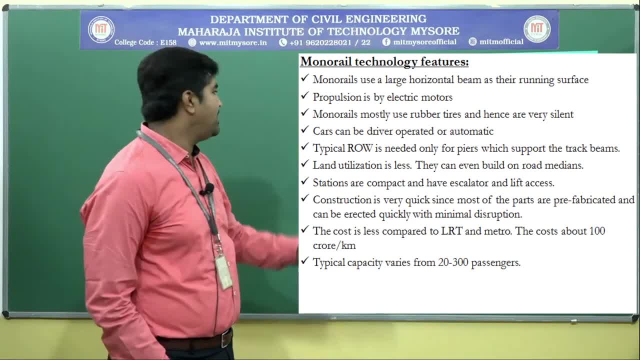 you have seen in the figure it needs. you have seen in the figure it needs place only to provide the peers columns place only to provide the peers columns place only to provide the peers columns. okay, it utilizes the less space they. okay, it utilizes the less space they. okay, it utilizes the less space. they can even build on the road medians road. can even build on the road medians road. can even build on the road medians road medians in either 1.2 to 1 to 2 meter medians in either 1.2 to 1 to 2 meter. 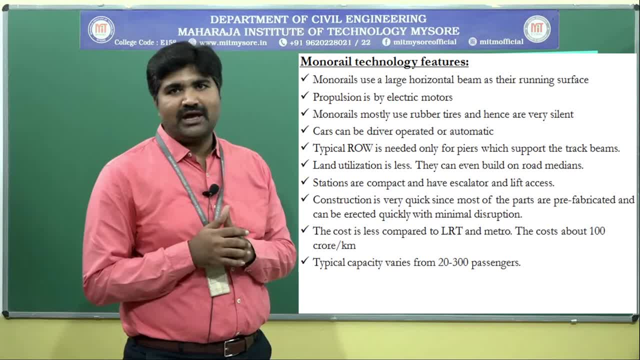 medians in either 1.2 to 1 to 2 meter, anywhere that can be sufficient to build, anywhere that can be sufficient to build, anywhere that can be sufficient to build the peers okay, the peers okay, the peers okay. and stations are compact and have escalator. 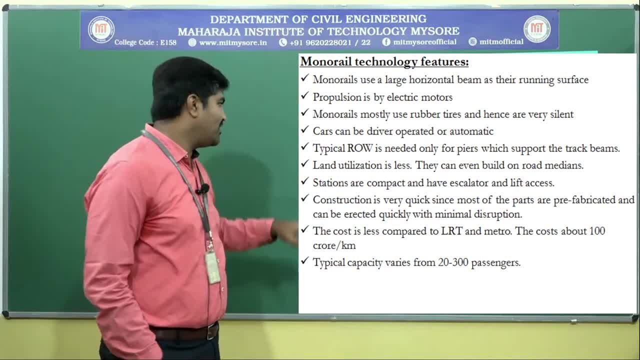 and stations are compact and have escalator and stations are compact and have escalator- okay, elevated, so we have to provide okay, elevated, so we have to provide okay, elevated. so we have to provide the escalator: okay, construction is very. the escalator: okay, construction is very. 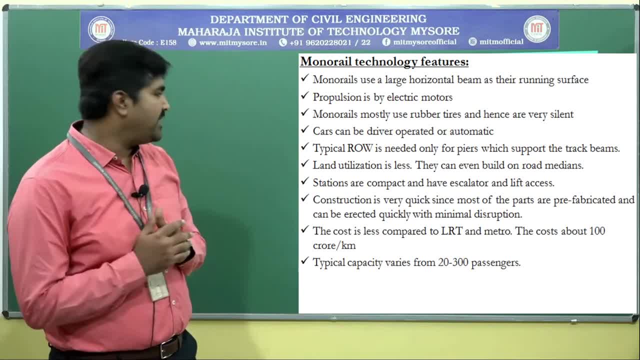 the escalator: okay, construction is very quick, since most of the parts are free. quick, since most of the parts are free. quick, since most of the parts are free. sorry, pre-fabricated and can be erected. sorry, pre-fabricated and can be erected. sorry, pre-fabricated and can be erected. very quickly with minimum disruption, as very quickly, with minimum disruption, as very quickly, with minimum disruption, as we have seen just. we have to what we we have seen just. we have to what we, we have seen just. we have to what we have to. we have to construct the peers have to. we have to construct the peers. 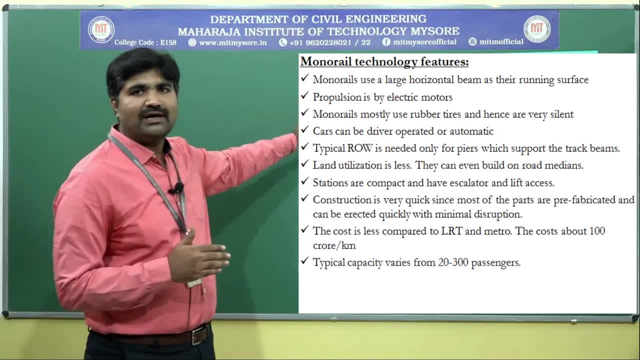 have to. we have to construct the peers light rail transit: okay, the cost of this light rail transit: okay, the cost of this light rail transit. okay, the cost of this monorail, okay. cost of construction: will monorail okay, cost of construction. will monorail okay. cost of construction will be very less for this monorail, okay, when? 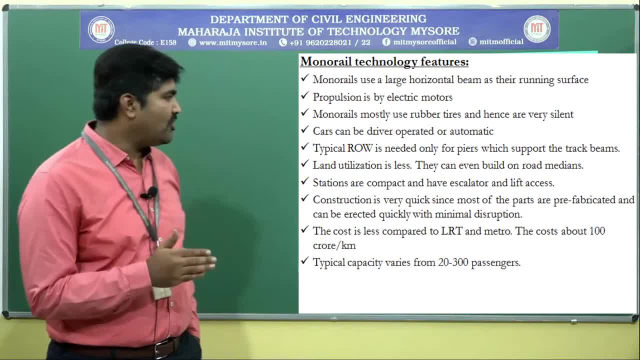 be very less for this monorail. okay, when? be very less for this monorail? okay, when compared to lrt, that is, the light rail, compared to lrt, that is the light rail compared to lrt, that is the light rail. transit and the metro. okay, the cost. 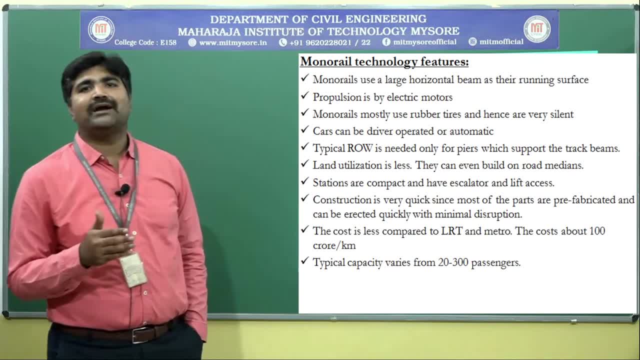 transit and the metro: okay, the cost: transit and the metro: okay. the cost required: okay. to provide the facility for required: okay, to provide the facility for required: okay. to provide the facility for monorail is 100 crore per kilometer. okay, monorail is 100 crore per kilometer, okay. 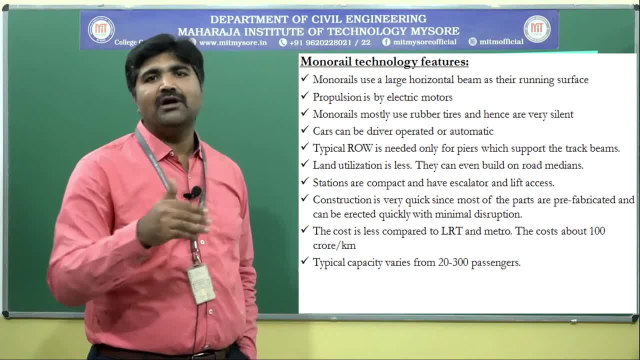 monorail is 100 crore per kilometer. okay, that is more in case of metro, or that is more in case of metro, or that is more in case of metro or light rail transit or metro line activity, light rail transit or metro line activity, light rail transit or metro line activity. it requires 500 to 600 crores per it requires 500 to 600 crores per. it requires 500 to 600 crores per kilometer. okay, see, the capacity varies kilometer. okay, see, the capacity varies kilometer. okay, see, the capacity varies from 20 to 300 passengers. that depends from 20 to 300 passengers. that depends. 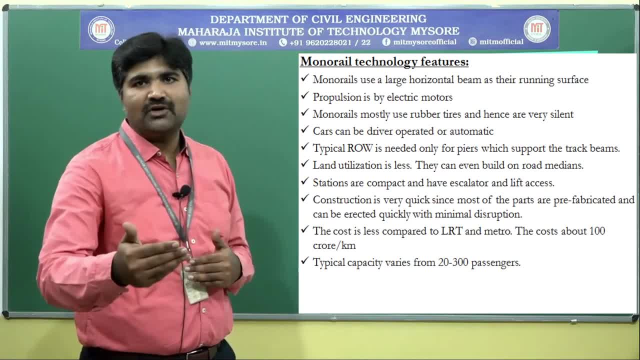 from 20 to 300 passengers. that depends upon the bogies or cars wagons and upon the bogies or cars wagons and upon the bogies or cars wagons. and attached moderate tv: okay, engine based. attached moderate tv: okay, engine based. attached moderate tv: okay, engine based upon that: the passion, the number of 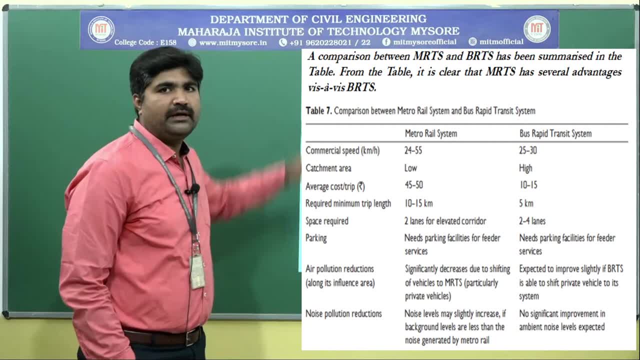 upon that the passion, the number of. upon that the passion, the number of passengers can be accommodated. passengers can be accommodated. passengers can be accommodated. next comparison between the mrts and next comparison between the mrts and next comparison between the mrts and brts. okay, what do you mean by mrts? 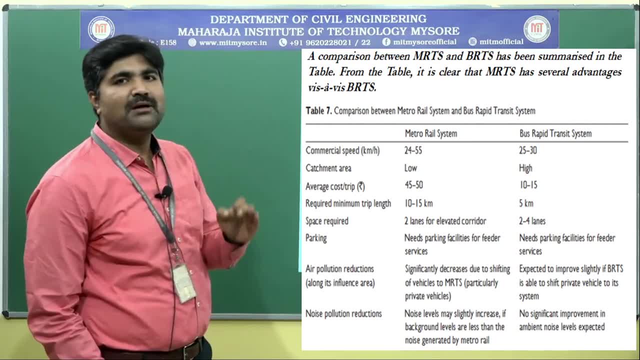 brts- okay. what do you mean by mrts? brts- okay. what do you mean by mrts? that is the metro rail transit system. that is the metro rail transit system. that is the metro rail transit system. brts means bus rapid transit system has. brts means bus rapid transit system has. 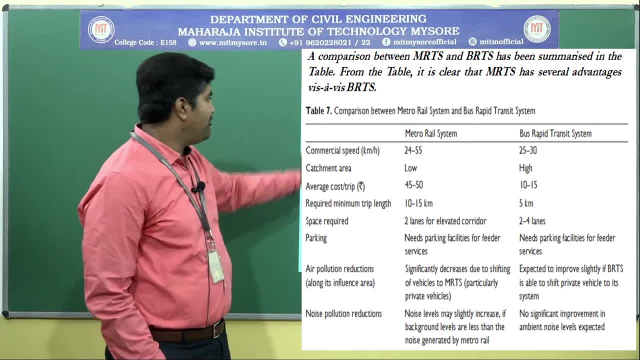 brts means bus rapid transit system, has been summarized in the table. okay, by been summarized in the table. okay, by been summarized in the table. okay, by keeping some factors. okay, by keeping keeping some factors. okay, by keeping keeping some factors. okay, by keeping some characteristics: okay. see, this is the 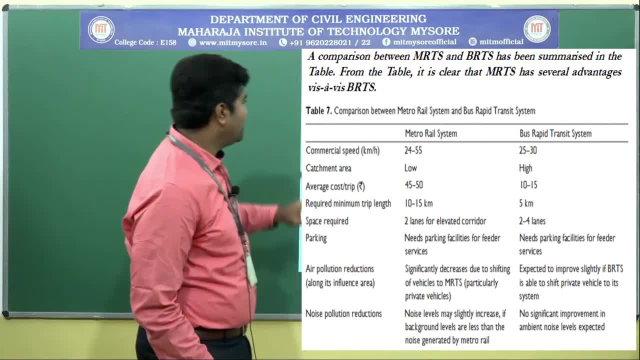 some characteristics. okay, see, this is the some characteristics. okay, see, this is the metro rail system and this is the bus metro rail system, and this is the bus metro rail system and this is the bus rapid transit system. okay, the first rapid transit system. okay, the first rapid transit system. okay, the first factor is the commercial speed. okay, as. 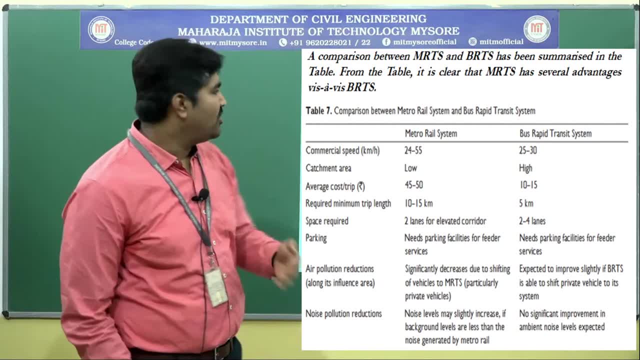 factor is the commercial speed. okay, as factor is the commercial speed. okay, as we know, speed yaduk speed, just the metro. we know speed yaduk speed, just the metro. we know speed yaduk speed, just the metro that has the high speed. okay, that can. 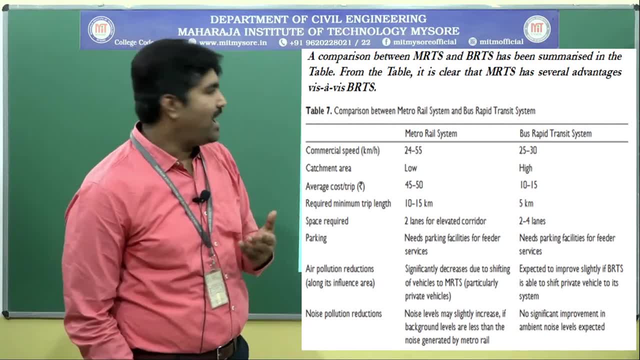 that has the high speed- okay, that can. that has the high speed- okay, that can. travel around 24 to 55. travel around 24 to 55. travel around 24 to 55. 55 kilometer per hour- here the speed. 55 kilometer per hour- here the speed. 55 kilometer per hour. here the speed will be less. that is 25 to 30 kilometer will be less. that is 25 to 30 kilometer will be less. that is 25 to 30 kilometer per hour. okay, catchment area, okay the. 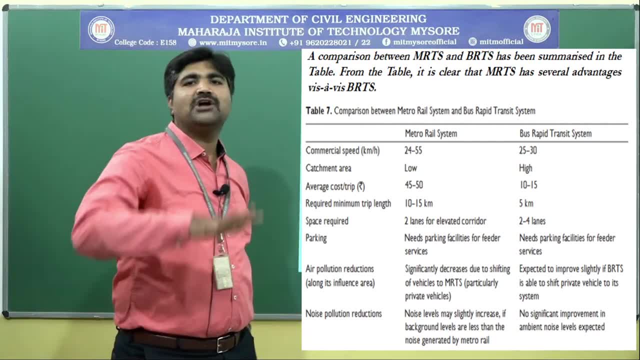 per hour: okay, catchment area: okay the per hour: okay, catchment area. okay, the catchment area for metro: it will be less catchment area for metro. it will be less catchment area for metro. it will be less because we cannot reach all the area. because we cannot reach all the area. 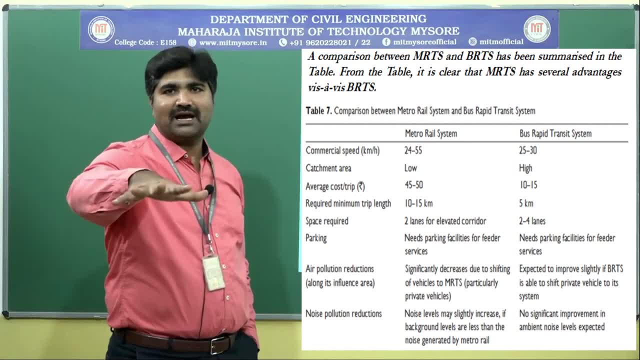 because we cannot reach all the area. alwa i got bangalore. if you take bangalore. alwa, i got bangalore. if you take bangalore, alwa, i got bangalore. if you take bangalore, okay, you're gonna reach ugly kagala. okay, you're gonna reach ugly kagala. 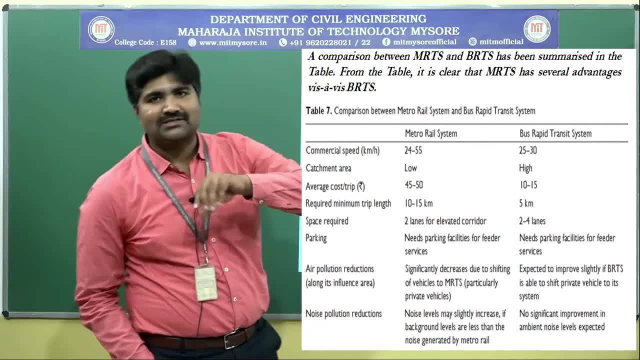 okay, you're gonna reach ugly kagala, okay. so, but the bus can reach all the okay. so, but the bus can reach all the okay. so, but the bus can reach all the areas. okay, the catchment area for the areas. okay, the catchment area for the. areas: okay. the catchment area for the bus will be more okay. next average cost bus will be more okay. next average cost bus will be more okay. next average cost trip: okay. average cost trip will be less trip. okay. average cost trip will be less trip. okay. average cost trip will be less. in case of metro, that may be 4.5 to 5. in case of metro, that may be 4.5 to 5. in case of metro, that may be 4.5 to 5 rupees per trip. okay, there, it may be 10 rupees per trip. okay, there, it may be 10 rupees per trip. okay, there, it may be 10 to 15 rupees. okay, required minimum trip. to 15 rupees. okay, required minimum trip to 15 rupees. okay, required minimum trip length: okay, the minimum trip length is length. okay, the minimum trip length is length. okay, the minimum trip length is 10 to 15 kilometer. okay, in cities in 10 to 15 kilometer. okay in cities in. 10 to 15 kilometer. okay, in cities, in bangalore, if you take example the bangalore, if you take example the bangalore, if you take example, the minimum trip length in the metro will be minimum trip length in the metro will be minimum trip length in the metro will be two to five kilometer means from one. two to five kilometer means from one. two to five kilometer means from one stop to next stop. that is the minimum stop to next stop. that is the minimum stop to next stop. that is the minimum trip length: okay in bus, that may be two. trip length: okay in bus, that may be two. trip length: okay, in bus, that may be two to five kilometer. that is the minimum to five kilometer. that is the minimum to five kilometer. that is the minimum trip length. okay, next space required: okay, trip length: okay. next space required: okay, trip length: okay. next space required. okay, what is the space required? okay, two. 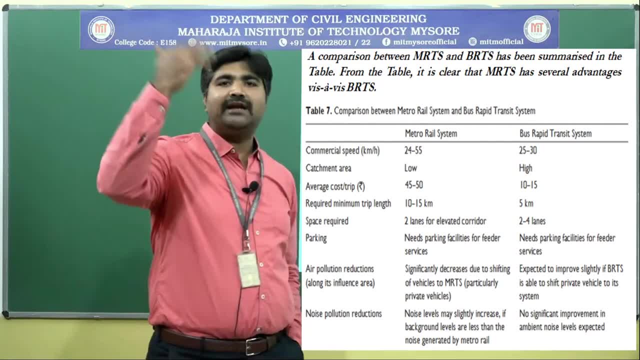 what is the space required? okay, two. what is the space required? okay, two lanes for elevated corridor, as we have lanes for elevated corridor, as we have lanes for elevated corridor, as we have seen bangalore metro, you know elevated. seen bangalore metro, you know elevated, seen bangalore metro, you know elevated corridor. there will be two lanes, okay to. 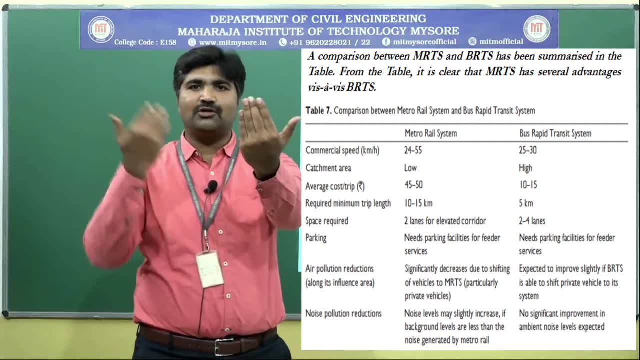 corridor there will be two lanes. okay, to corridor there will be two lanes. okay to carry in both the direction. okay, one to carry in both the direction. okay, one to carry in both the direction. okay, one to train: one: the metro walk through in on train. one: the metro walk through in on. 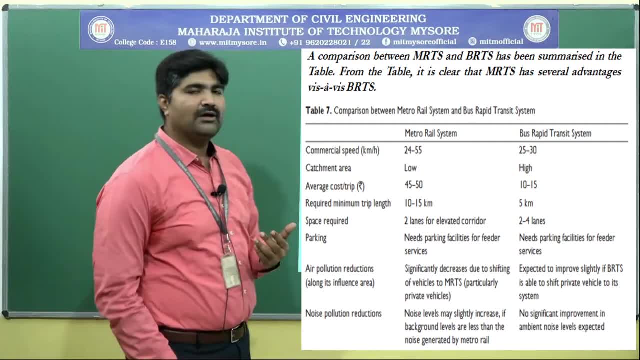 train one, the metro, walk through in on the metro bar back with the. we have. we the metro bar back with the. we have. we the metro bar back with the. we have. we should have a two lane, okay, and next two should have a two lane, okay, and next two. 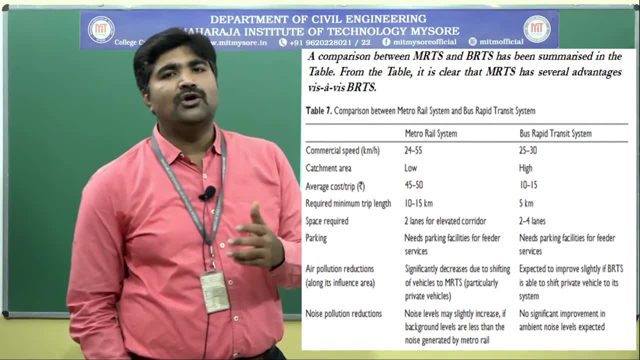 should have a two lane, okay, and next two to four lanes for the buses. single to four lanes for the buses. single to four lanes for the buses single line. a line up to the bus operate line. a line up to the bus operate line. a line up to the bus operate Madhya Gala to line it through an act. 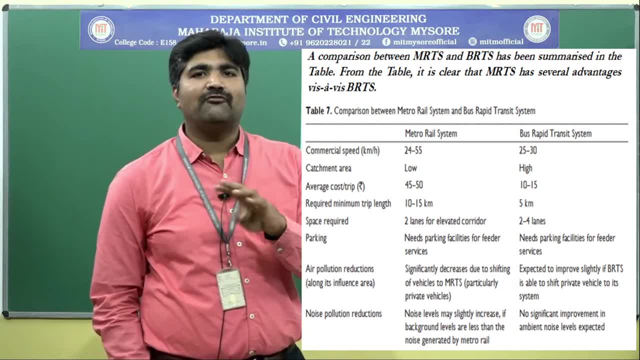 Madhya Gala to line it through an act. Madhya Gala to line it through an act of the due to congestion. it takes more of the due to congestion. it takes more of the due to congestion. it takes more line. okay, there should be a at least four. line. okay, there should be a at least four line. okay, there should be a at least four lines. is that easier to operate mode lines? is that easier to operate mode lines? is that easier to operate mode? about the okay, divided carriage with two. about the okay, divided carriage with two. 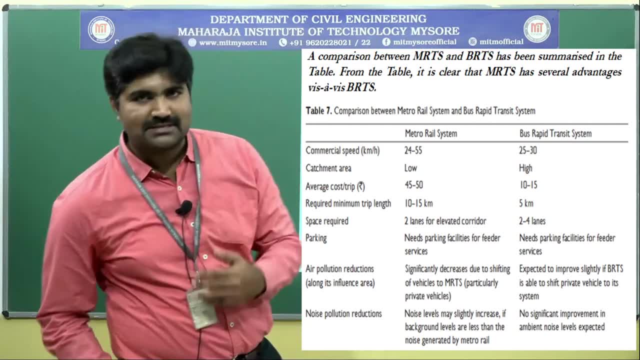 about the okay, divided carriage with two lines on: either says that will be easy, lines on, either. says that will be easy, lines on either. says that will be easy to carry the buses: okay. next parking to carry the buses: okay. next parking to carry the buses: okay. next parking needs parking facilities for feeder. 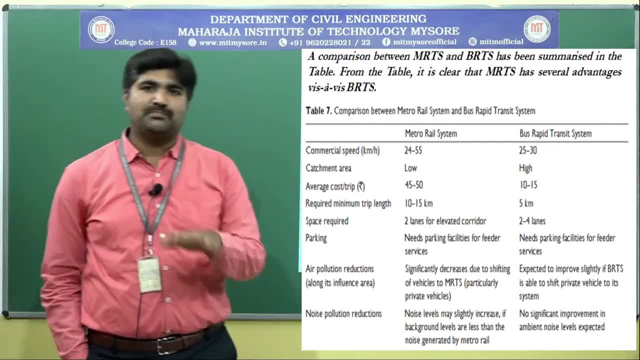 needs parking facilities for feeder, needs parking facilities for feeder system. okay, this metro station needs a system. okay, this metro station needs a system. okay, this metro station needs a parking space. okay for the feeder system. parking space okay for the feeder system. parking space okay for the feeder system. feeder system at the money in the now. oh, 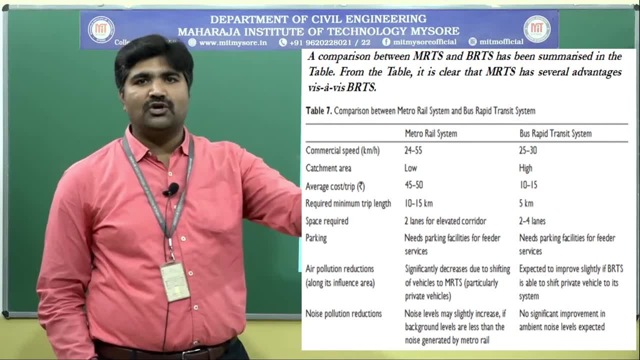 feeder system at the money in the now. oh, feeder system at the money in the now, oh, you got one kilometer metro station in. you got one kilometer metro station in. you got one kilometer metro station in the next day. we cannot walk to reach that. 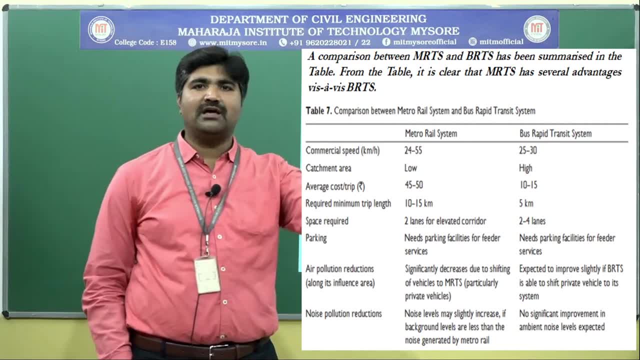 the next day we cannot walk to reach that. the next day we cannot walk to reach that metro station. at that time, we will use metro station. at that time, we will use metro station. at that time, we will use our own personalized vehicle- two-wheeler- our own personalized vehicle, two-wheeler. 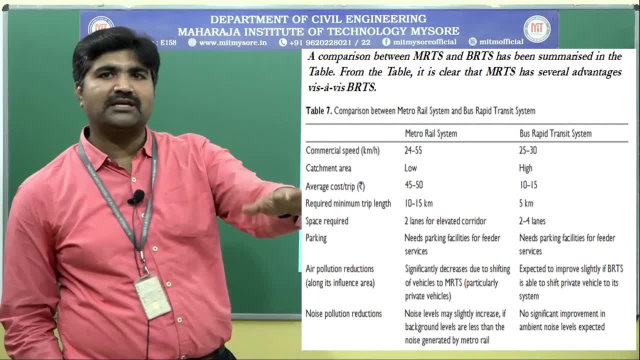 our own personalized vehicle, two-wheeler in a use Marty, we okay, I think. a park in a use Marty, we okay, I think. a park in a use Marty, we okay, I think a park Marley can space back parking space is. Marley can space back parking space is. 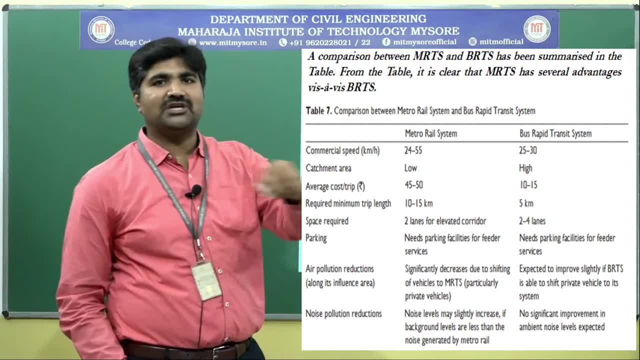 Marley can space back. parking space is needed. okay, for the feeder system now needed. okay, for the feeder system now needed. okay for the feeder system now. the feed Martha, the allegory chocolate. the feed Martha, the allegory chocolate. the feed Martha, the allegory chocolate. okay, we need a parking space needs. 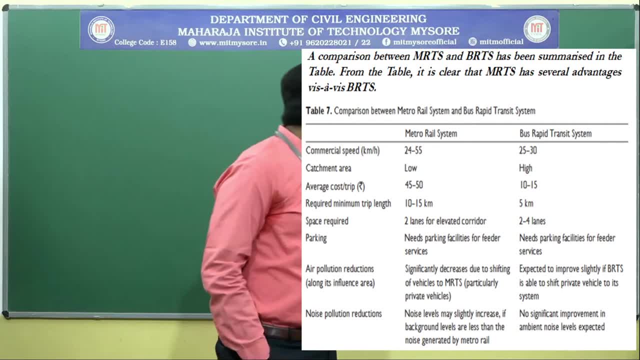 okay, we need a parking space needs. okay, we need a parking space. needs parking facilities for feeder services. parking facilities for feeder services. parking facilities for feeder services- here also we need a parking space. but it here also we need a parking space. but it here also we need a parking space. but it will be less when compared to this. okay, 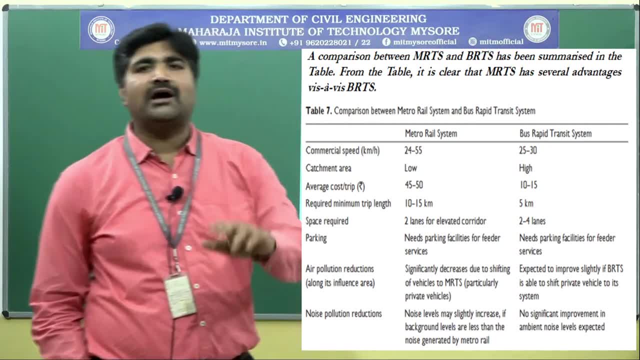 will be less when compared to this: okay, will be less when compared to this: okay. bus bus stations: Allah, almost near earth. bus bus stations: Allah, almost near earth. bus bus stations: Allah, almost near earth. and Amma origin is stations- okay, so, and Amma origin is stations- okay, so. 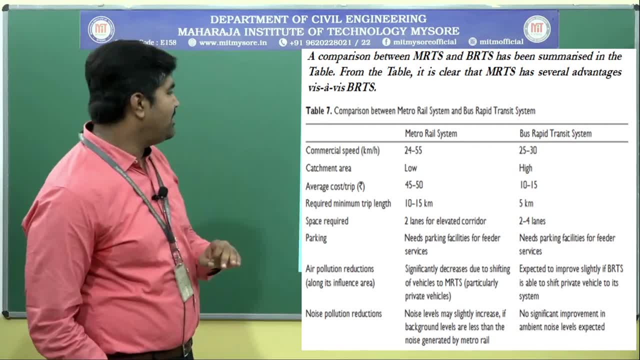 and Amma origin is stations. okay, so, bacteria next air pollution reduction, bacteria next air pollution reduction. bacteria next air pollution reduction. okay, okay, there will be significantly. okay. okay, there will be significantly okay, okay, there will be significantly decreases. okay, significantly decreases due. decreases, okay, significantly decreases due. 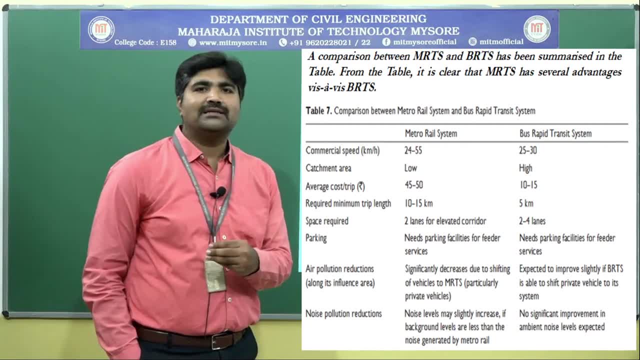 decreases. okay, significantly decreases due to shifting of vehicles to mrts. okay to shifting of vehicles to mrts. okay to shifting of vehicles to mrts. okay, in active in a world, a metro mass in active in a world, a metro mass in active in a world. a metro mass transportation provide: Madagha: okay. 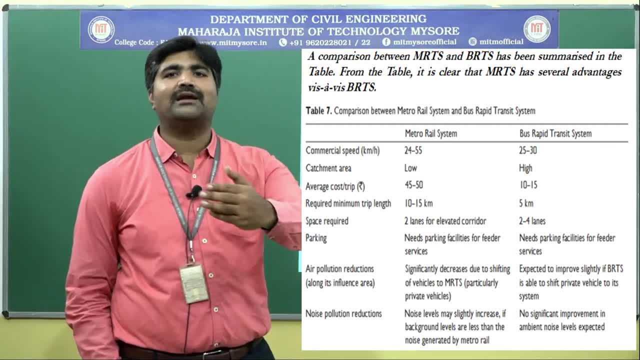 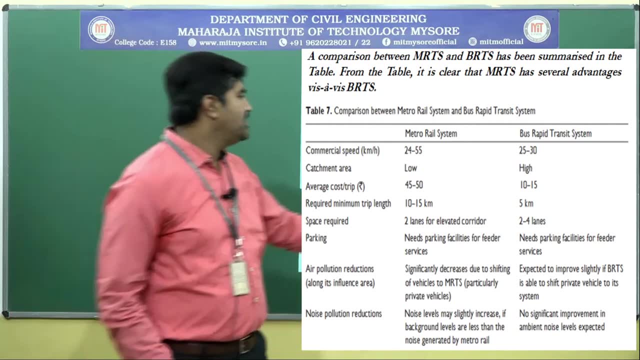 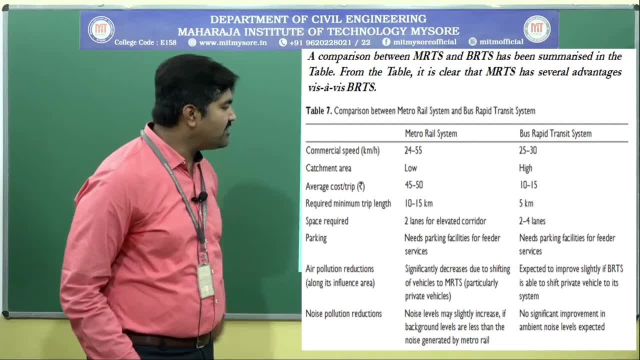 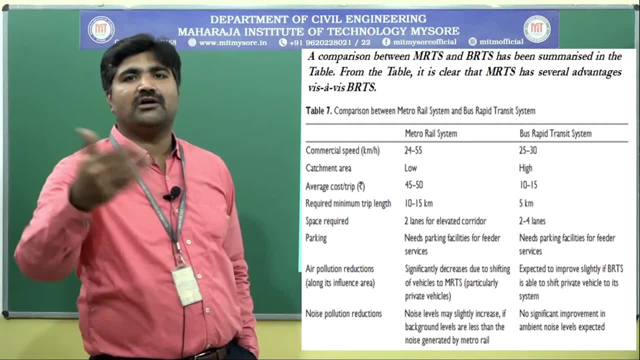 okay, steel rails and steel wheels. okay okay, steel rails and steel wheels. okay, enough to this steel. will to steel rail. enough to this steel. will to steel rail. enough to this steel. will to steel rail. smell: move up to render in the soul pole. smell, move up to render in the soul pole. 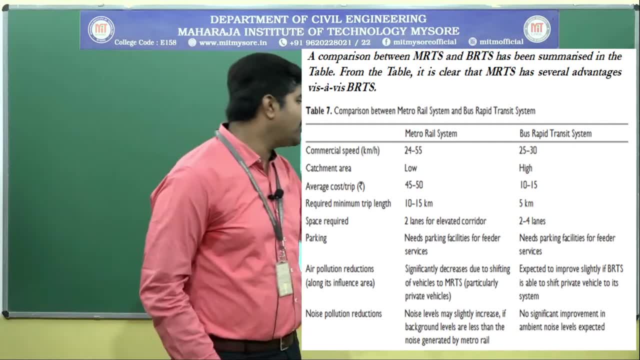 smell, move up to render in the soul pole noise. so Justin air today, okay, yeah, no noise. so Justin air today, okay, yeah, no noise. so Justin air today, okay, yeah, no. significant improvement in the ambient, significant improvement in the ambient, significant improvement in the ambient. noise: okay, there will be RN and all the. 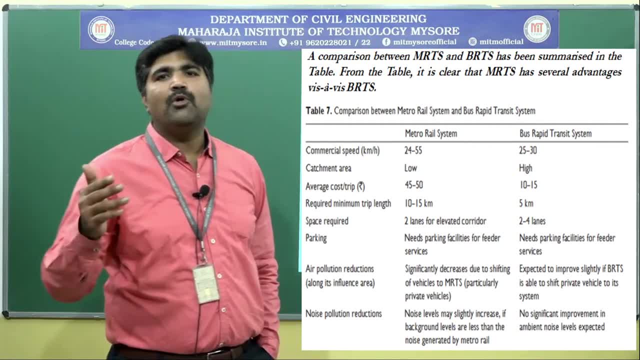 noise. okay, there will be RN and all the noise. okay, there will be RN and all the due to congestion idling earlier. other in due to congestion idling earlier. other in due to congestion idling earlier. other in the Guardian. after that, there will be the Guardian. after that, there will be. 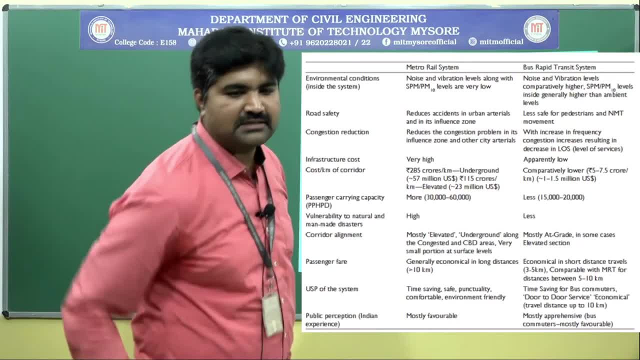 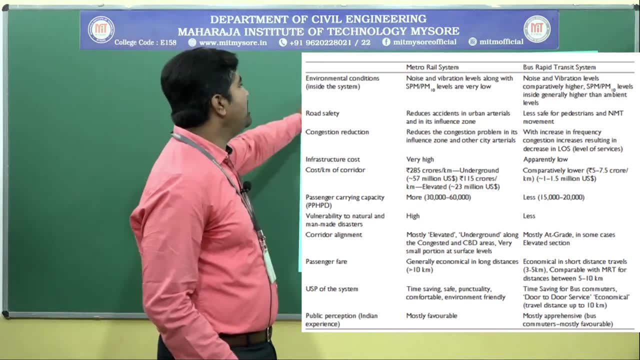 the Guardian. after that, there will be more noise. next environmental conditions: more noise. next environmental conditions: more noise. next environmental conditions: okay, noise and vibrations along with the. okay noise and vibrations along with the. okay noise and vibrations along with the levels. okay, here there will be noise, noise. 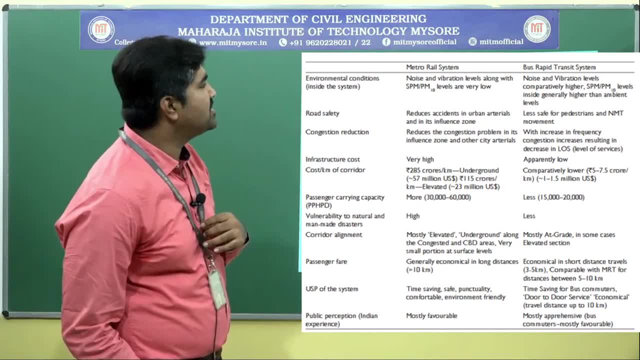 levels. okay, here there will be noise, noise levels. okay, here there will be noise. noise with the vibration level super Justin with the vibration level, super Justin, with the vibration level, super Justin. air today. there the noise and vibration air today. there the noise and vibration air today. there the noise and vibration levels comparatively, you think, in the 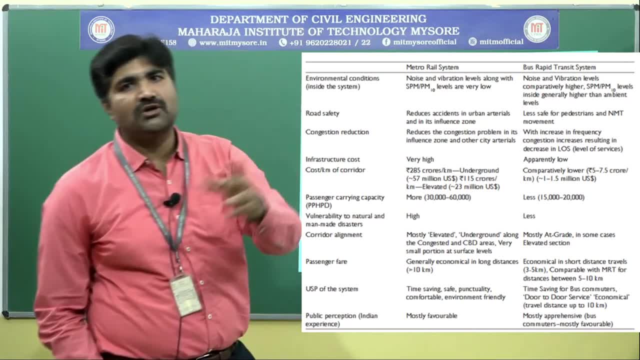 levels comparatively. you think in the levels comparatively. you think in the just hear today, there the noise due to just hear today, there the noise due to just hear today, there the noise due to. you know vehicles to move the dog luna. you know vehicles to move the dog luna. 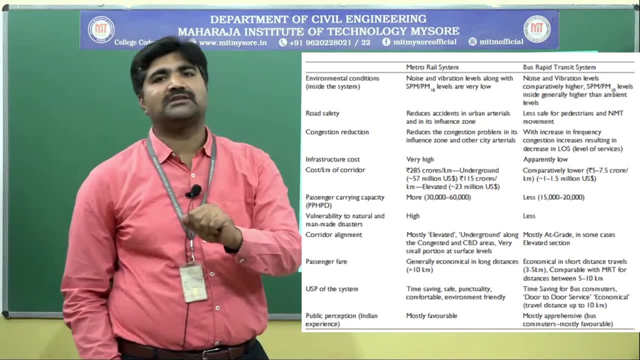 you know, vehicles to move the dog luna noise here today, okay. and also idling noise here today, okay. and also idling noise here today, okay. and also idling traffic congestionally stoppages. are traffic congestionally stoppages. are traffic congestionally stoppages? are you know, idling conditionally though, okay. 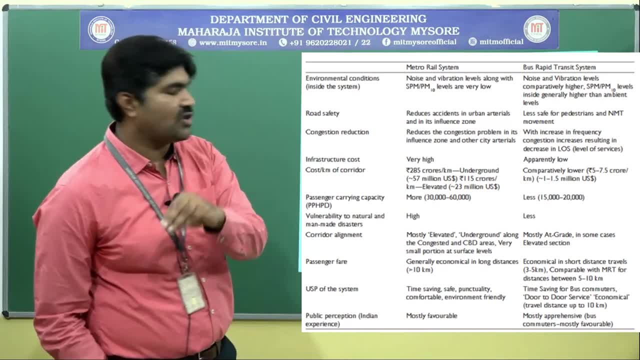 you know idling conditionally, though okay. you know idling conditionally, though okay. inner congestion are they due to, and inner congestion are they due to, and inner congestion are they due to, and aren't aren't matter in the adrenaline, aren't aren't matter in the adrenaline? 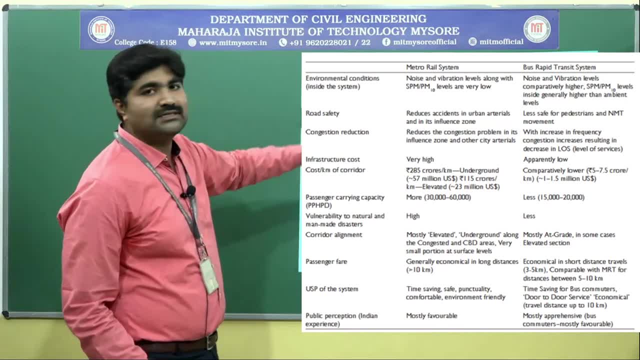 aren't, aren't matter in the adrenaline: active noise to just hear today, and active noise to just hear today, and active noise to just hear today. and road safety: okay, this metro system, road safety. okay, this metro system, road safety. okay, this metro system reduces the accidents: okay, accidents in. 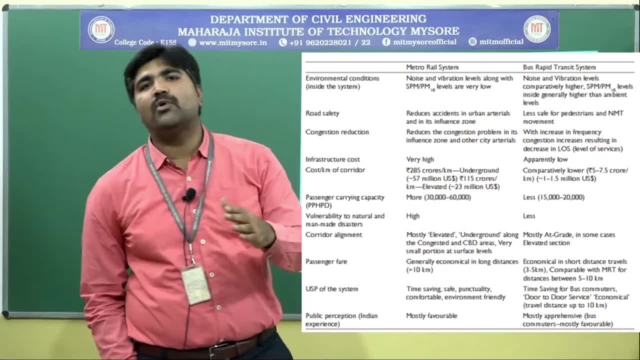 reduces the accidents- okay, accidents in reduces the accidents: okay, accidents in urban: okay, this is less safe for urban. okay, this is less safe for urban. okay, this is less safe for pedestrians. we are seeing more accidents, pedestrians. we are seeing more accidents, pedestrians. we are seeing more accidents in the roads. okay, the people are seeing. 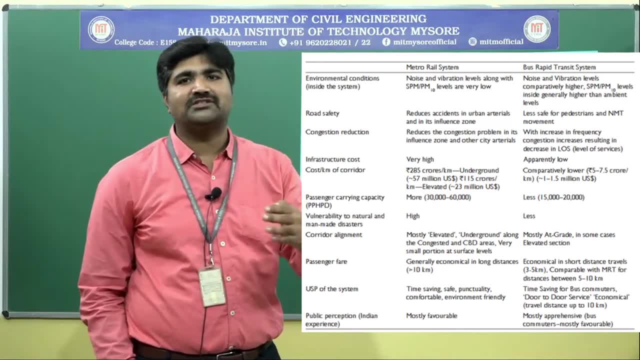 in the roads. okay, the people are seeing in the roads. okay, the people are seeing that, okay, less safe on the streets, the that okay. less safe on the streets, the that okay, less safe on the streets. the people are observing that streets are. people are observing that streets are. 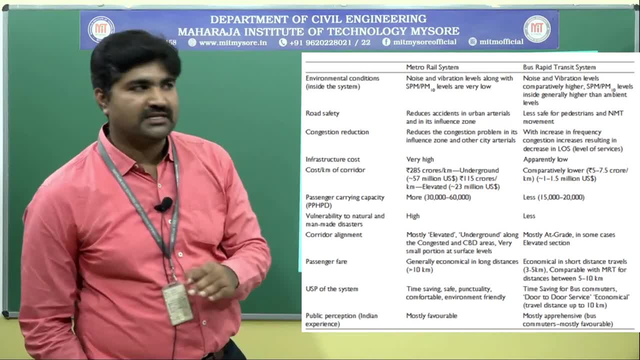 people are observing that streets are less safe to move. means that to less safe to move. means that to less safe to move means that to exclusively for pedestrians- okay. next. exclusively for pedestrians- okay. next. exclusively for pedestrians- okay. next. next conjunction reduction: okay, reduces. next conjunction reduction: okay, reduces. 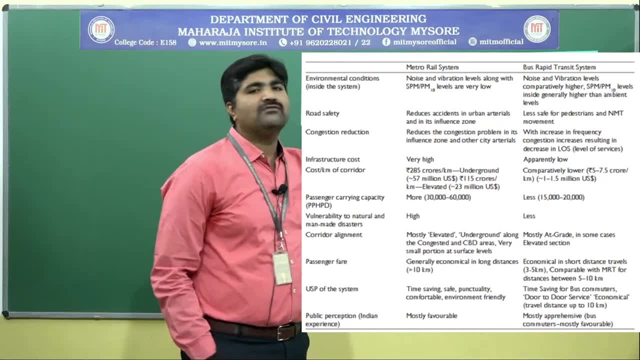 next conjunction: reduction: okay, reduces the congestion. this relieves the the congestion. this relieves the the congestion. this relieves the congestion. okay, there we have some congestion. okay, there, we have some congestion. okay, there, we have some congestion here today. okay, in case of congestion here today. okay, in case of. 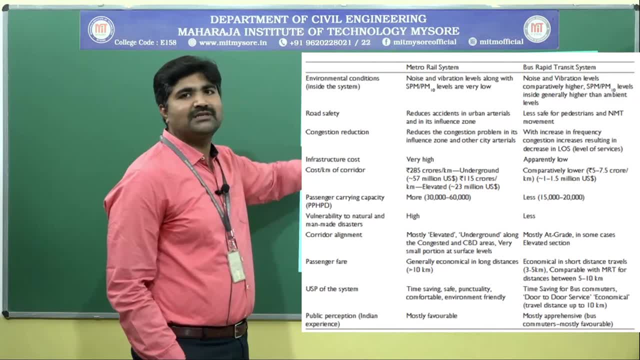 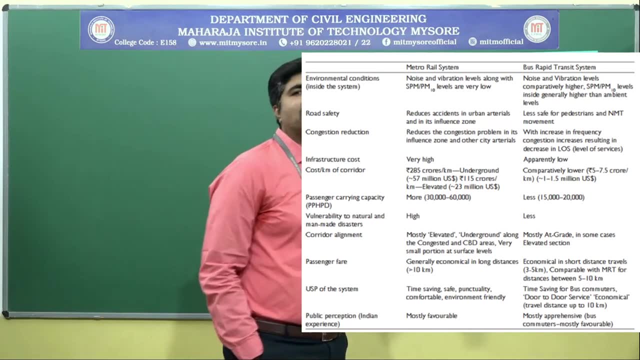 congestion here today. okay, in case of next transport infrastructure cost: okay. next transport infrastructure cost: okay. next transport infrastructure cost: okay, this requires high cost to this requires high cost to this requires high cost to provide the infrastructure: okay, that is provide the infrastructure. okay, that is provide the infrastructure. okay, that is there here. the for bus: okay, bus key and. 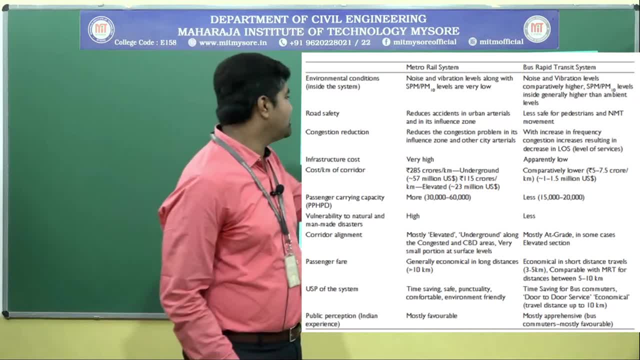 there the for bus: okay, bus key. and there the for bus- okay, bus key. and infrastructure problem are because the infrastructure problem are, because the infrastructure problem are, because the cost will be less. here it requests nearly cost will be less. here it requests nearly cost will be less. here it requests nearly 500 to 600 kilometer foot- sorry, 500. 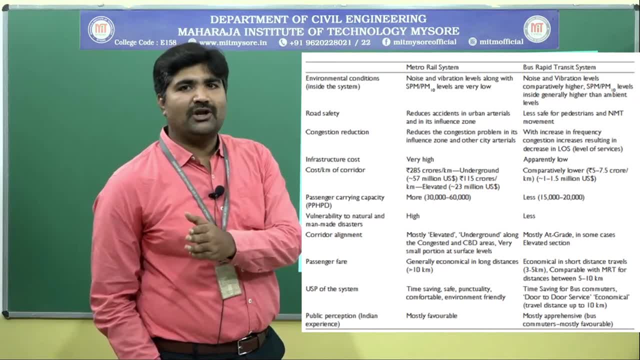 500 to 600 kilometer foot, sorry 500. 500 to 600 kilometer foot, sorry 500. quotes to 600: okay per kilometer, okay. in quotes to 600: okay per kilometer. okay in quotes to 600, okay per kilometer. okay in case of buses. it requests to 5 to 6. 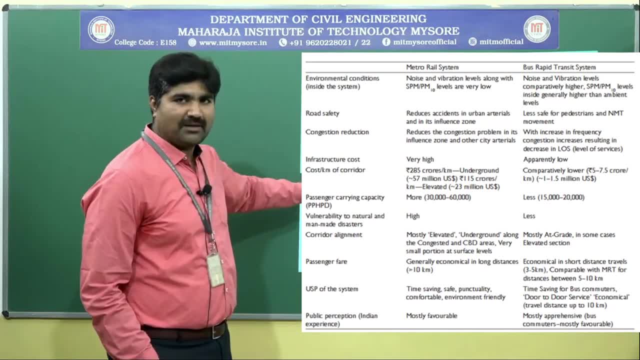 case of buses. it requests to 5 to 6 case of buses. it requests to 5 to 6 quotes: okay, per kilometer. okay. next quotes, okay per kilometer. okay. next quotes, okay per kilometer. okay next. passenger carrying capacity as we has. passenger carrying capacity as we has. 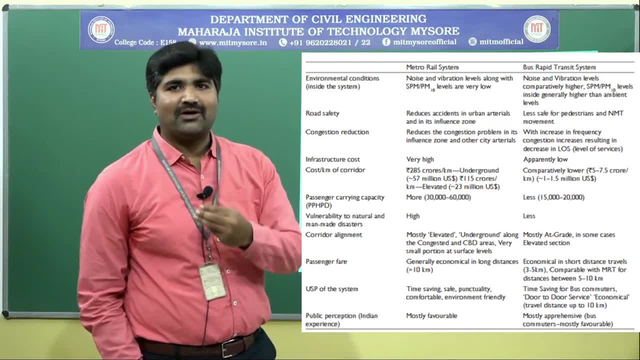 passenger carrying capacity, as we has discussed in the Metro. it has capacity of discussed in the Metro. it has capacity of discussed in the Metro. it has capacity of 1 lakh- okay, 1 lakh per hour it can carry. 1 lakh- okay, 1 lakh per hour it can carry. 1 lakh. okay, 1 lakh per hour it can carry, but it has a less capacity bus transit but it has a less capacity bus transit but it has a less capacity bus transit system around 10 to 15,000 per hour it system around 10 to 15,000 per hour it. 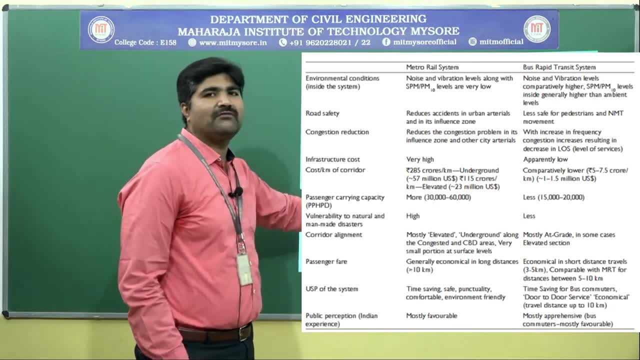 system around 10 to 15,000 per hour. it can carry okay, and next passenger fare can carry okay and next passenger fare can carry okay and next passenger fare passenger fare will be very less in case passenger fare will be very less in case passenger fare will be very less in case of Metro. that will be I. in case of bus.